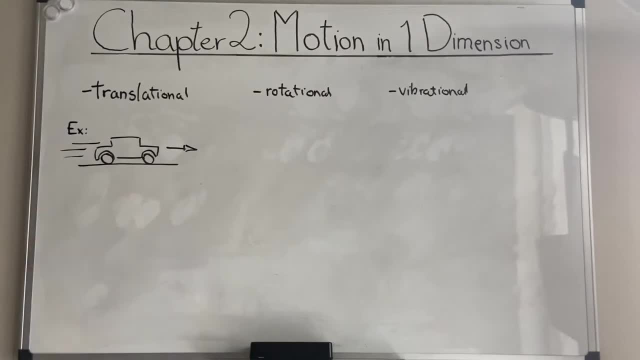 And there's a lot of different motions happening inside, But as a whole, if we just consider the car moving, it is a translational movement. right Now, rotational Rotational is a bit different. An example of rotational could be where the place where we all live. 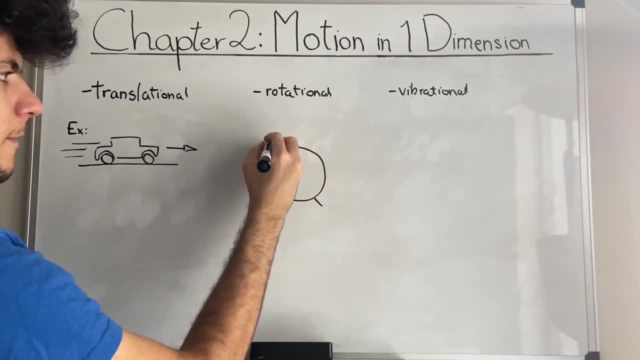 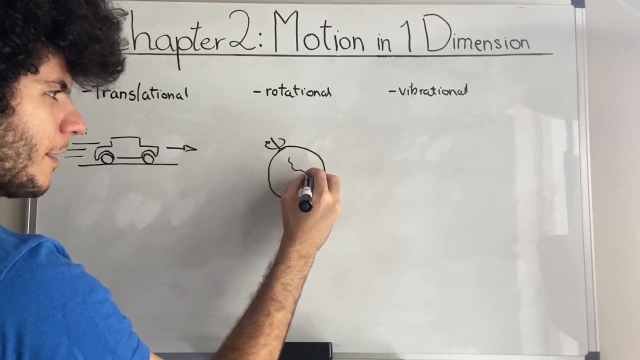 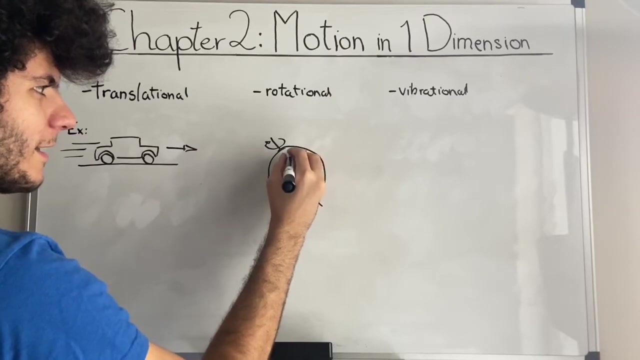 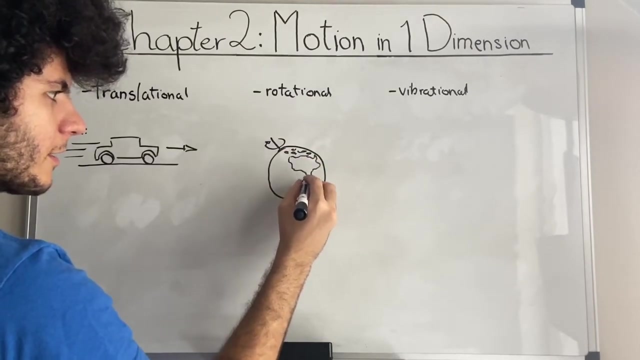 Earth. I guess I'm going to try and make like a America. oh, that's not very good, And there's little islands in the north of Canada, And then we have South America. I'm just going to make a blob. We have Australia, Russia. 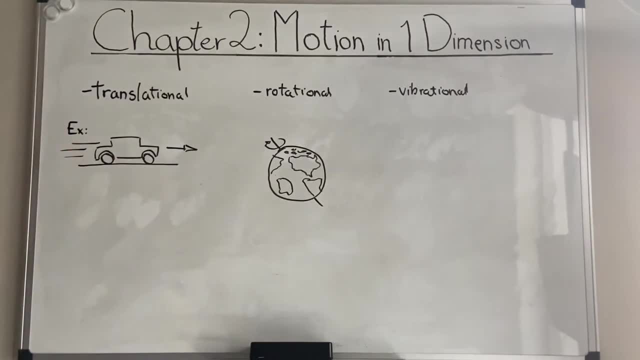 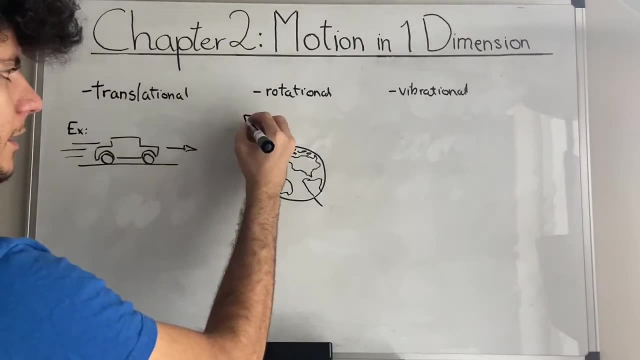 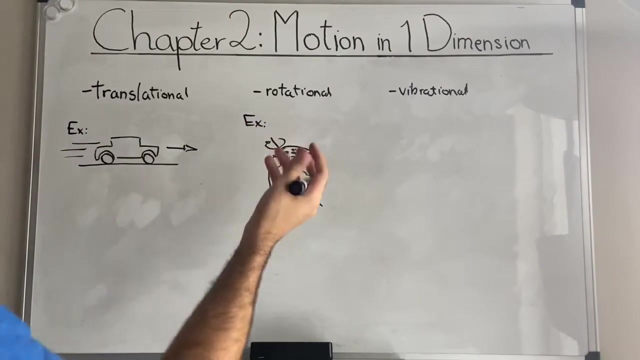 Okay, There we go. Our planet is actually rotating on itself. That's what makes us see. that's how we see the days and the nights. At some point of the day, we are facing the sun. At another point, we are not facing the sun. 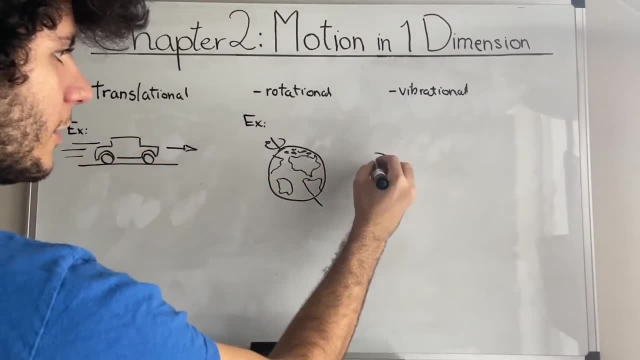 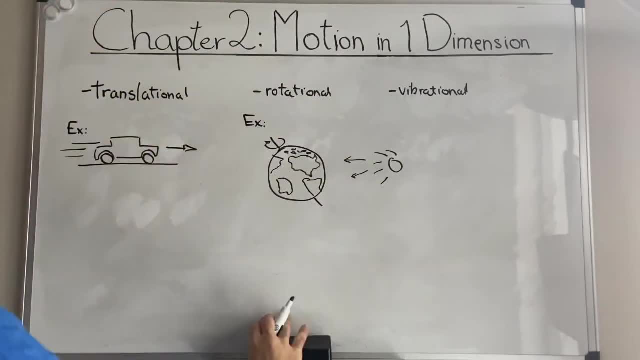 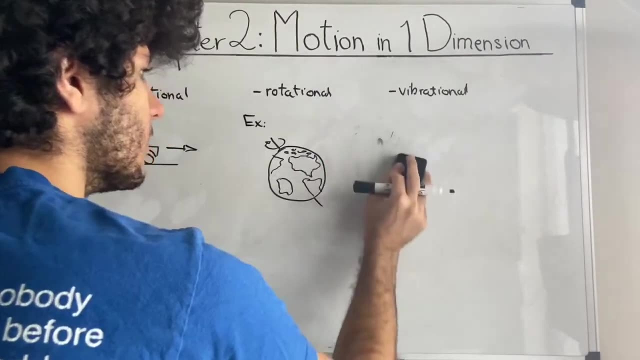 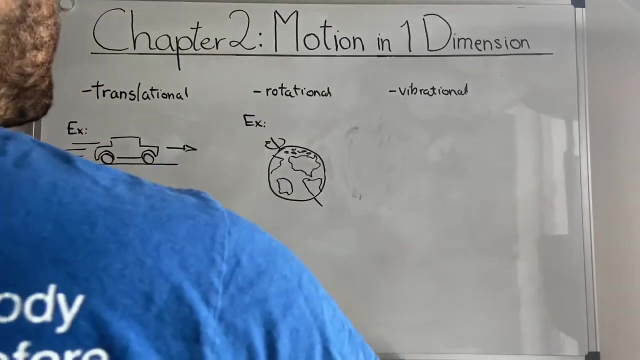 And that turning motion is what we call rotational motion. It's not a turning motion. Yeah, it's specifically a rotational motion. Oh, what's going on here? It's all right, I'll fix that later. And finally we have vibrational. 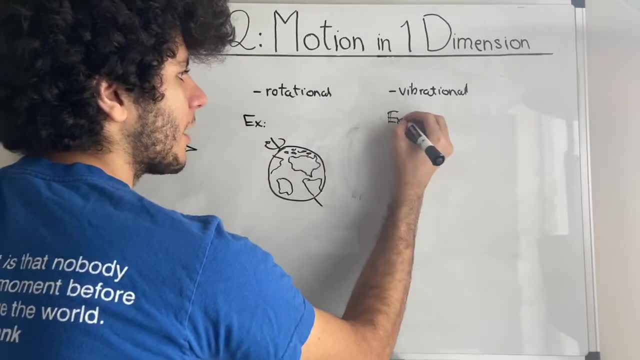 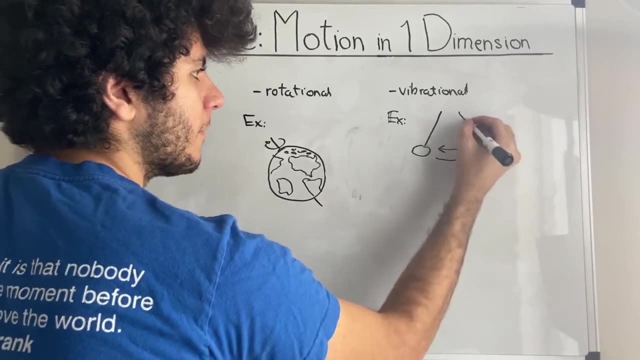 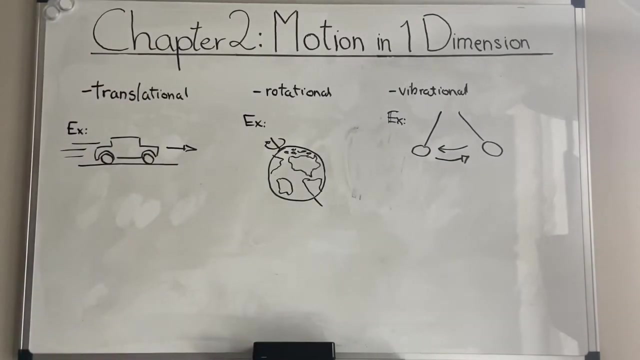 This might be a little bit counterintuitive, but a good example of a vibrational movement. This might be a little bit counterintuitive, but a good example of a vibrational movement Is a pendulum moving back and forth. It's heading, it's movement, it's back and forth movement is what we call a vibration. 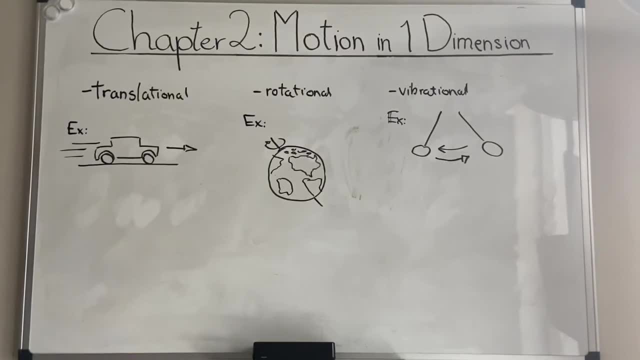 Right, And in this and the next few chapters we will only be considering translational motion, Only this one. Later on in the course you're definitely going to see that We're going to work with rotational movement and we're actually going to work with vibrational as well. 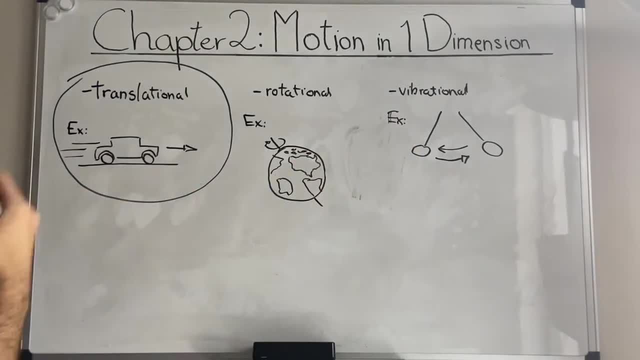 I have these pendulums. I wouldn't necessarily be. Yeah, I mean, I guess we're going to sometimes discuss vibrational movement, but we're mainly going to deal with translational and rotational movement motion in this class. But for now we will only be talking about translation. 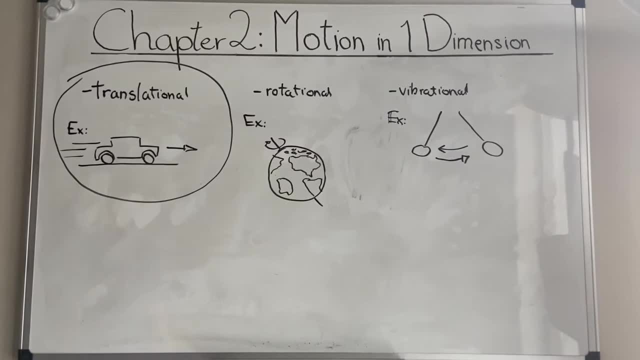 In our study of translational motion, we will use what is called the particle model And describe The moving object is a particle, regardless of its size. So, even though this is a car, we're just going to say that it's a point and it's heading in this direction. 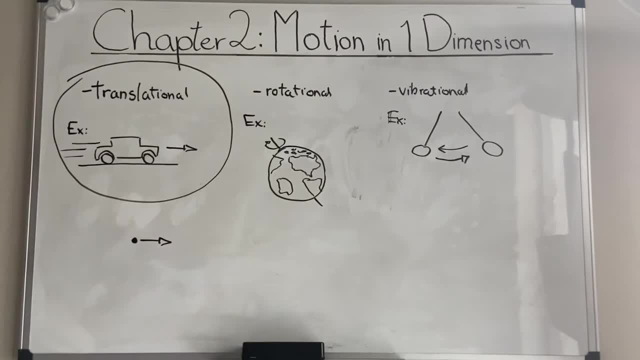 Not only will that simplify things, but, yeah, it will basically simplify things, and it'll help us avoid considering a lot of details that would make physics very difficult to warm up to. We need to start somewhere, And so a particle is like a. 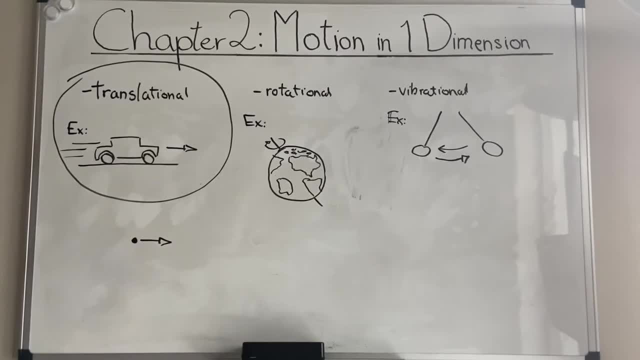 A point like object, that is, an object that has a mass but is of infinite, infinitely, infinitesimal size. I always mess up that word, So it's extremely small, but it does have a mess, And that's what we're going to work with for the next few chapters. 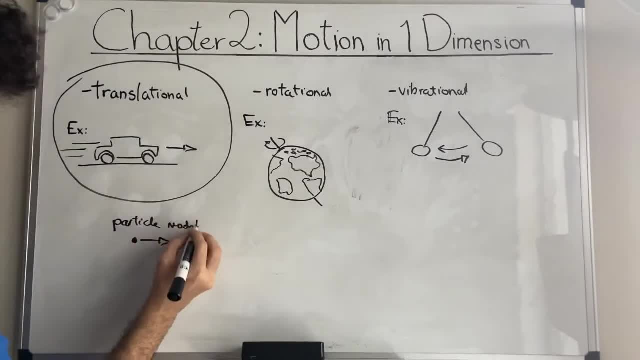 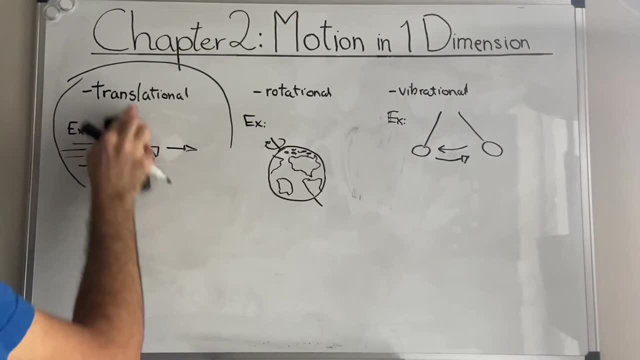 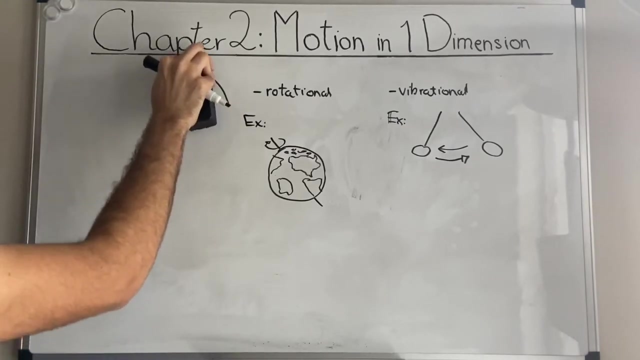 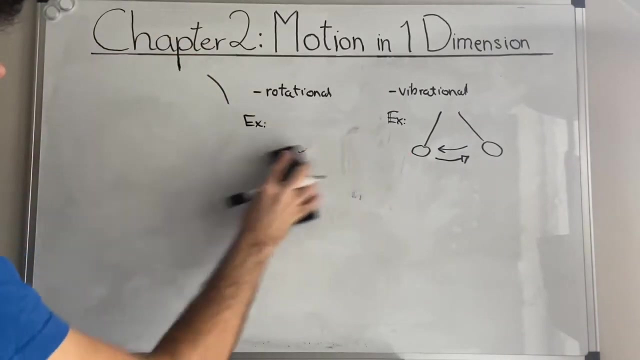 And we're going to call that the particle model Right. All right, That's great. Next we will begin to discuss position. What is position? Well, it's basically where something is at a given moment in time, And this will be the basis for so much to come in our class. 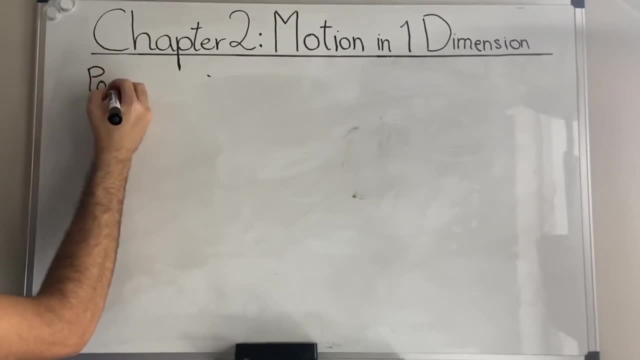 Position, Position, Very, very basic and fundamental. That's the whole notion. I need to take a sip of water, All right. So When we study the motion of an object, the most important quantity is the position of the object. 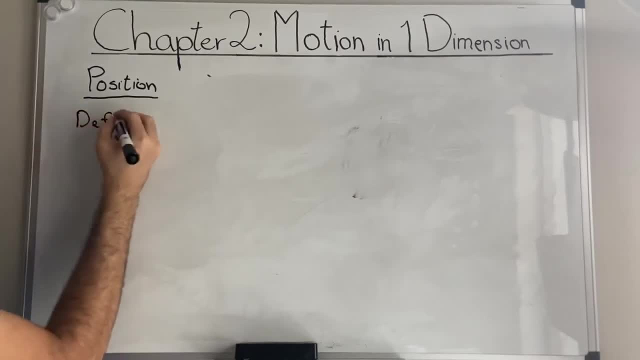 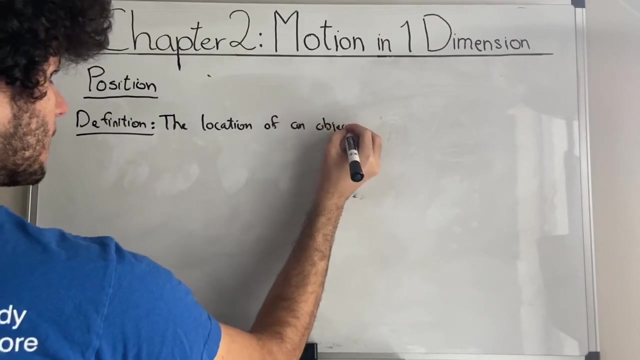 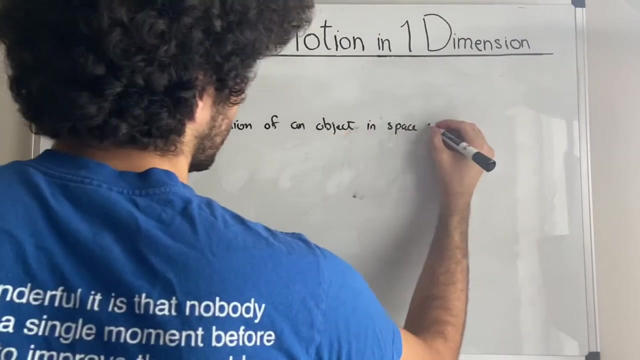 And we can. let's define this actually The definition Of position that we'll be using, And we won't need to define it a lot. This is just A way to pinpoint what it is exactly is the location of an object in space with respect to a coordinate system. 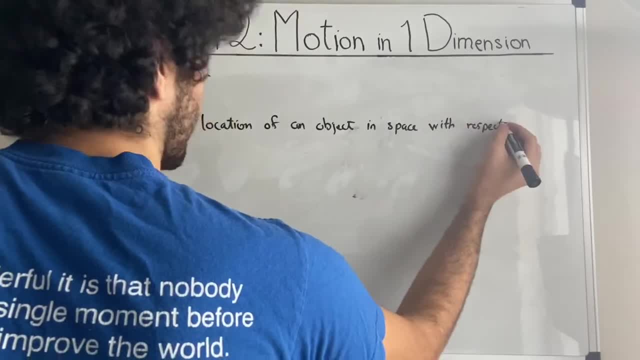 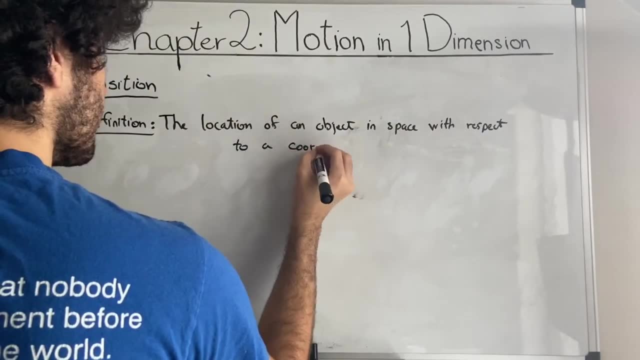 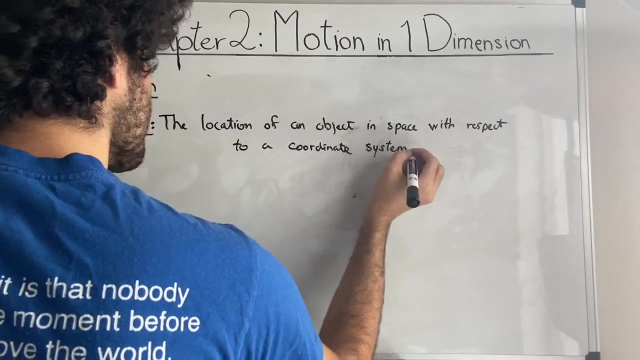 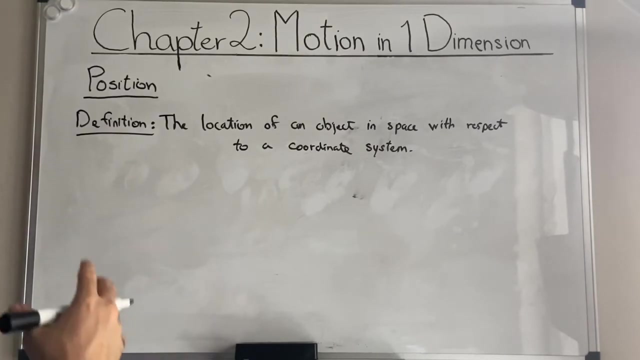 And that last bit is very important. Actually, all of it's important, But let's not forget that last part. Okay, With respect to a coordinate system, All right, So Let's start things off by defining. We've started things off by just defining it. 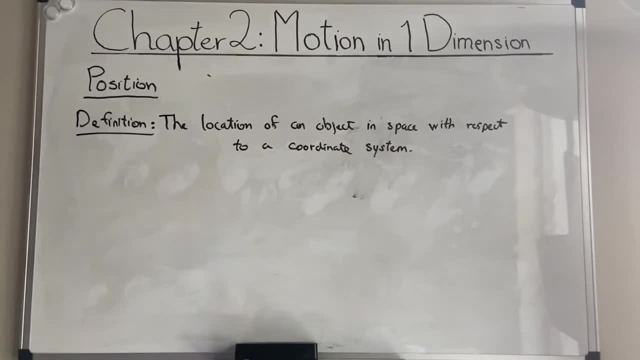 The location of an object in space with respect to a coordinate system. Note that we're working in one dimension, So An example of Such A scenario, of like, an example that can help us picture this is, like I said before, same example that I gave for the for the translational notion. 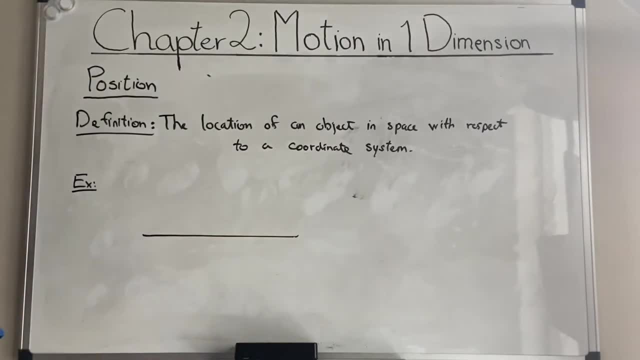 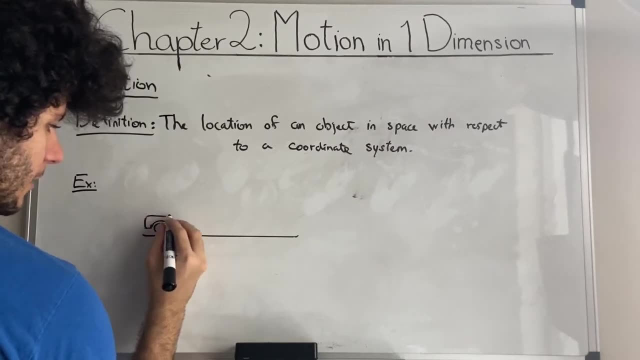 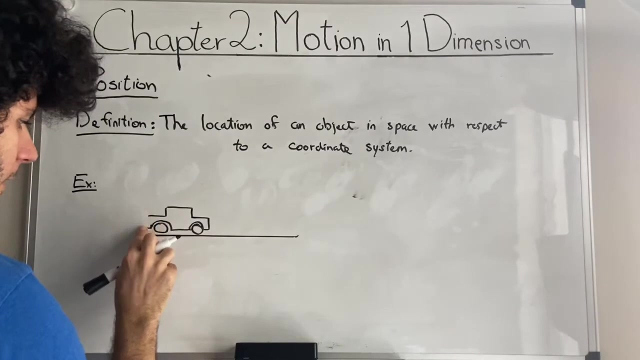 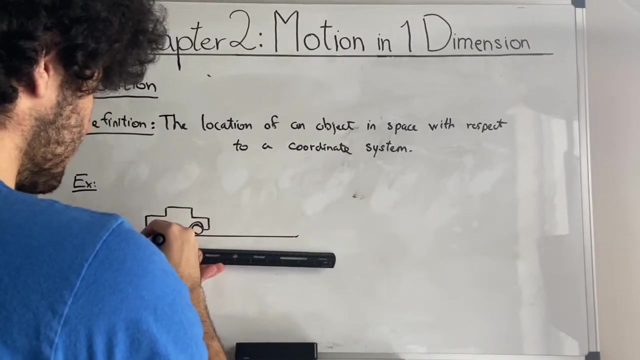 It's just a car driving down the highway. Thanks, Do quick little trying So we can have these seeds a car, All right, So we have a car and we're actually going to measure it. So it's on a coordinate system, right. 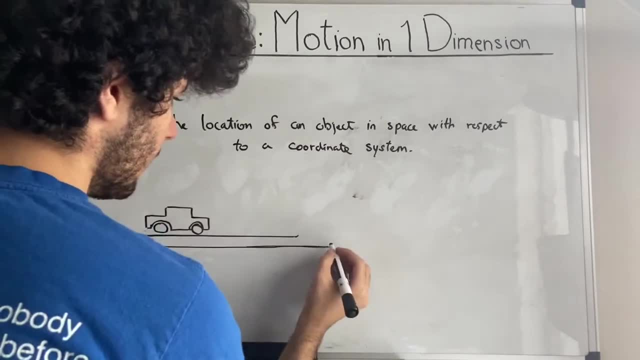 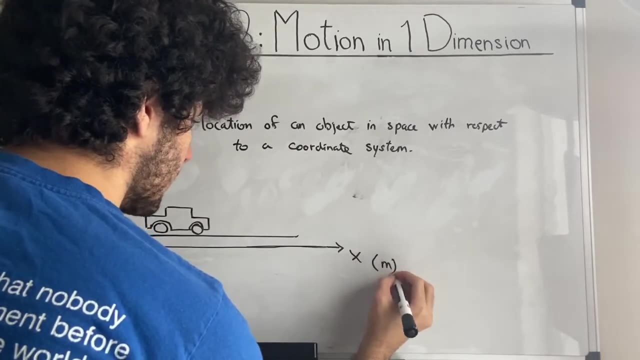 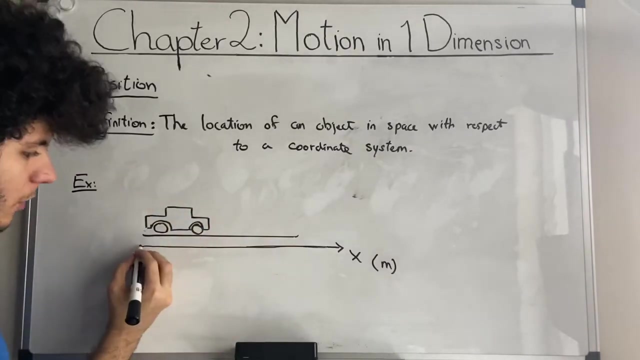 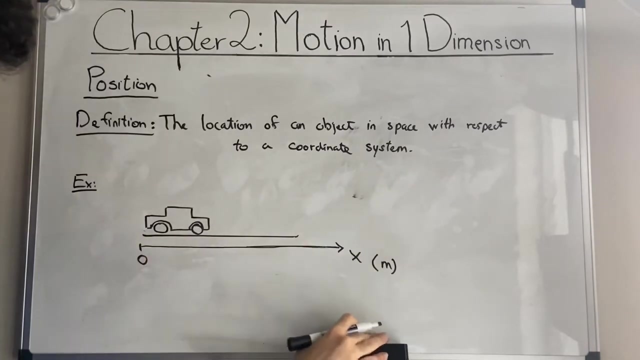 And we're working in one dimension. So we will be working with the X axis And that X axis will be measuring how many meters it's traveled, or not actually how many meters it's traveled, Just how many meters away from the Initial, from our zero, it is in its travels, however fast, however slow it might be going. 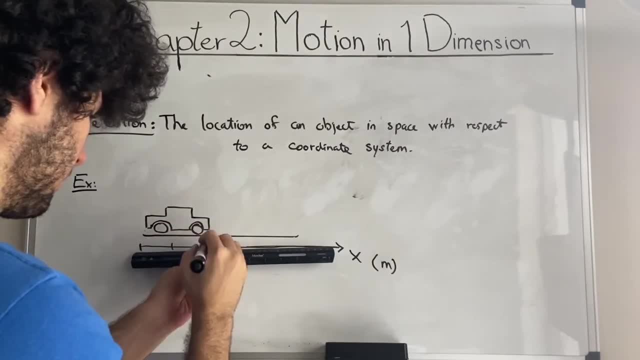 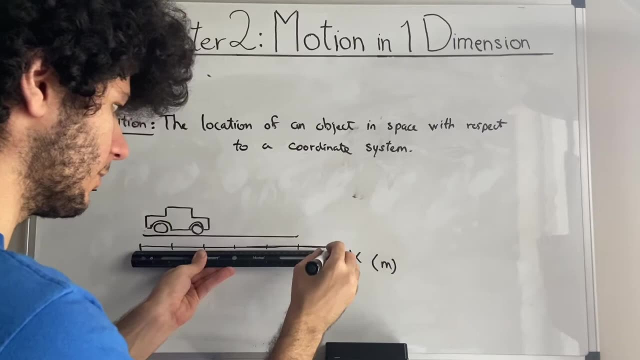 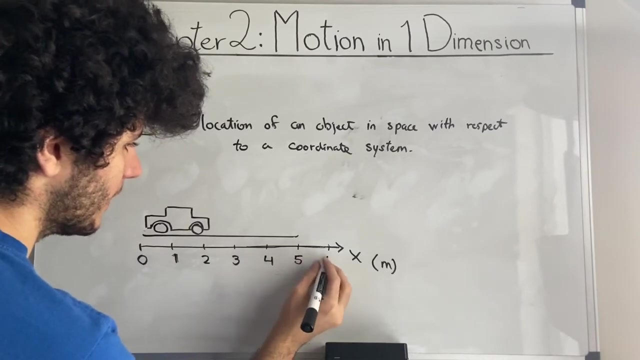 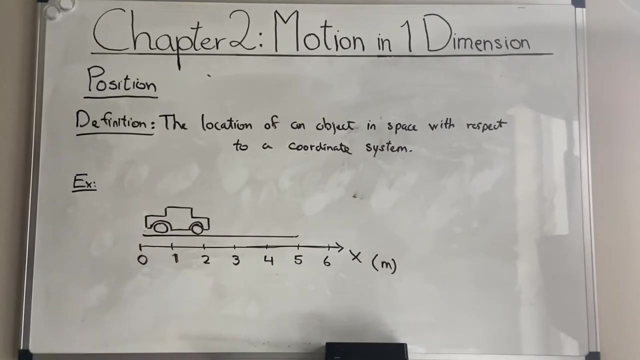 So let's set A few Different milestones along this Measurement, This instrument. We got one, two, three, Four, five and six, All right. So if we consider this to be, X equals zero, And remember we're working with the particle model. 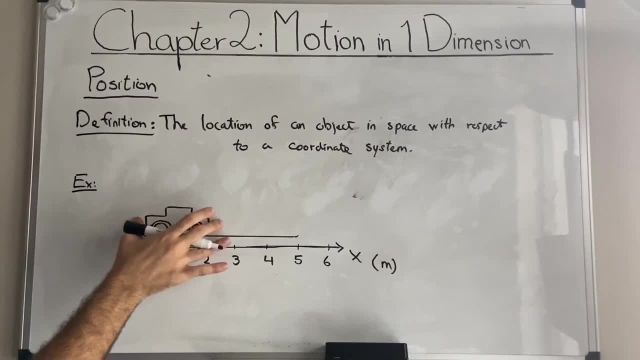 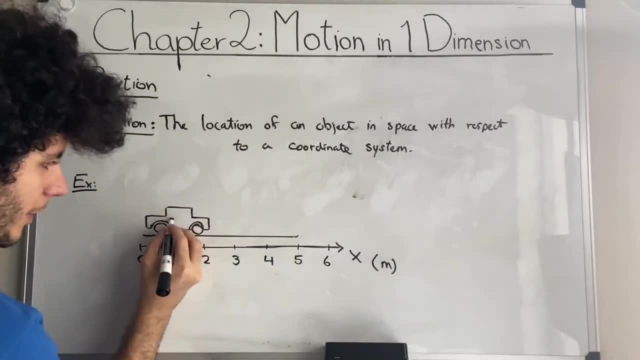 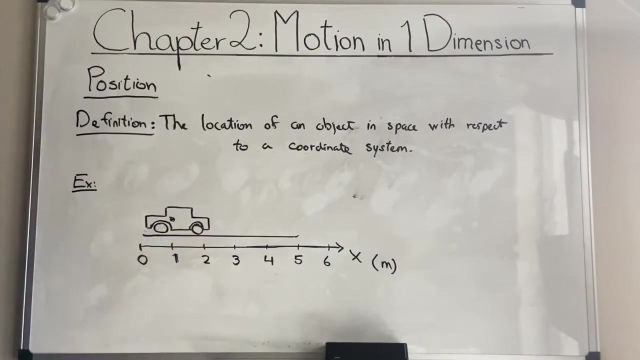 So basically this: though: I've drawn this car as a whole, we're going to try to summarize it with just a point, so that things are a little bit more digestible. So let's say, this is the point where it is. Well, in that case, ask yourself, where is? 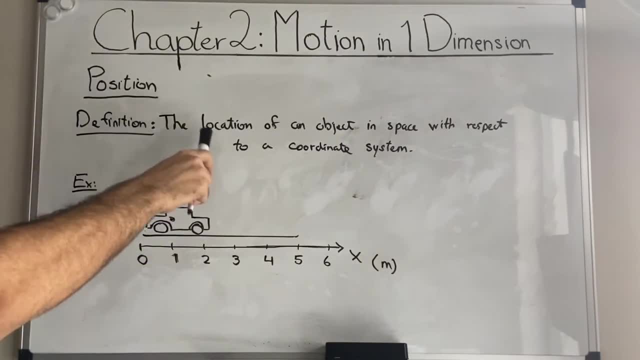 It along this line? What position does it have? What is? what is the location of the object with respect to the coordinate system? Well, if we consider this to be zero- X equals zero- then the car is actually at one meter away from the startup, from the zero zero. 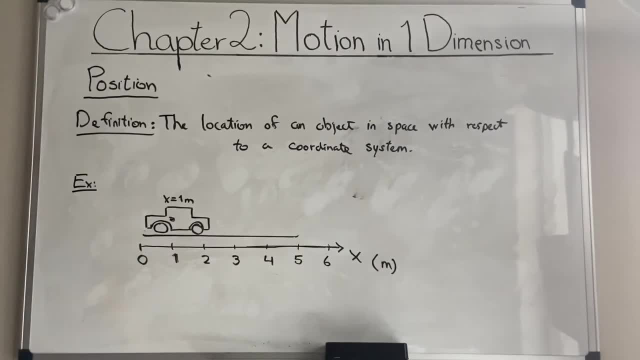 Well, in this case, just the zero, And that's. that's basically how we Under Determine the distance between two things. Let's say that there's like something else over here, like a ball. Well then, it's one meter away from the ball. 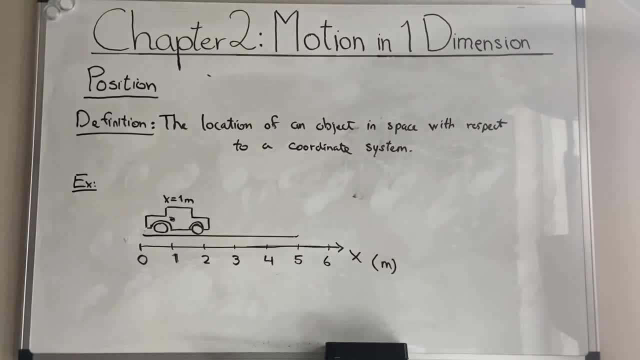 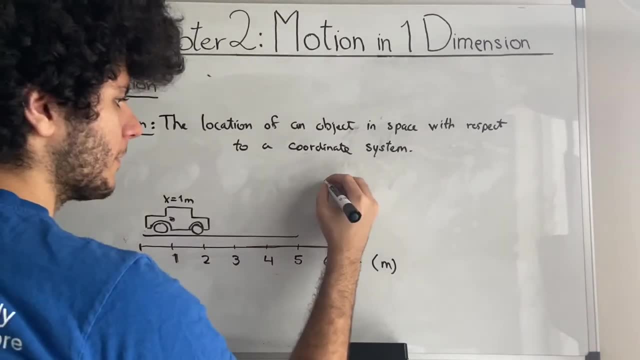 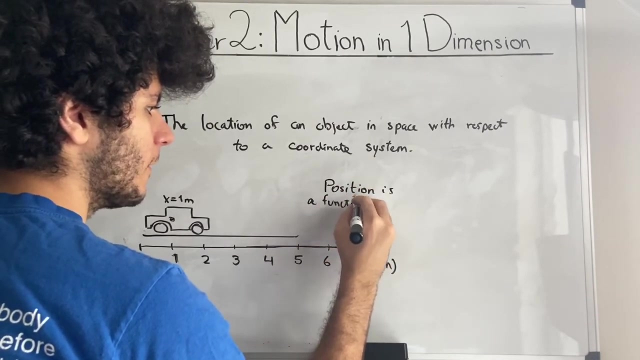 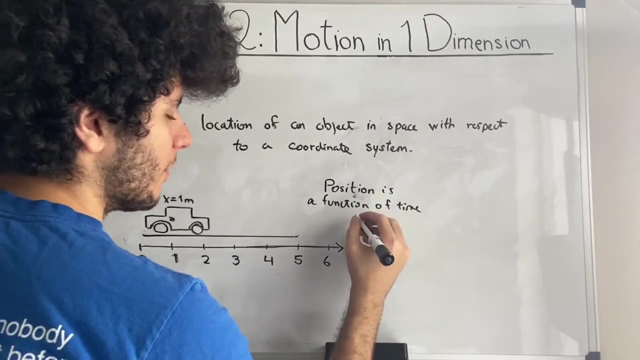 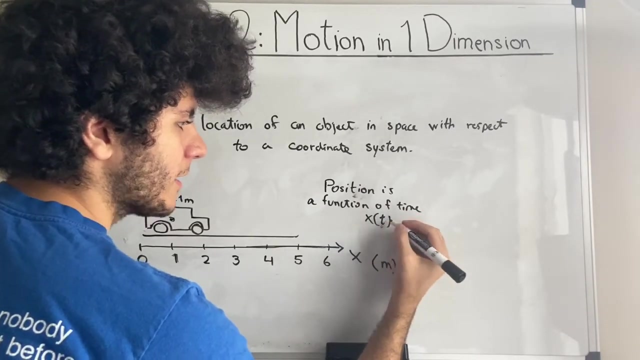 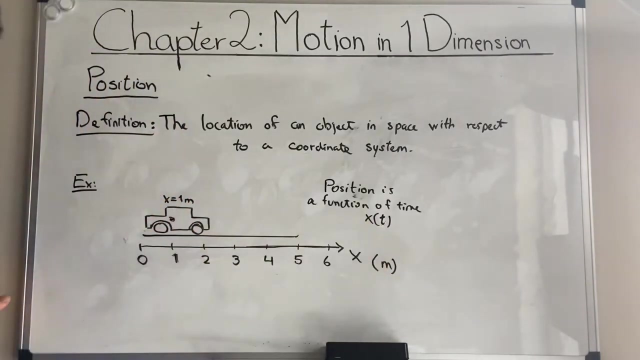 That's a little bit irrelevant. Another very important notion is that position is a function of time. right, Position is a function of Time, and we're actually going to be writing the function of position like this: X of T, where X is the position, as I've shown here, and T is the time that has elapsed- right. 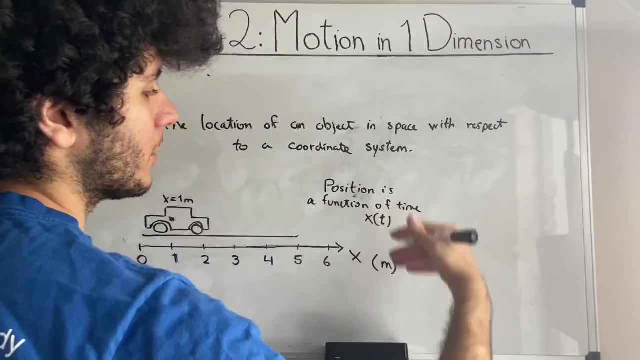 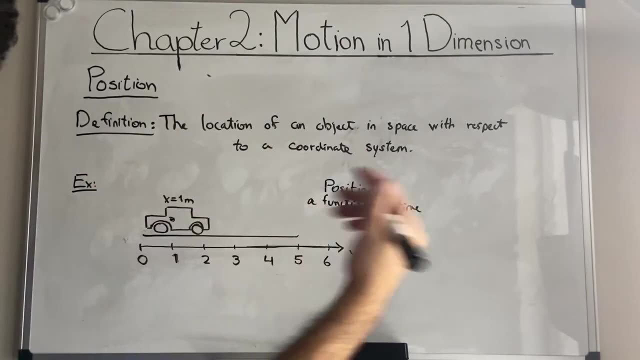 So at X, at T is equal to three, The car is likely going to be at a different location. At T is equal to seven, seven seconds. I suppose X is going to be another value, depending on wherever the car is in its travels. 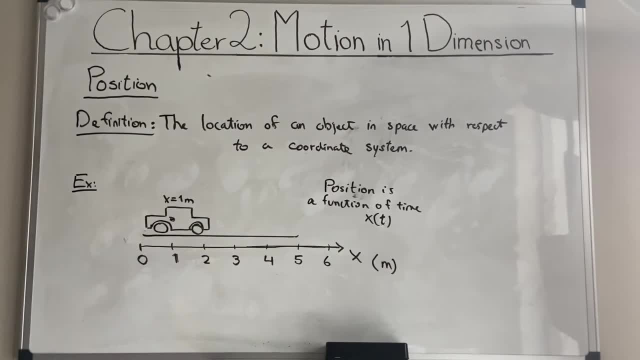 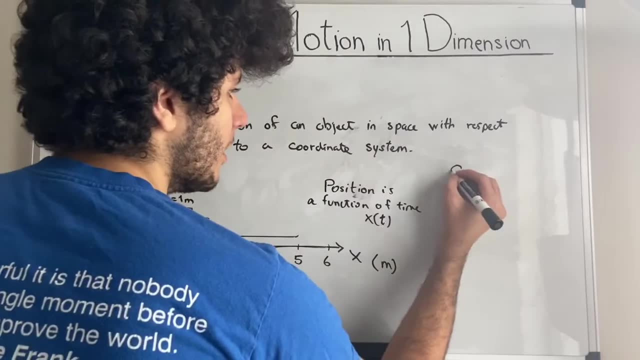 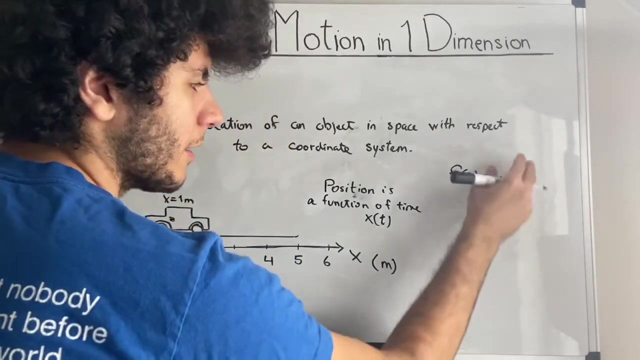 So, and let's note that plotting position versus time is useful, just as in math, when you were plotting F of X, you would consider: well, first of all, F of X altogether is equal to X. right, It's a Y. I'm sorry. 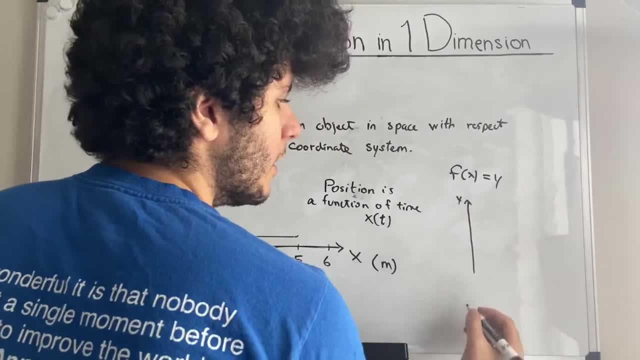 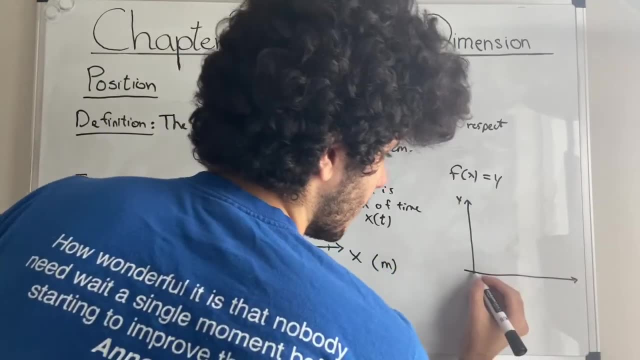 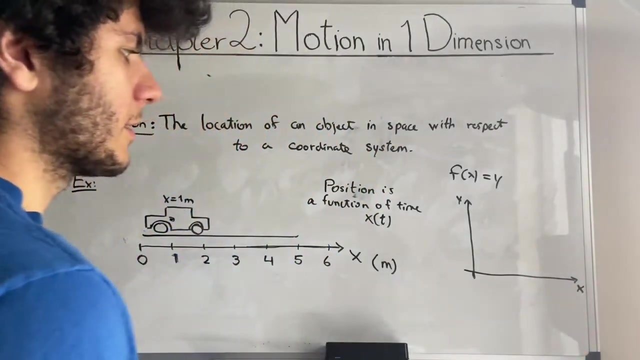 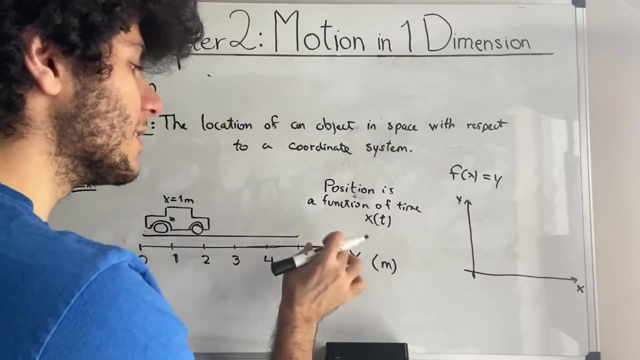 So that would be our vertical axis, and then X being the dependent variable. the independent variable, I'm sorry, would be the horizontal axis. Well, in this situation, time is independent of wherever the car is. The car, or at least the position of a car, is dependent on the time that has elapsed. 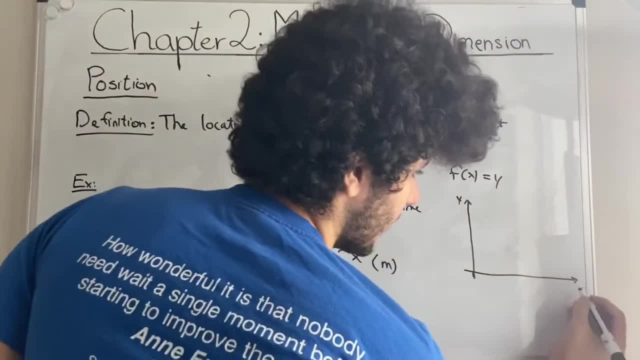 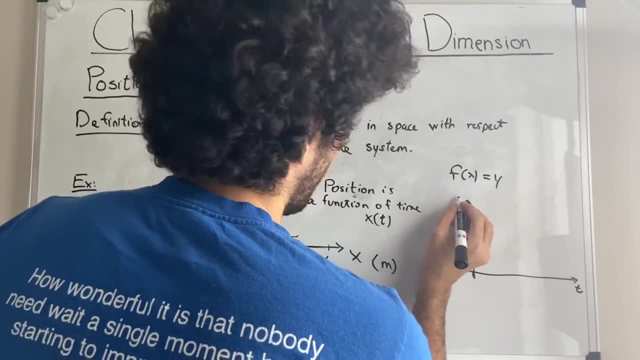 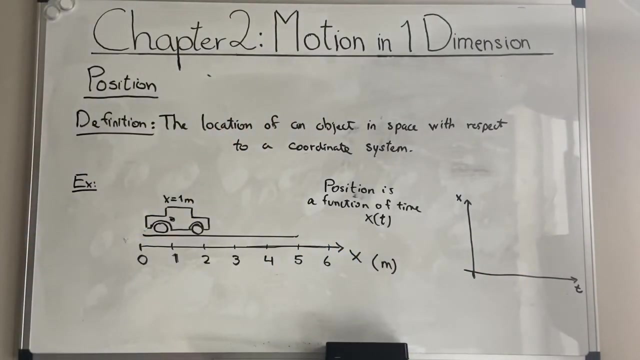 So it's going to change depending on what point in time we are. So, because of that, we will be using T as a horizontal axis and Y- not Y, I'm sorry- X- as our vertical axis. right, And before we go into that, one final point I forgot to make was that our coordinate system can be whatever we want it to be. 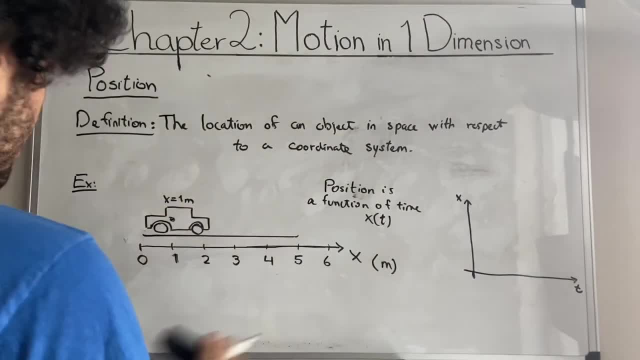 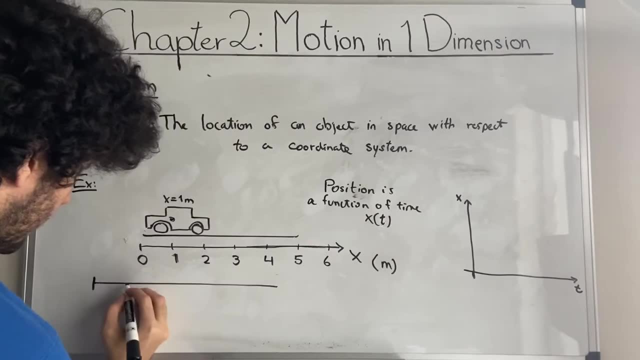 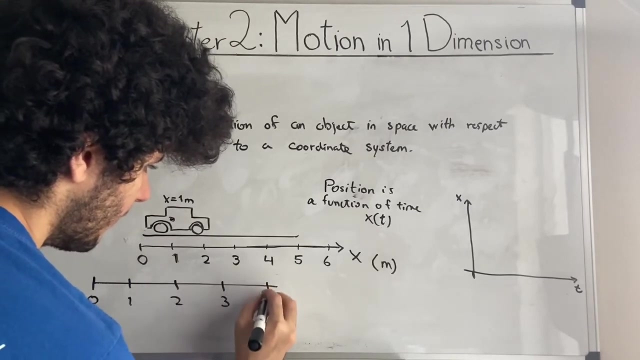 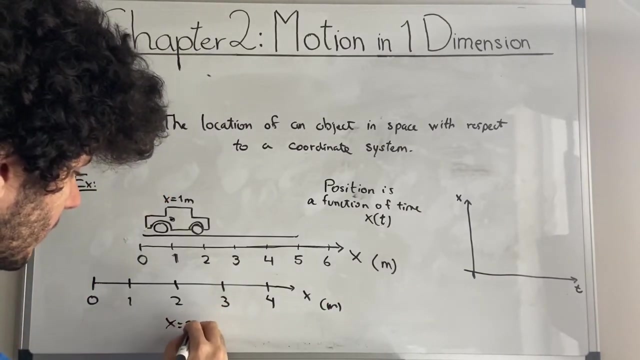 It doesn't need to be this exactly. We could create a new coordinate system where we have zero, one, two, three, four, And if you take a look at this coordinate system, X is actually equal to two meters, And so you see, everything is relative to the coordinate system. 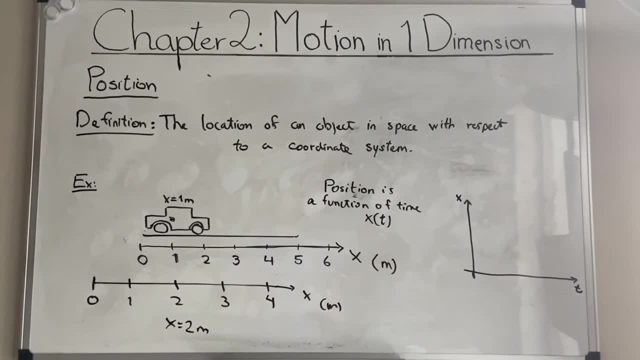 It depends on how, where we're like, what the axes are Of the situation. Oh, I'm on low power mode My phone. I'm filming this with my iPhone. Quick sip of water, Okay. So yeah, everything is relative to the coordinate system. 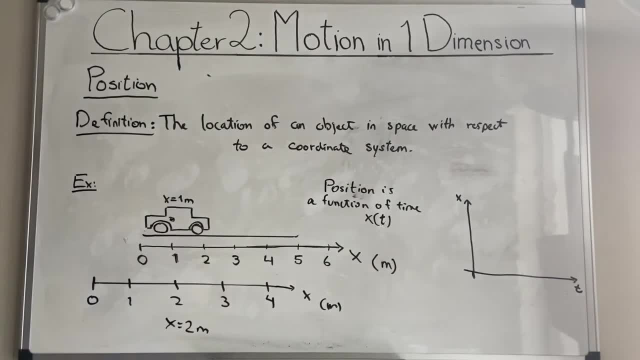 That's why establishing a coordinate system in physics problems is very important, just as it is important to define a system, For example. we need to have an understanding of the scenario, not just solve with the formulas by just plugging and chugging. 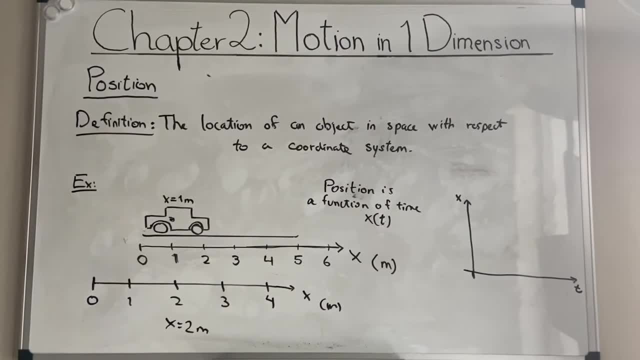 No, that's not how physics works. So, um, we are going to continue by discussing a little bit, finding out what we can use the position versus time graph for Right. I'm just going to plug in my iPhone. It's a little low on battery. 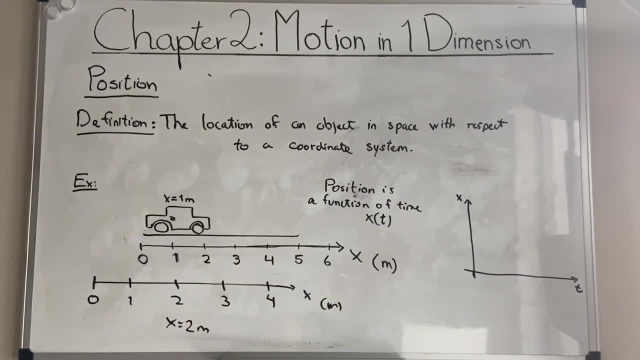 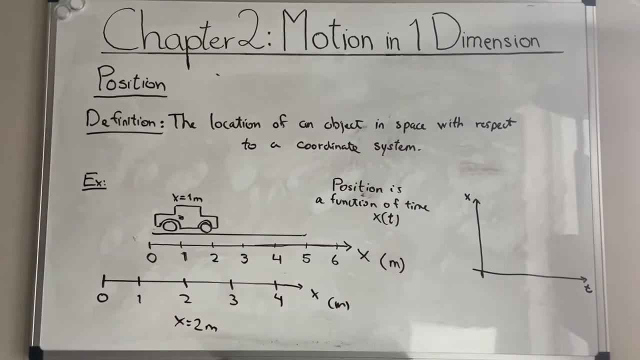 All right, There we go. Perfect. So the position versus time graph: right, We're all done with this. We can go ahead and erase what we have. We're still dealing with position. only We're going to be dealing with it. 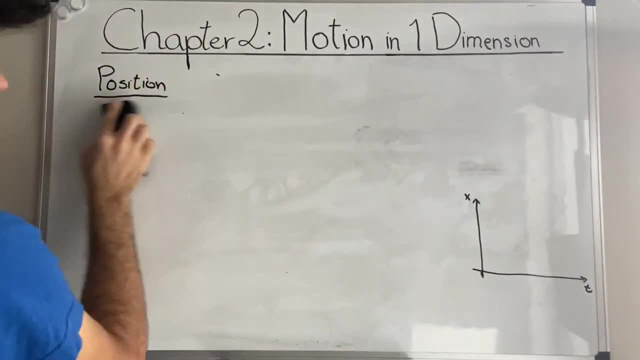 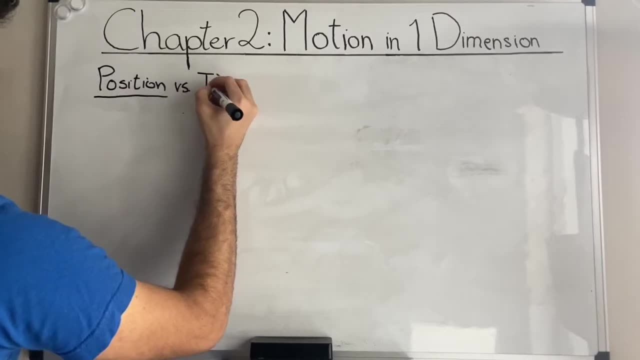 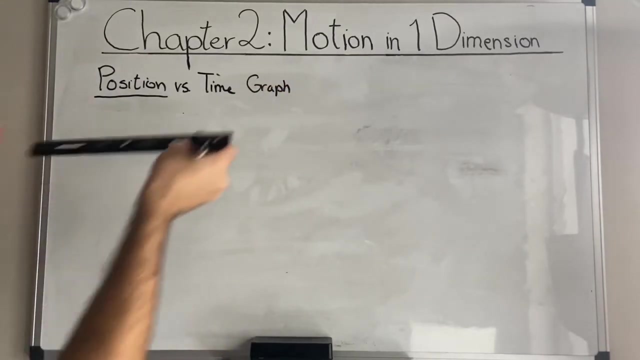 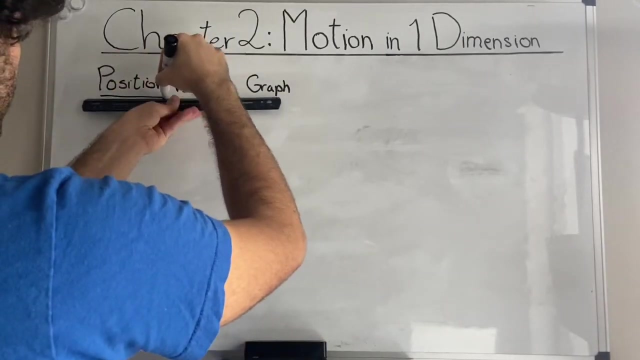 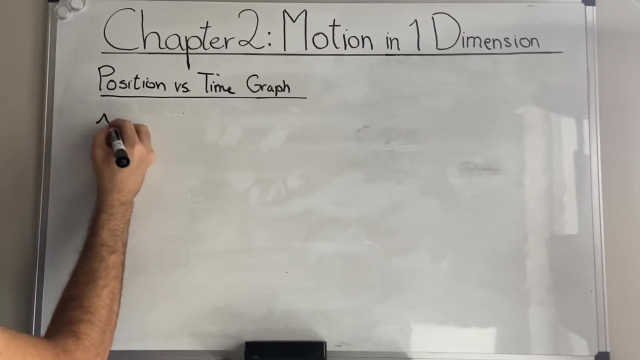 Dealing with its graph with respect to time Position versus time graph. right, We're going to use the graphs a lot in this class. This is only the beginning, All right, So let's go back and say if, wo have the following: 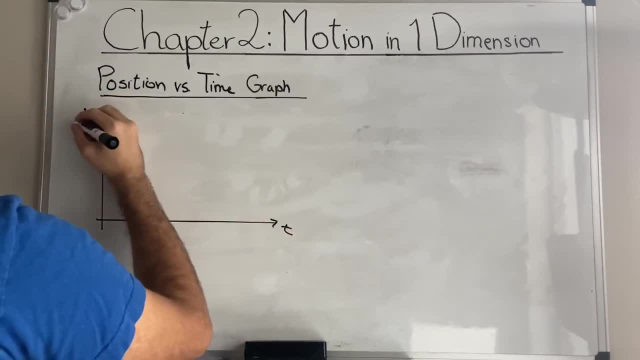 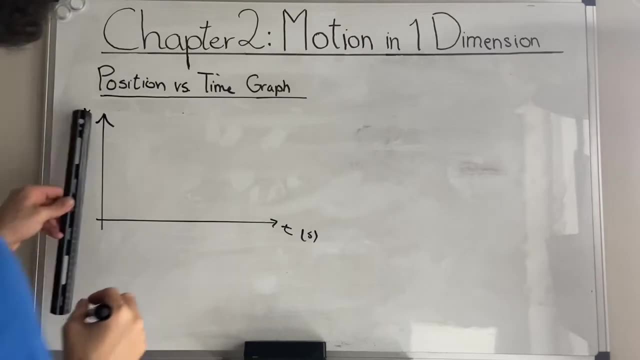 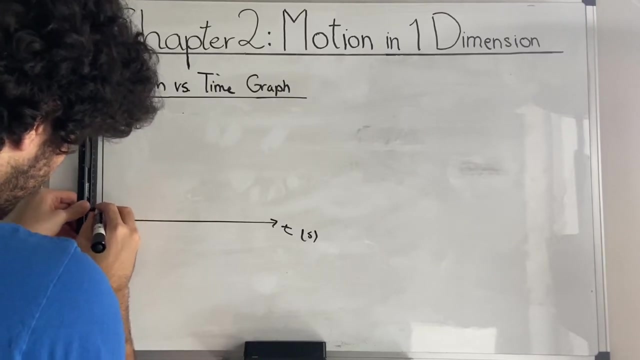 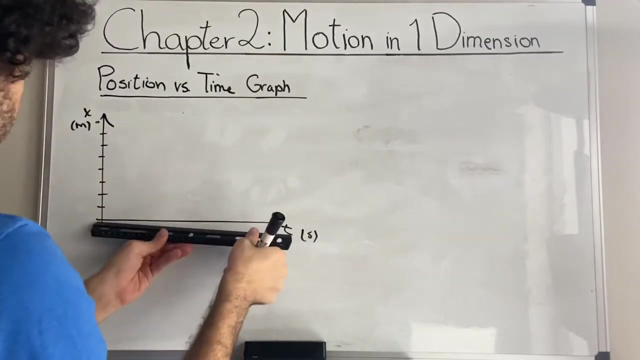 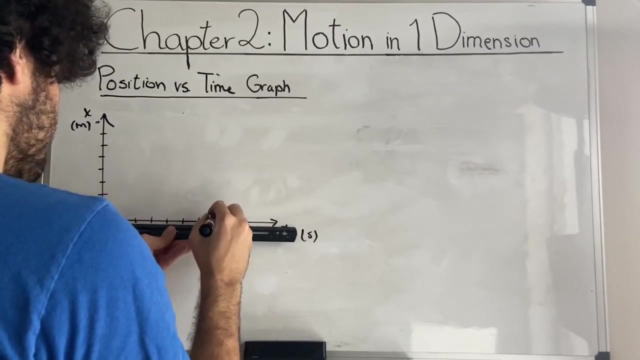 T. we have X- X is in meters, T is in seconds- and we have stems like this: Bang bang bang, bang, bang bang bang All right over here: One, two, three, four, five, six, seven, eight, nine, 10.. 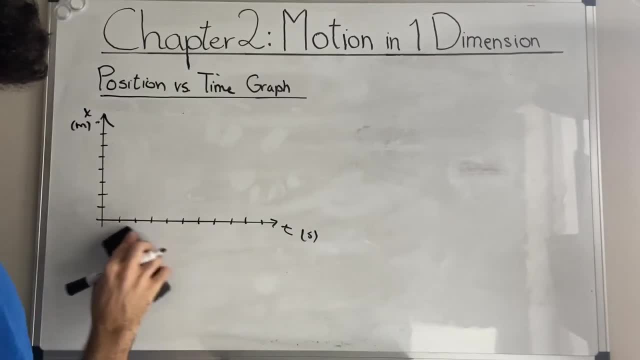 Two, let me do jumps. I'm gonna write all of these: Two, four, six, eight, 10.. Two, four, six- fantastic. So what if we had a graph like this and there was something plotted, only it was just a straight line? how odd. 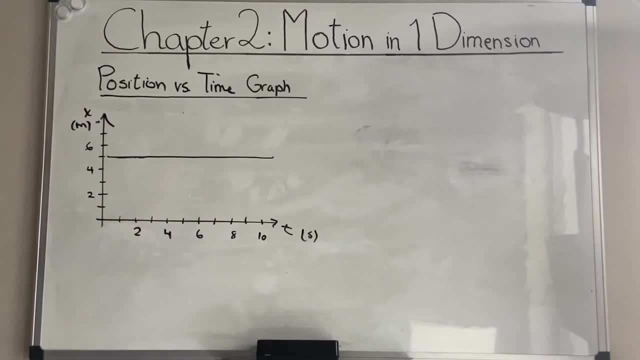 So what is this defining? What is this graph telling us? Where we see that the position of an object is defined over here, And as time changes, the object will move with respect to the coordinate system, right, So that coordinate system that we saw over there like this: 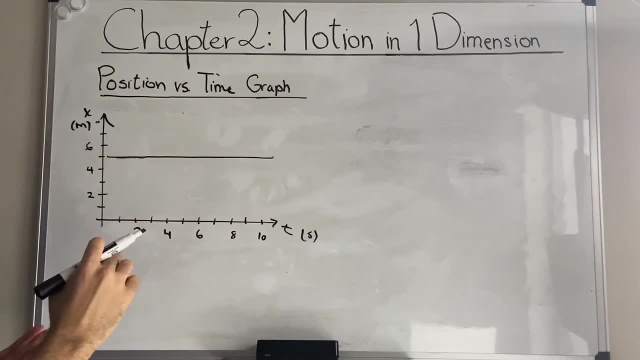 it's basically like this right now, And the car will change its position depending on what point in time we are. So in this situation, its position is: X equals five. Let me write that over here: X is equal to five meters. 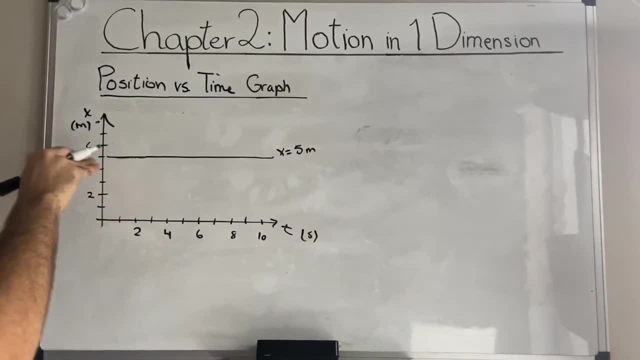 And the thing is that it's always X equals five. What this means is say: this is a car, it is stationary, it's not moving, It's at X equals five, permanently It's not going to move. As you see, with time, nothing changes. 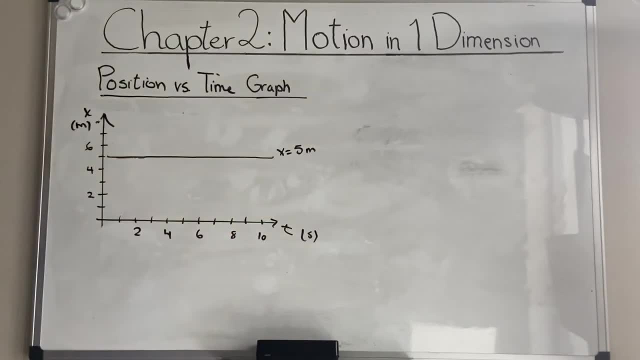 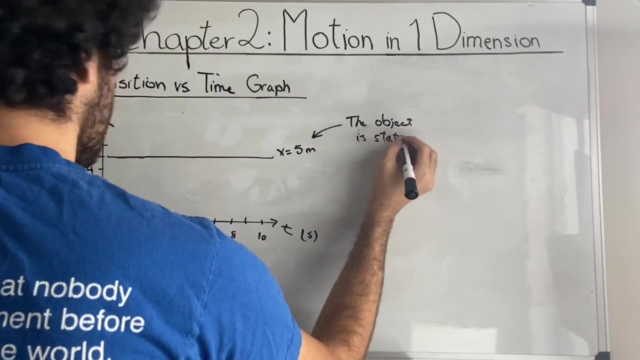 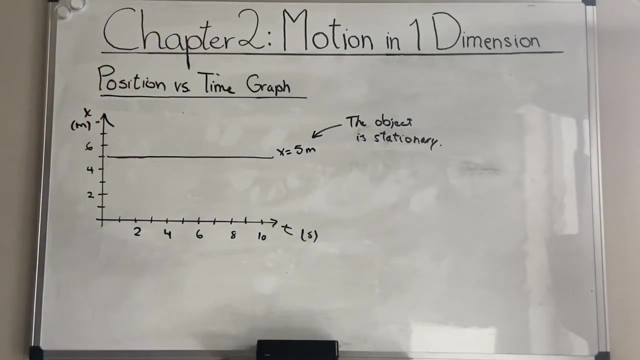 So basically, it's a car that's just in a parking lot, not moving, nothing to see here. So a way that we can say that is the object is stationary- Stationary, right. Okay. now we're gonna have a few different types. 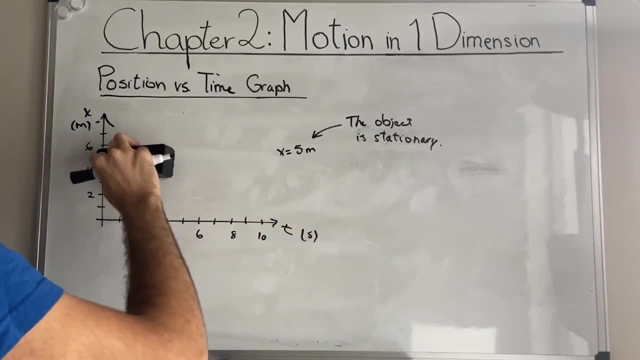 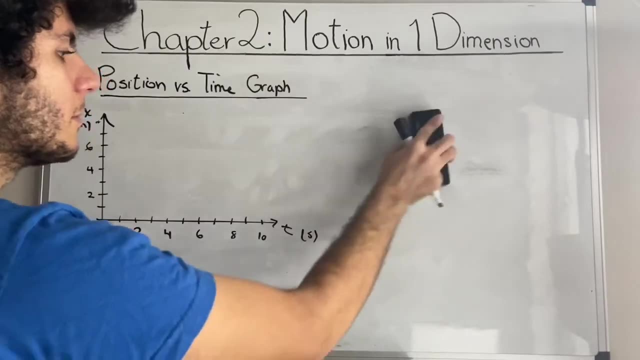 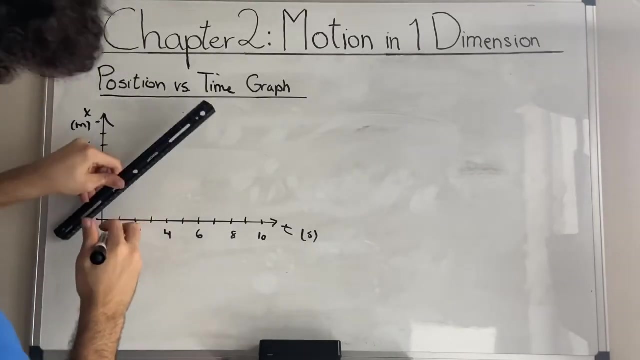 of scenarios, though. when we are working with time position versus time graphs, It's not always going to be as simple as that. Sometimes, we're gonna have things like this, And I'm gonna start it from zero. zero, just for the sake of it. 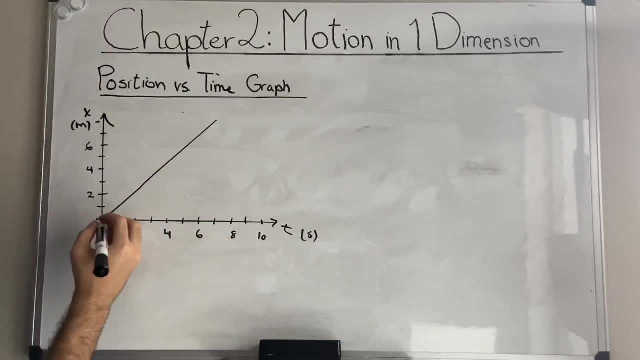 But sometimes it could start at different. at other points Say we have this. what does this mean? Well, if you take a look, the object started at X equals five. It's at X equals zero meters, and gradually goes all the way. 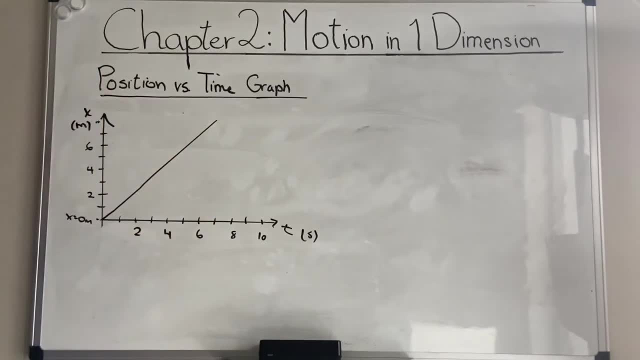 up to like eight meters away from where it started. Huh, okay. And it moves as time changes, right, As time changes, it moves in the positive X direction. right, And we could have. this could have been, we could have defined this coordinate system differently. 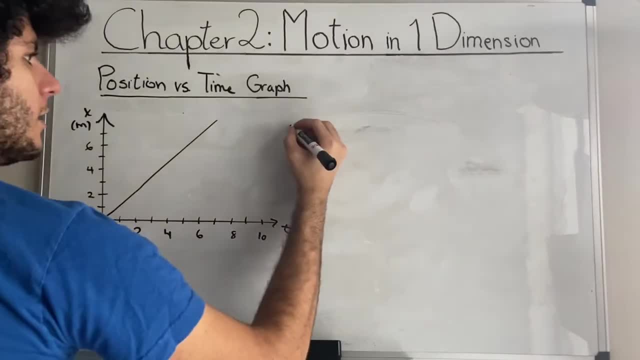 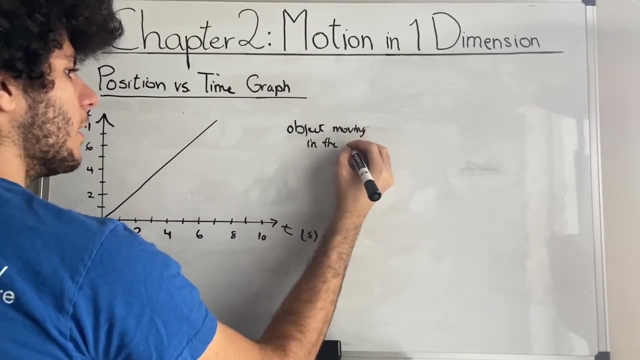 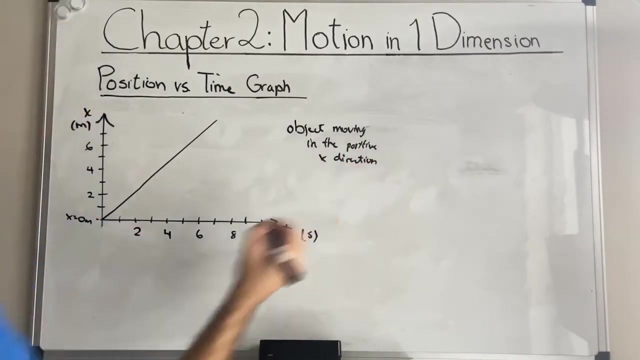 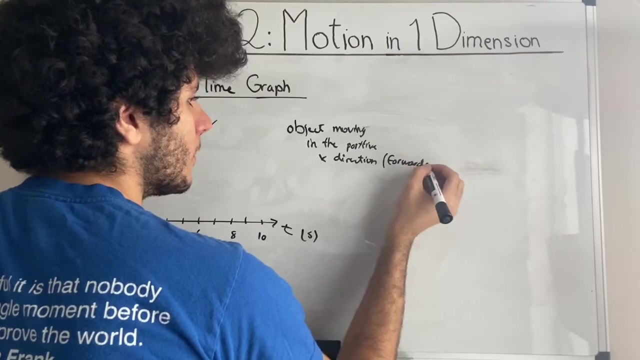 But in this scenario, this is, this is a coordinate system. So we have a coordinate system. So we have a coordinate system here, basically, the object moving in the positive X direction, all right, and this is what we could call forwards, and it's all relative to the coordinate system. 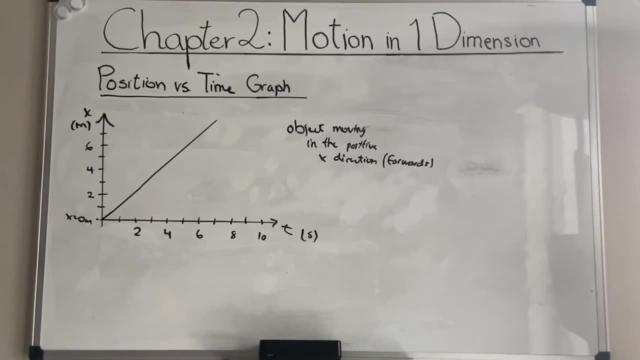 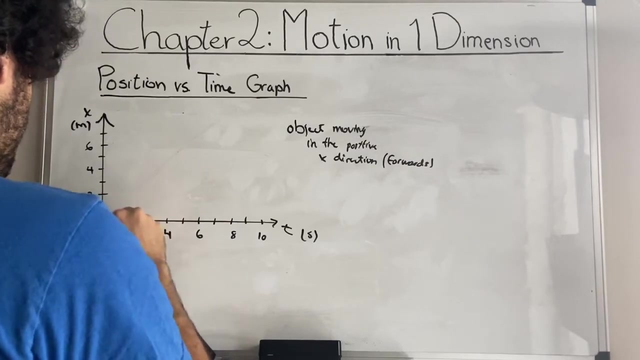 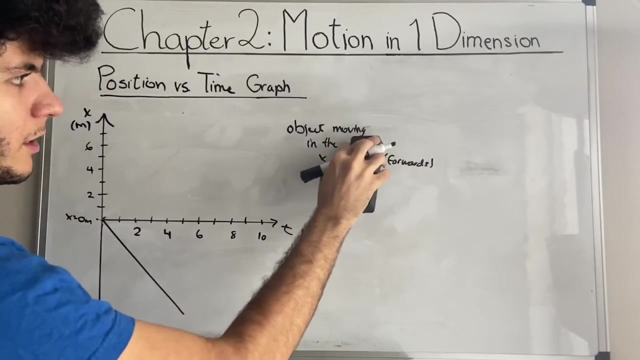 this could be a very different coordinate system and we'd have a very different understanding of what's going on. so another type of situation now we will often see is where the graph is going down and in this situation we- the object- will be moving in the negative X direction. 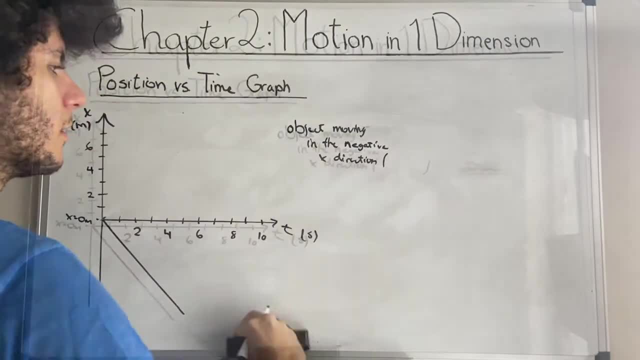 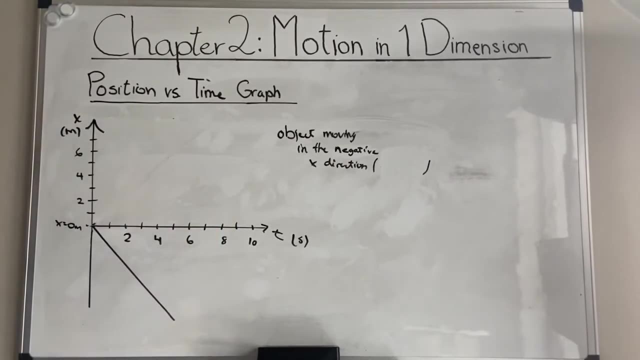 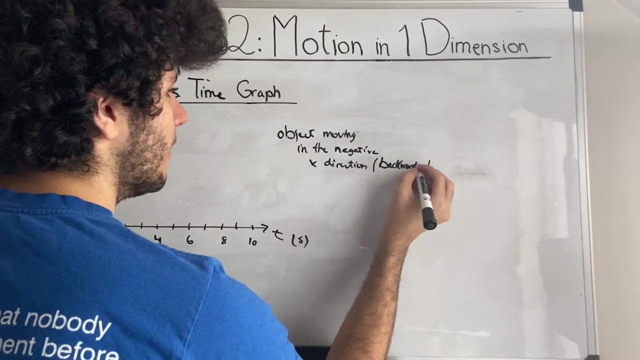 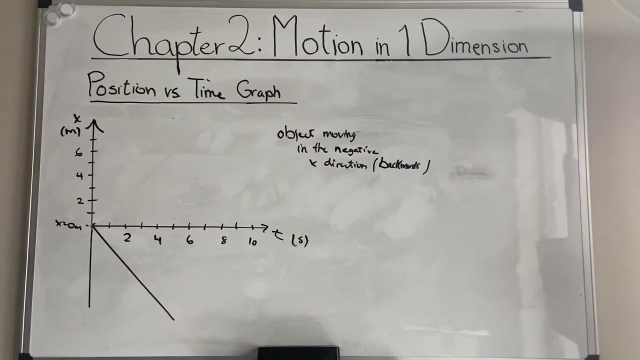 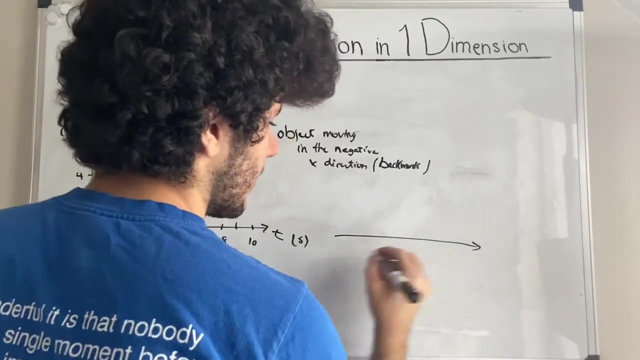 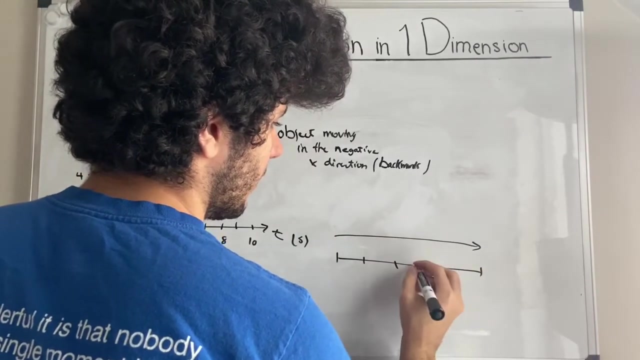 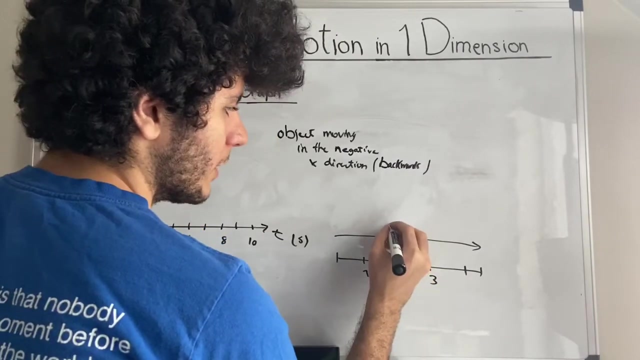 which is backwards, sorry about that which we will call backwards. so basically, um, in this situation the object is moving in the negative X direction. so if we had like a timeline over here, not a timeline but a measurement of distance, one, two, three, if the point was over here, if an object was over here, 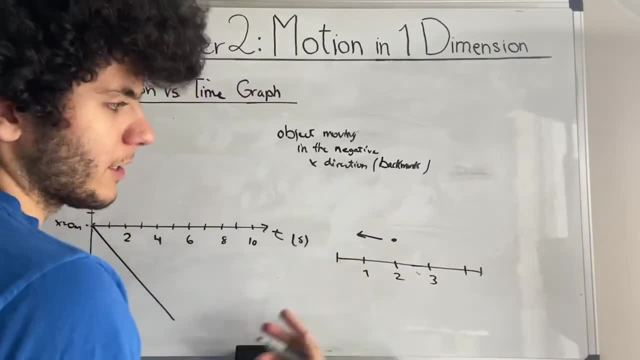 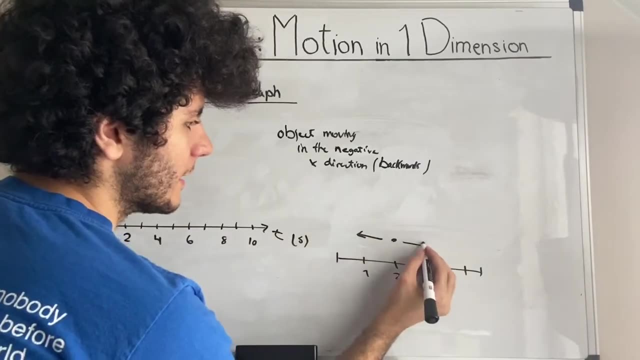 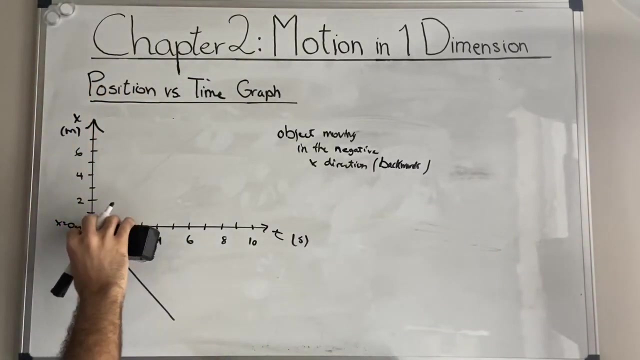 then it would be going in this direction, since that is the negative, the negative direction for this coordinate system moving forwards. is this direction right? so it all depends on how we define the coordinate system. okay. next we have a more complicated situation. all right, this looks very scary and we need to understand what is going on. 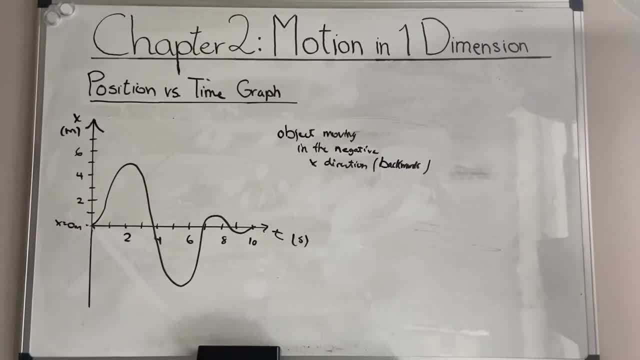 almost exactly what's going on here. this one is really a very strong constraint. so, basically, if we use what we understood in the last, what we learned in the last few minutes, this: since it's going upwards, since the slope is positive up until this moment the object is heading in the positive x direction. 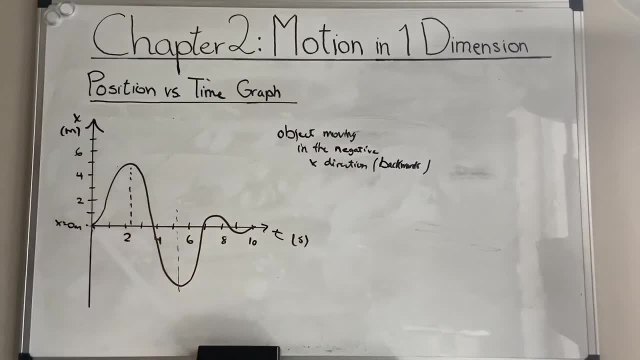 then, from this to point on to this point that we want as well, will be heading in the negative x-direction. and note that this, the crossing of this point, is just a return to the original startup point, since we start at zero. it doesn't mean anything, not much more than that. this is just a 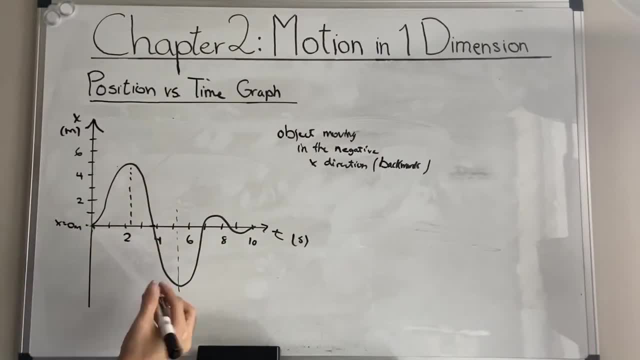 downward: a a movement in a negative x-direction, followed by a movement in the positive x-direction over here and another move in a negative direction. so an example of like what's going on could maybe be: you're going to school, you head to school, school, and this is your home, zero is your home. and then you realize: 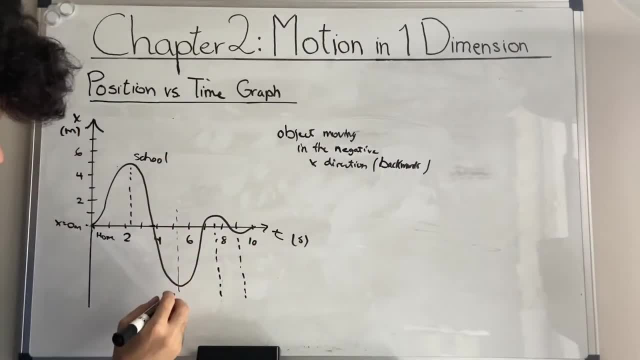 you forgot your backpack, so you head back home to- let's call this like negative, this is not home. you head, you go to- actually you're at home. you go to school and you realize you don't have any pencils. so I suppose it's weird of a. 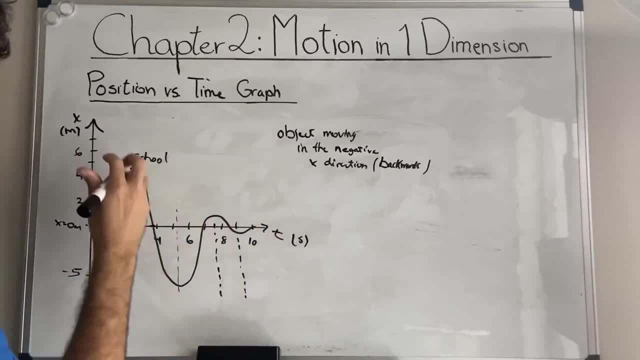 solution. this is: you go to the store far away past your home. you go to the store to buy some, after which you return back. you return, you pass your home again on your way to school, and then you realize you want to eat something, so you stop at. 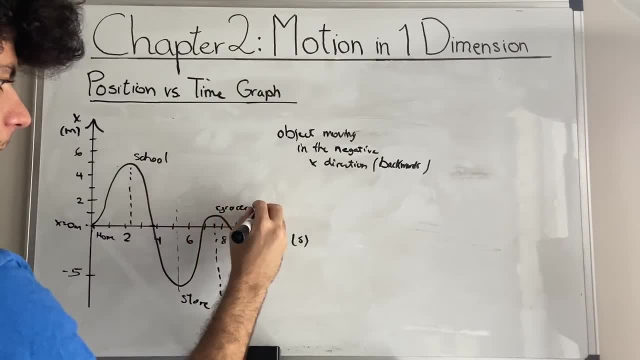 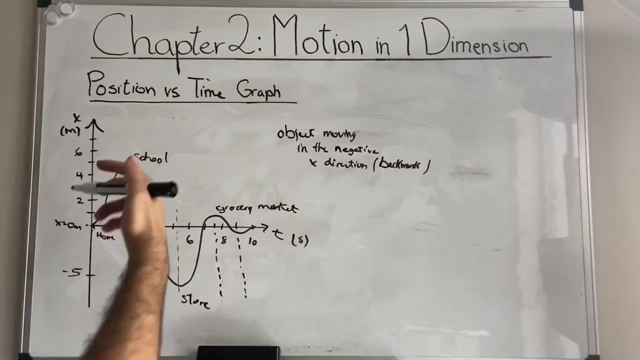 the grocery market and note that you're passing home in this situation and this situation and that's pretty much it. this is just a, an object moving back, forwards and backwards, and forwards and backwards, right, and the first time it moves very far in one direction, then it moves very much far in the other. 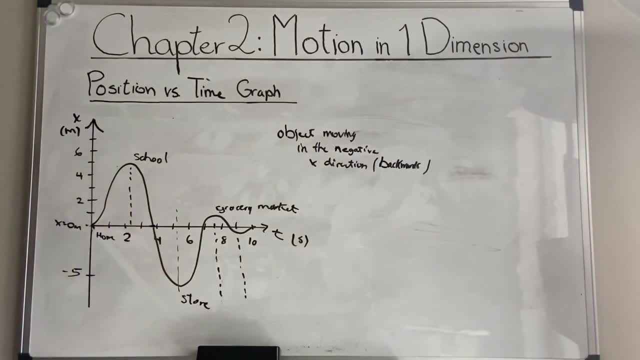 direction and even passes its starting point. then it heads back to its starting point, passes a little bit and starts going backwards a little bit behind its starting point, and that's that. repetition is what is happening over here. all right, okay. and another very important concept for position is: 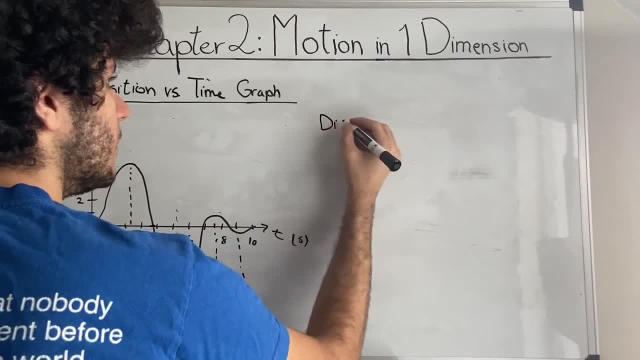 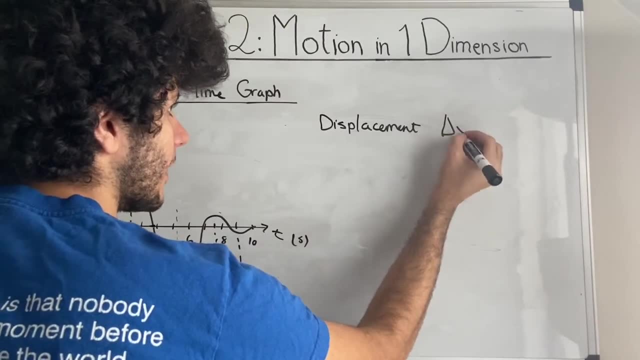 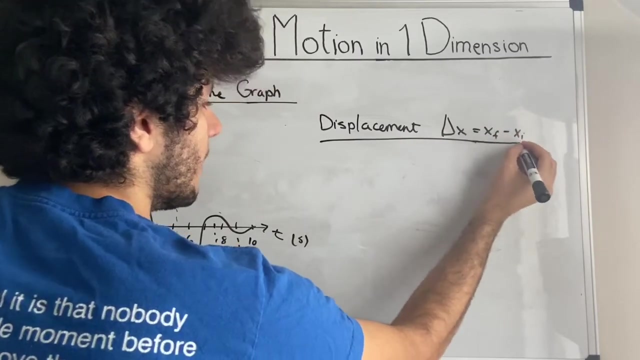 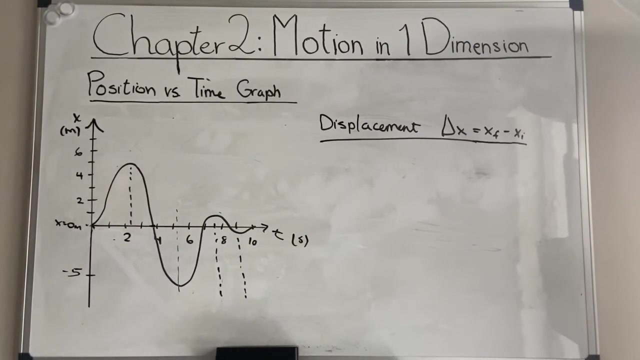 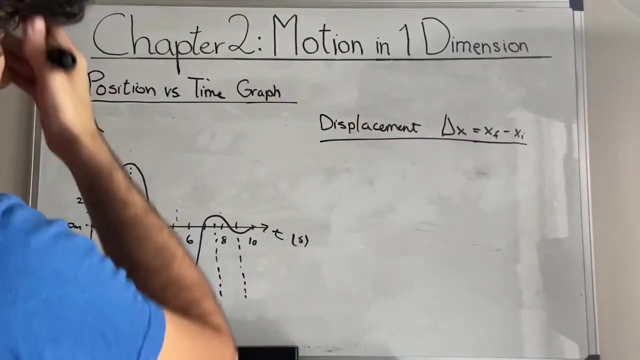 displacement. we will define this as Delta X, right, so Delta X is equal to X, final minus X. initial. displacement is basically the distance, the final distance. well, actually, just the change in distance. that's what Delta is, the change in something. in this case it will be of X, which is our unit of distance, of length. so our unit, our. 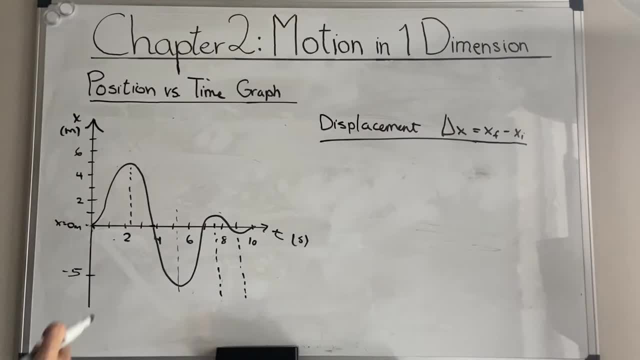 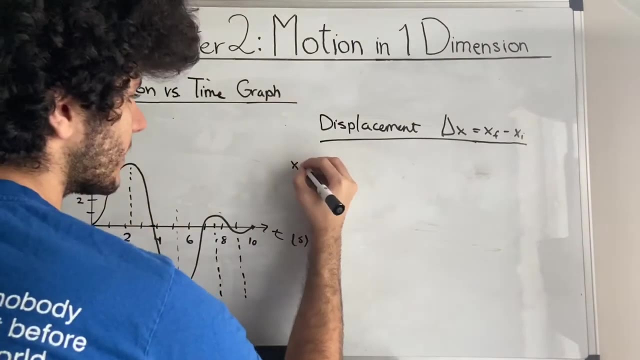 measurements of length. so basically, if you head to, you get head to school, head back to a store or go to the grocery store, blah, blah, blah blah and end up straight on X equals 0, we have: X initial is equal to zero meters over here. X final is: 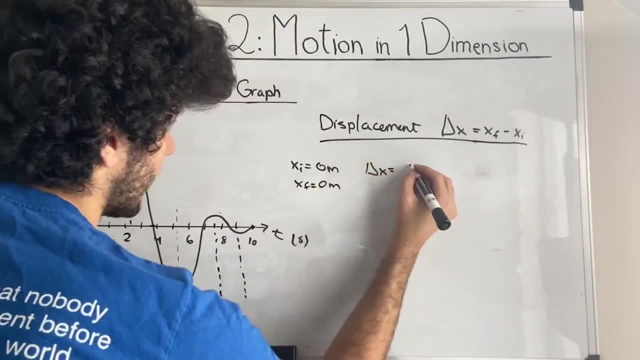 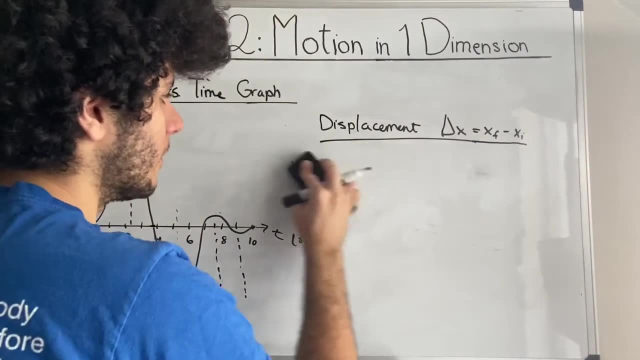 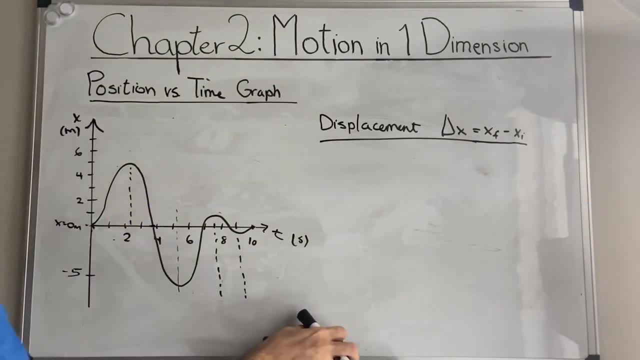 equal to 0 meters. thus the Delta X is equal to 0 meters, since final minus initial 0 minus 0 is 0. right, give, let's see that. yeah, so an example. let's know that. let's check another example out. so if we're dealing with a situation where 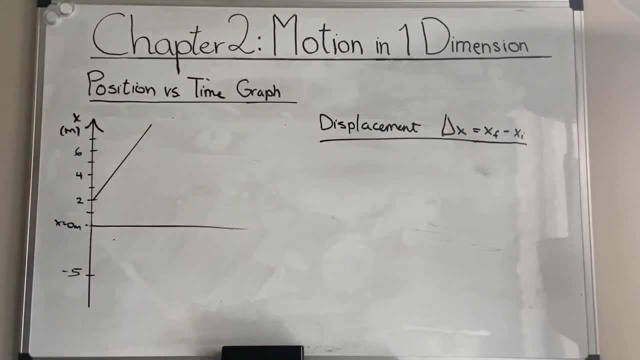 the initial point of the. so, basically, if we have so, one of the remark is that if the graph does not start at 0, 0- not to panic- that just means that the, the object starts at x equals 2 and then starts moving the positive X direction, or I was moving in the negative X direction. the 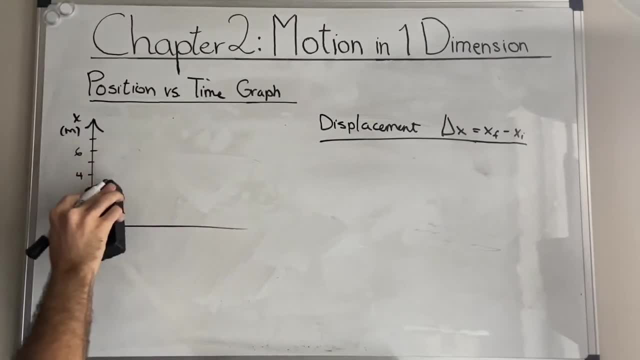 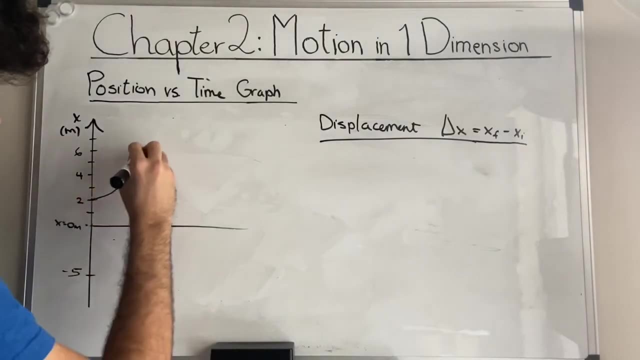 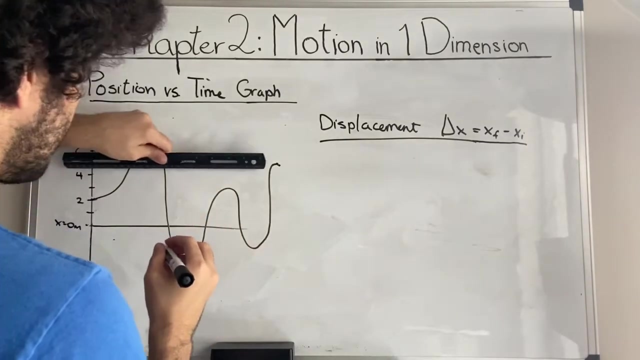 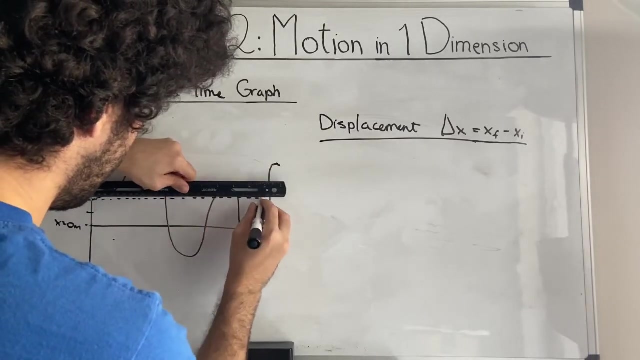 important is. important about displacement, though, is that, regardless. The displacement does not care about the journey, It only cares about the end point, Say, we end over here. What the displacement cares about is this: It is the distance between the initial and the final. 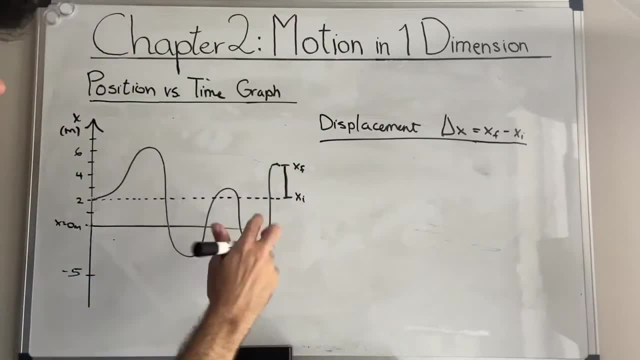 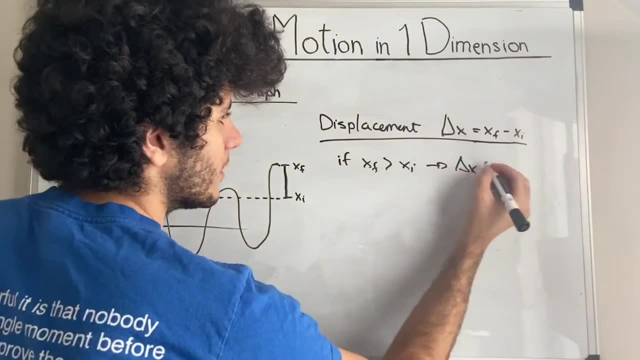 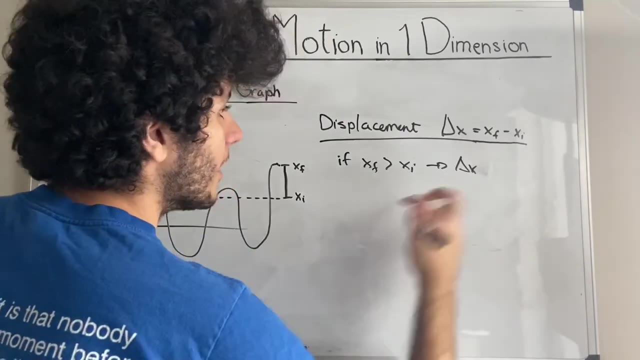 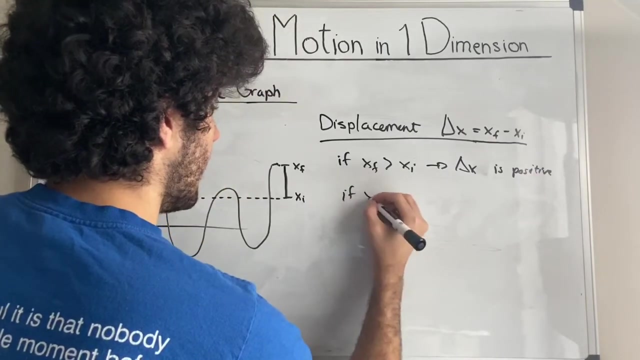 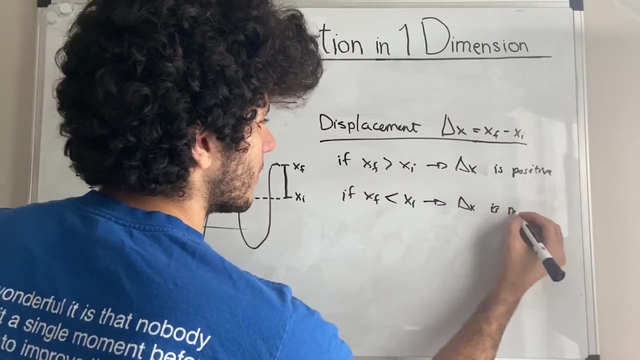 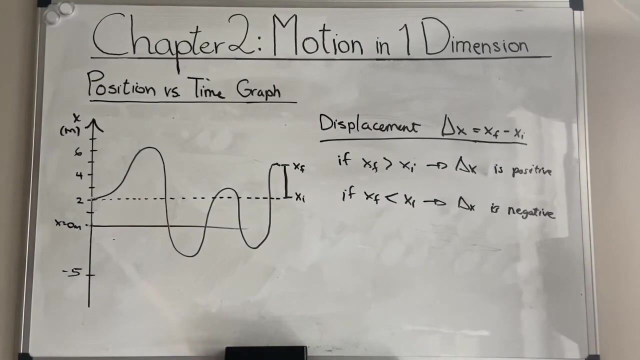 And it's calculated from final to initial. So if XF is larger than XI, then we have a positive displacement, If XF is smaller than XI, then we have a negative displacement. All right, so that's one of the big notions of position, right? 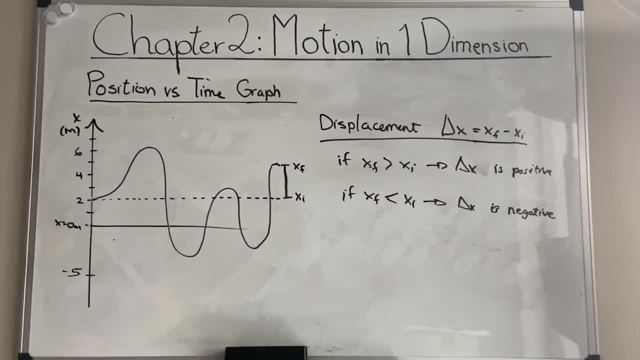 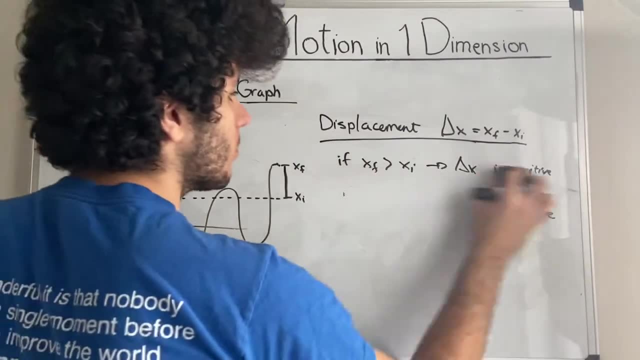 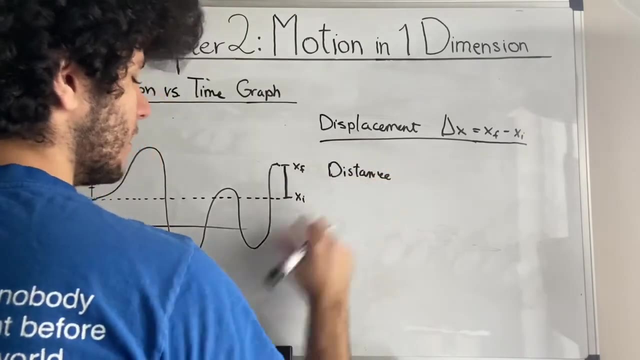 So there's displacement and it's worth noting that there's also distance right, And we really- and I mean really- don't want to confuse displacement with distance. Distance is not Displacement, right. That's what I've been trying to say for the past 10 seconds. 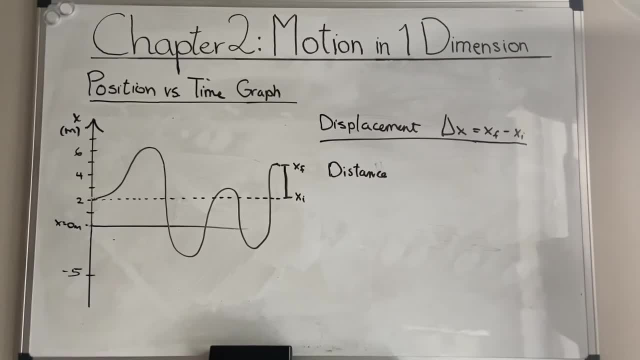 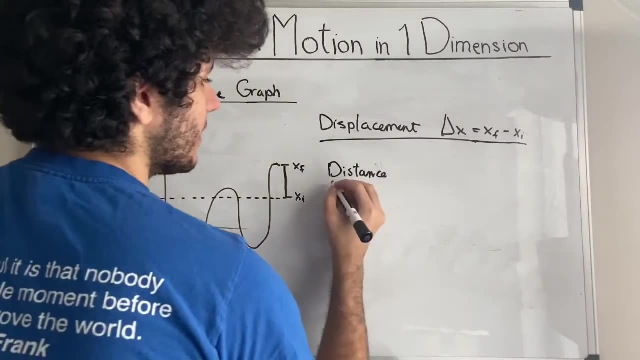 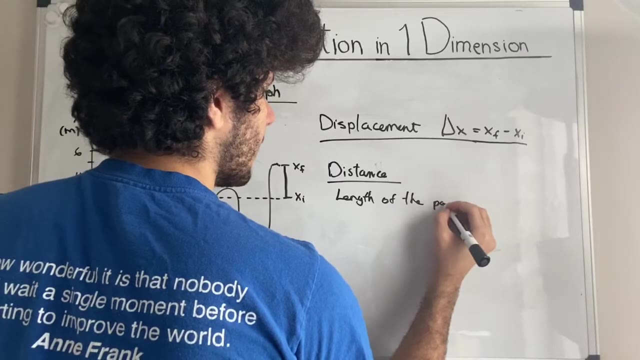 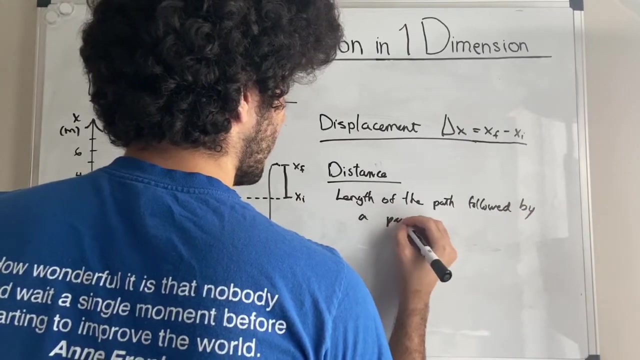 So it's very important to recognize the difference between these two. Distance is the length of a path followed by a particle Distance. Length of the path followed by a particle. Length of the path followed by a particle. Length of the path followed by a particle. 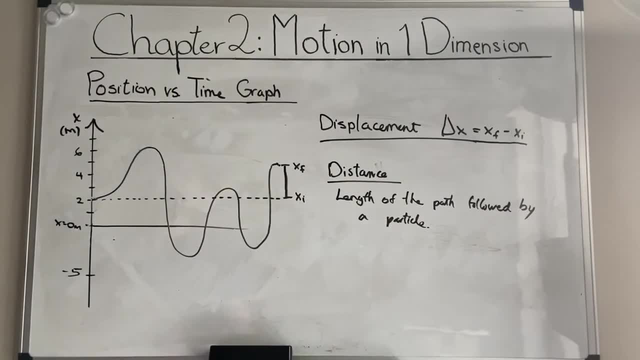 In that sense, displacement is very different from distance. Whereas distance would consider the change of, well, basically, how far the object has, just Just the length of the path followed by the particle, meaning, considering all of the ups and downs, The displacement only. 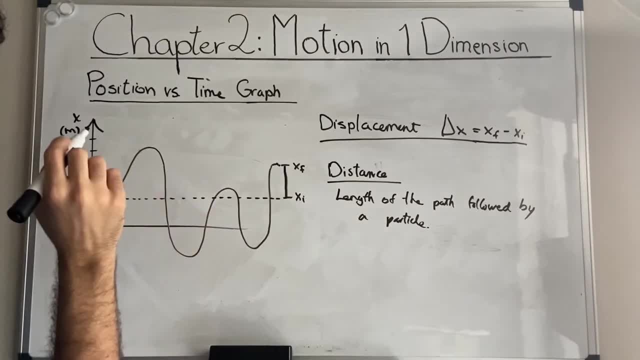 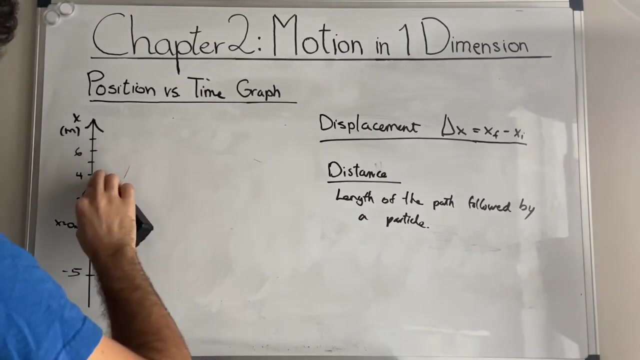 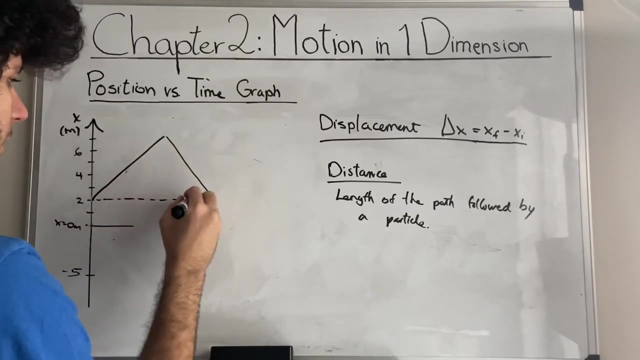 The displacement only cares about the, the final position with regard regards to the initial position, right? so an example. it could be that let me let me give you a good example where distance and displacement are clearly shown to be different. if we have this, so Timmy's walking from X is equal to 2 to X is equal to 7, and then heads. 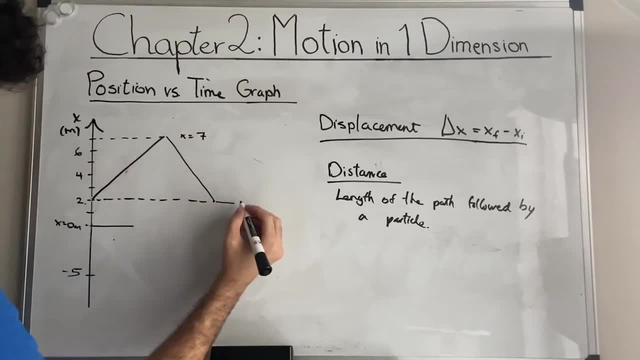 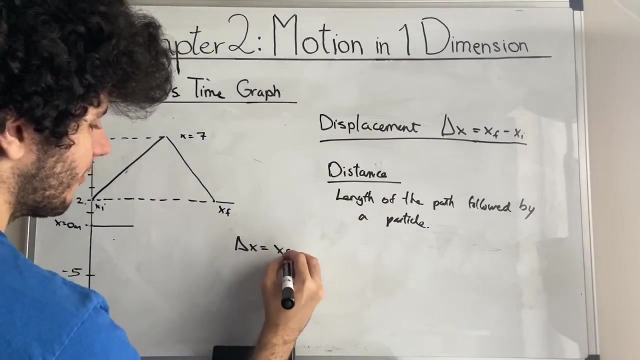 back to X is equal to 2 right, and this is his final position. his initial one is over here. well, if we're asked to determine both values to displacement and the distance, you'll see that we'll end up with two different results. the displacement can be calculated with that formula: X F minus X initial and. 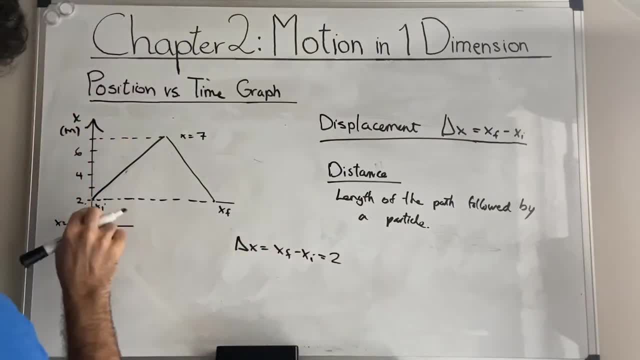 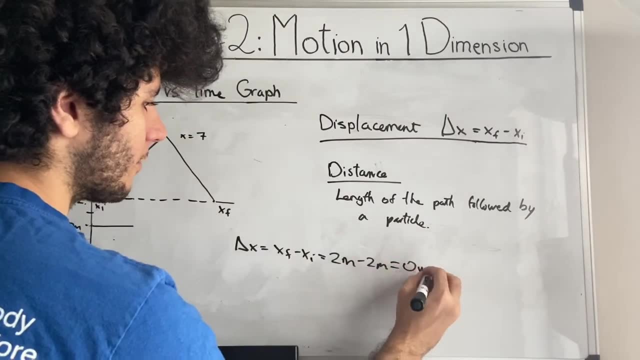 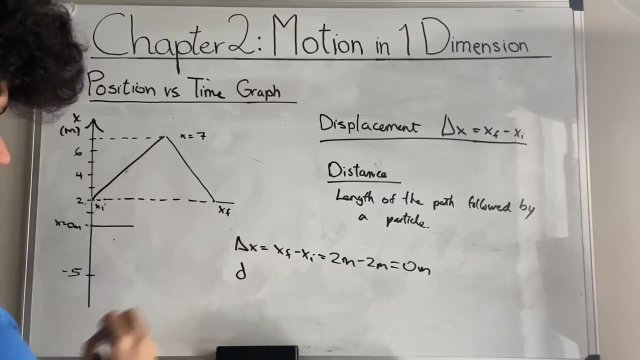 because in both scenarios, in at both the final and initial position we step, we have two meters. we end up with zero meters of displacement right. on the other hand, the just distance which we denote with G will not be zero right. so if we're asked to determine the distance between X and the initial position, 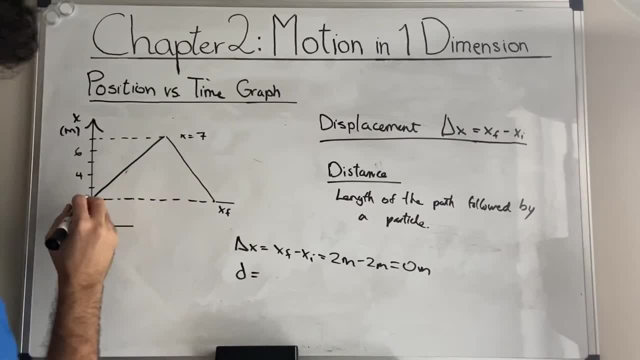 distance will consider the fact that, um just so seven minus two, five meters were traveled in this initial bit and then five meters were again traveled in this little bit. so five meters over here and then five meters over here, even though it's in the negative, the negative direction. 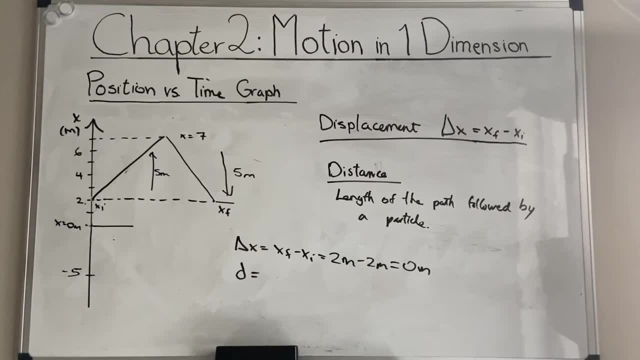 fuck, even though it's in the negative direction. fuck, I don't want to do all this, motherfucking, okay. on the other hand, on the other hand, distance considers the five meters that have been traveled, one going up, well, basically in the positive X direction, and then the five meters when, Tim, you is going in the negative X direction. 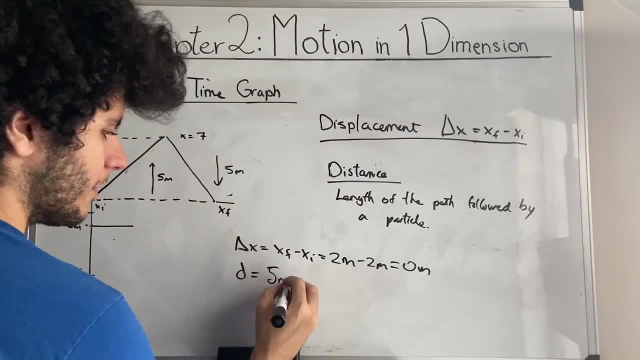 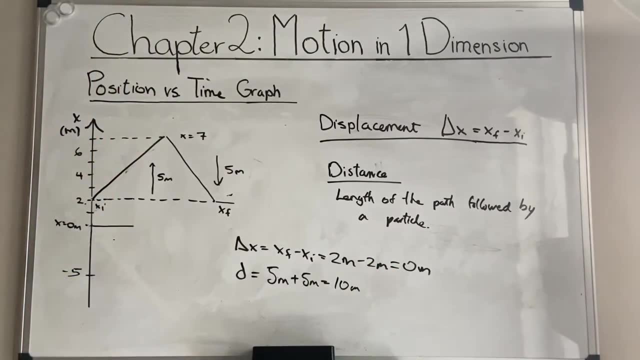 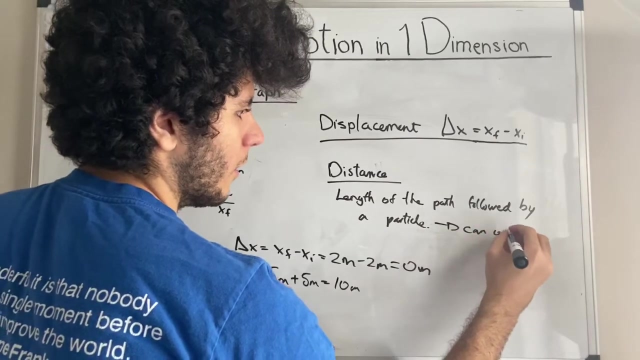 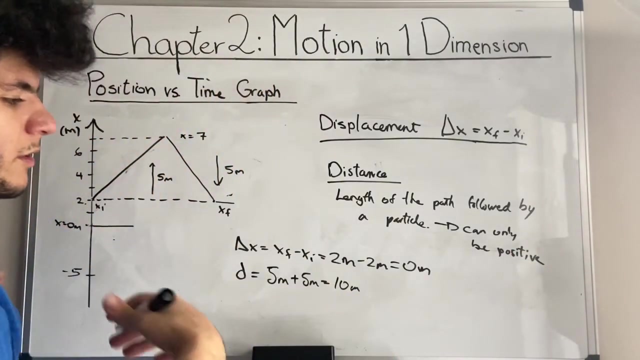 therefore, it is five meters plus five meters, plus five meters, plus five meters, which gives us a total distance traveled of ten meters. right, so, that's pretty much it, and it's worth noting that distance can only be positive, can only be positive. you can't travel in negative distance. however, you can travel. 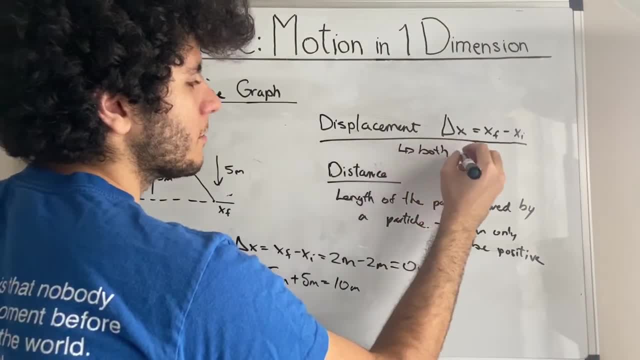 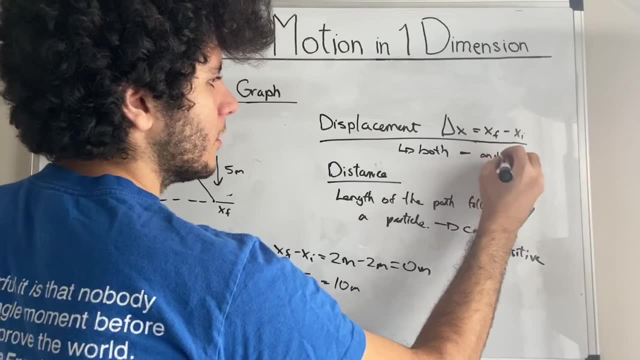 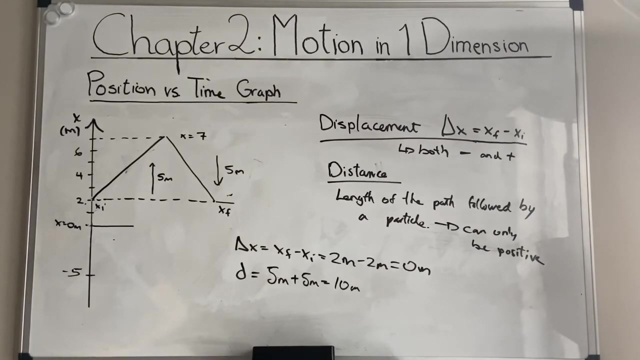 negative displacement. Well, not travel a negative displacement. You can have a negative displacement, both negative and positive. There we go. That's a very important distinction we have to make right, And now we are going to move on to the next. 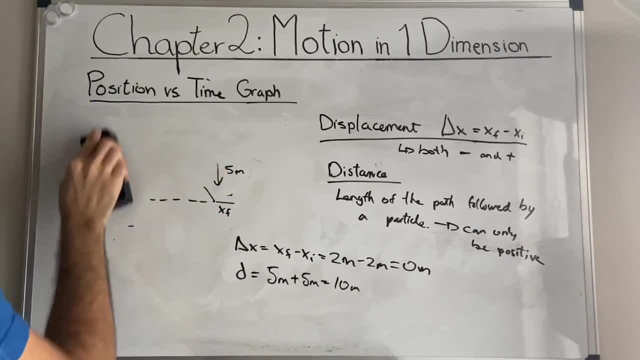 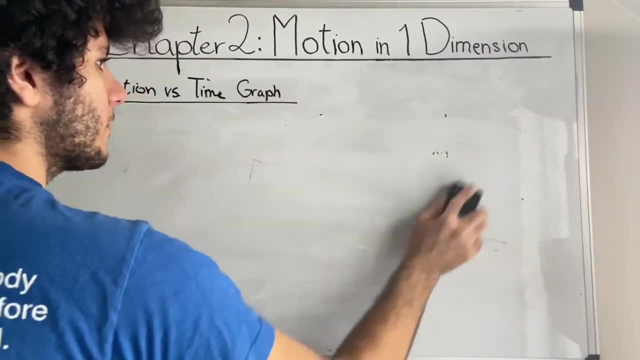 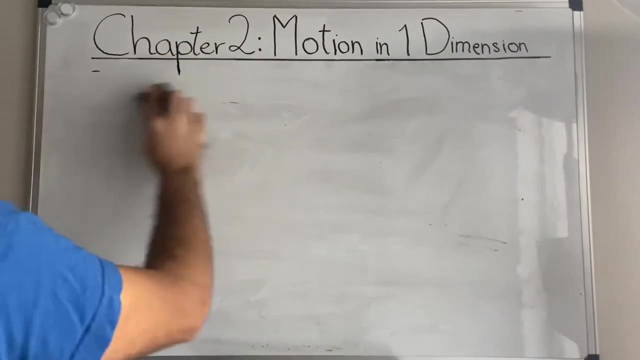 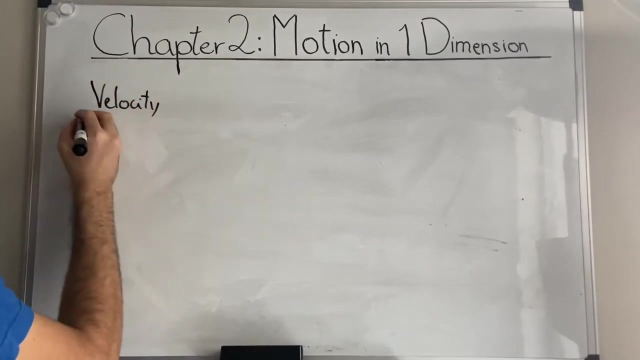 topic which is actually very related to position. It's velocity. I'm gonna go a little bit quicker over this. Velocity, All right. So velocity, What is its definition? Velocity is the velocity of the direction of the wind. Velocity is the velocity of the direction of the wind. 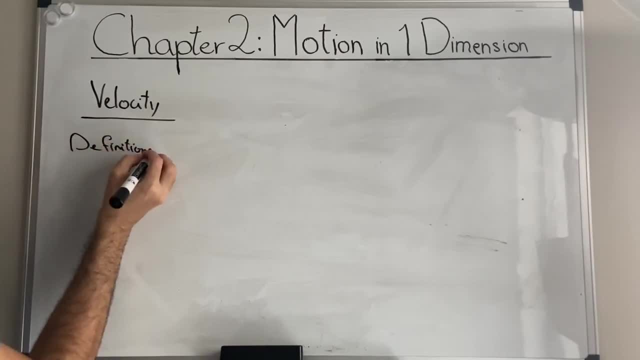 Velocity is the rate of change of position. For those who have taken calculus, you'll notice that this is a very specific way of defining velocity, right? So we're going to see how calculus can actually play in the direction of the wind. So we're going to see how calculus can actually play in the 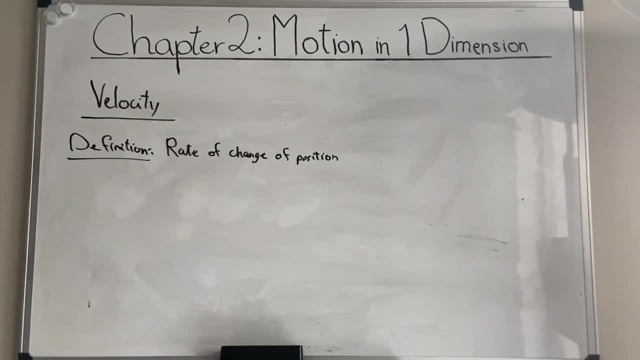 physics And it's going to play a lot in physics. So that's why we recommend students take physics along with calculus or take calculus before taking physics, because a lot of things won't be properly understood if they have not yet taken physics First. we're going to go over. 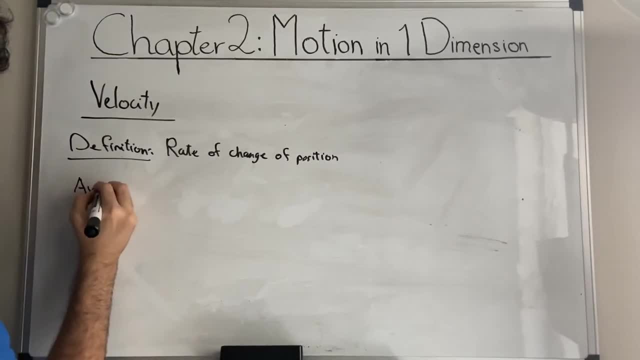 average velocity. Average velocity- Right So average velocity is denoted, right So average velocity is denoted as such. velocity V of average equal to Delta X over Delta T. we're gonna use this formula quite a lot, and we- this is the way that we write. this is so. this is. 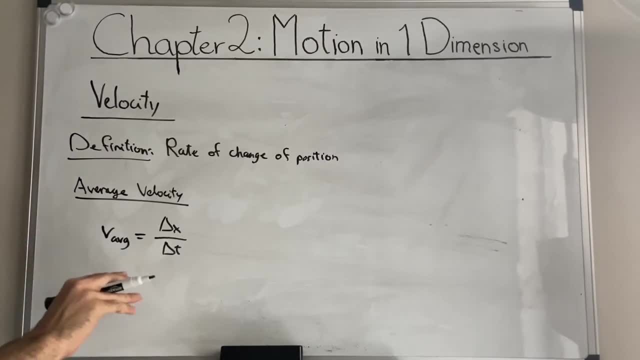 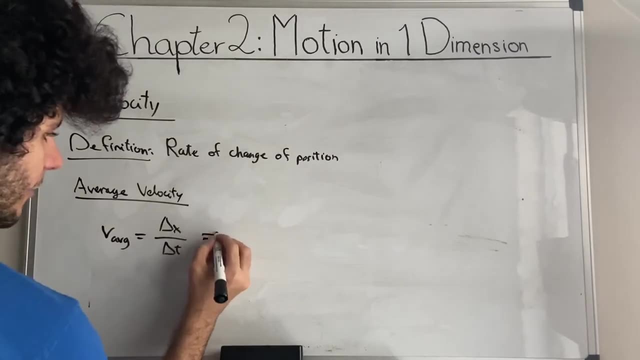 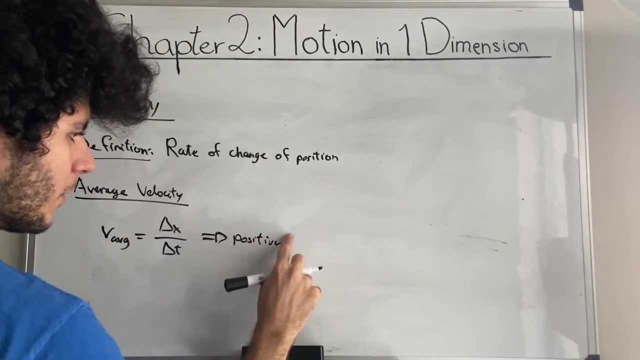 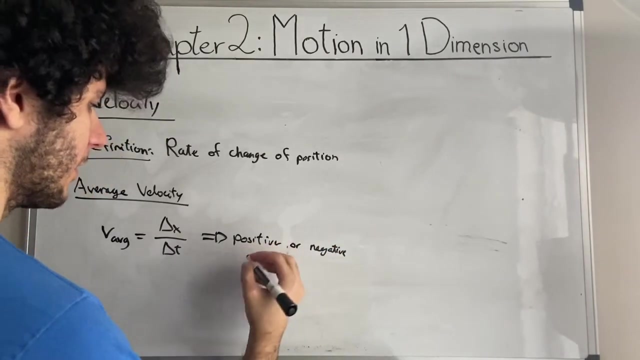 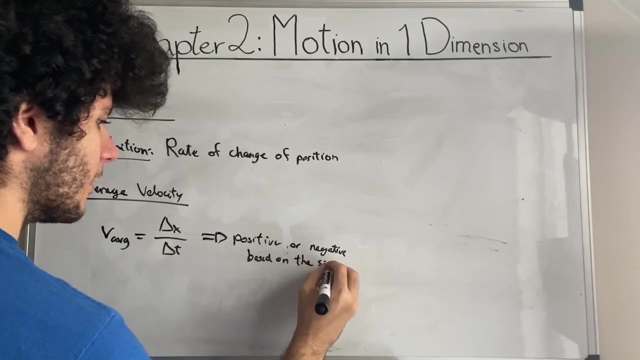 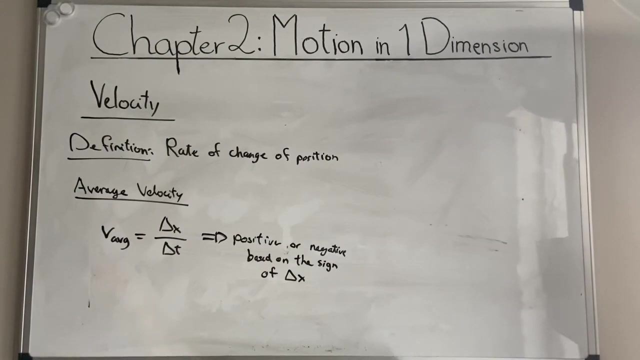 basically a displacement divided by the time interval during which that displacement occurs, and this can either be positive or negative. oh, let's not drop that. base based on the sine of Delta X, right? so that's actually a very important, very important detail. velocity can be negative and generally we mix and match of velocity and speed. 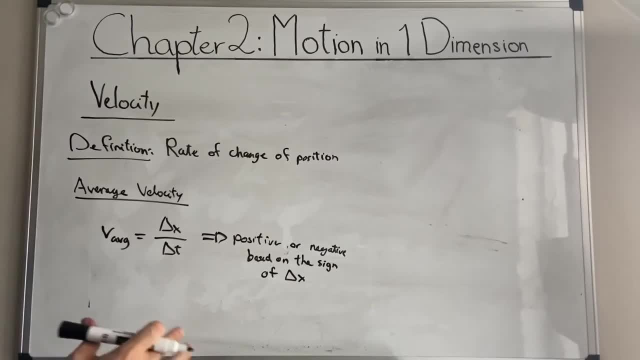 like they're the same thing, but we're gonna realize that in the next few minutes we're gonna see how velocity is not the same thing as speed. they're very, really, they're very relatable, but not exactly the same thing. the average velocity can be negative, right, and it can be positive. 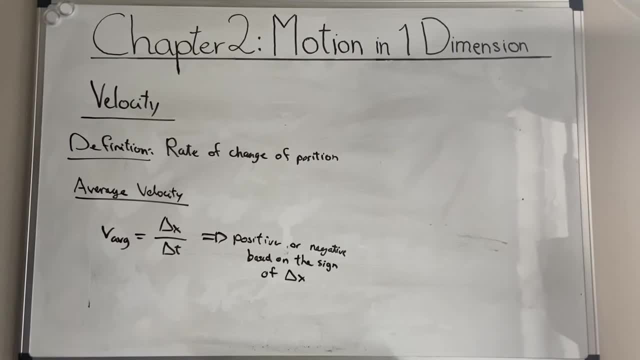 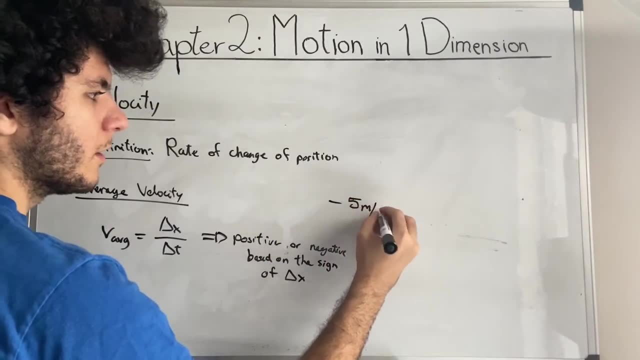 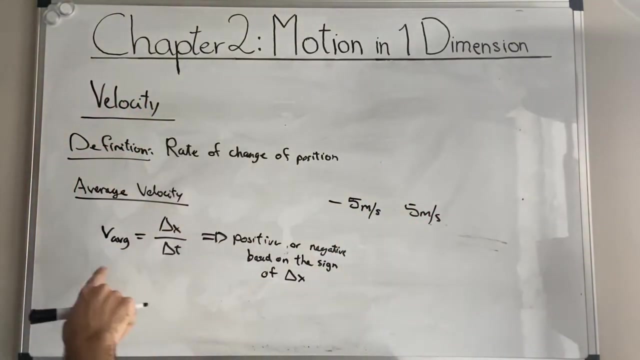 and negative velocity is similar to positive velocity. if we have the same, if we have negative five meters per second and then we have five meters per second, these are very similar velocities, or let's call these average velocities, right, they're very similar. however, the sign is different. and what does this? 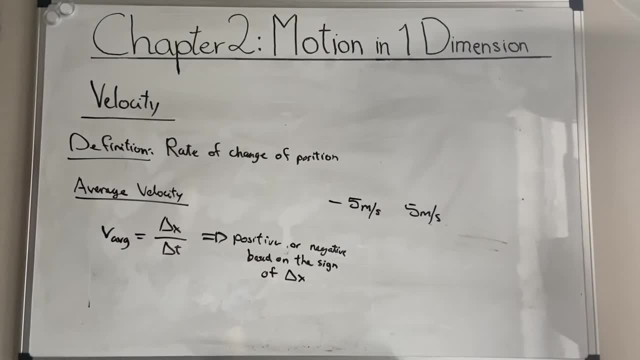 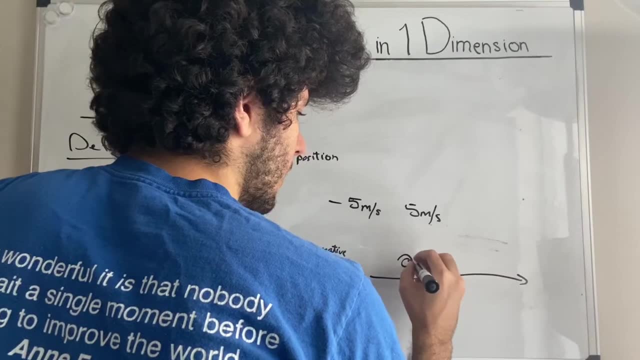 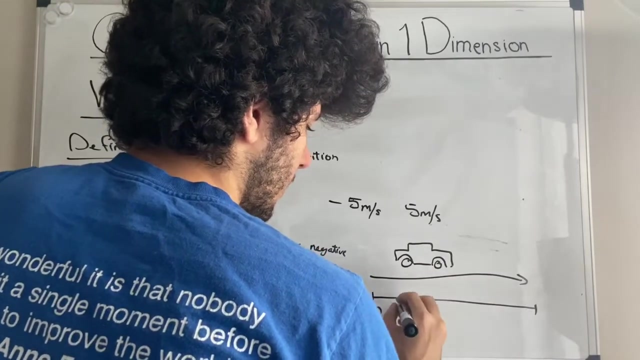 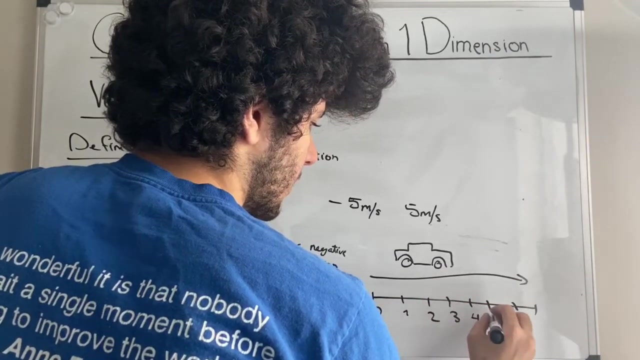 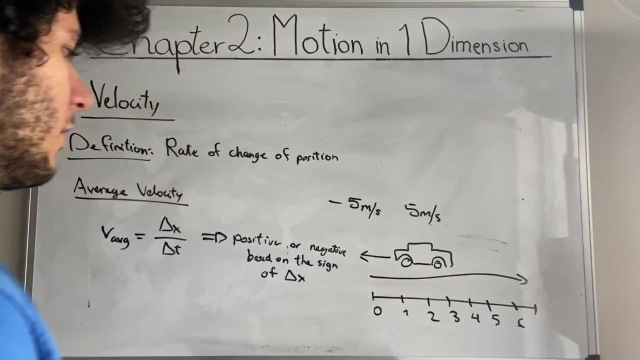 mean actually? it means that the car that we're talking about- I guess let's say we're talking about a car if it's along a- you have an instrument to calculate, to measure what position it is, if it's heading in and the negative, well, if the displacement, the total, 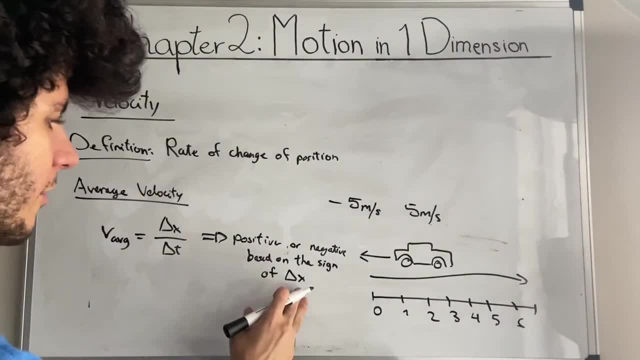 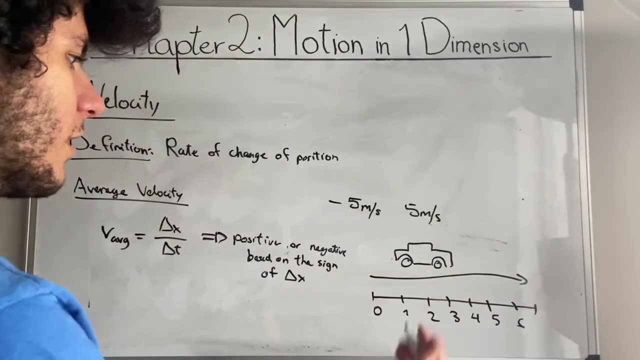 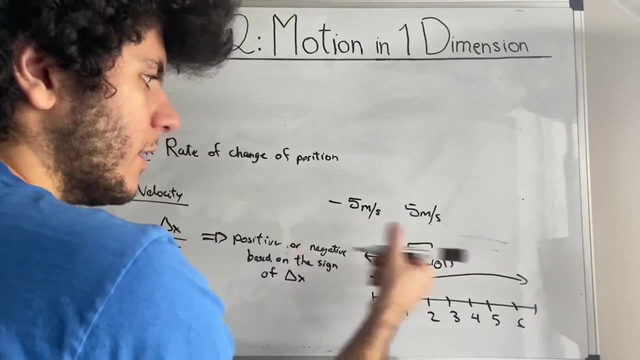 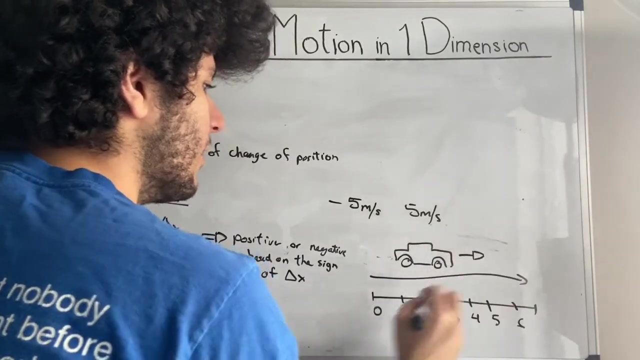 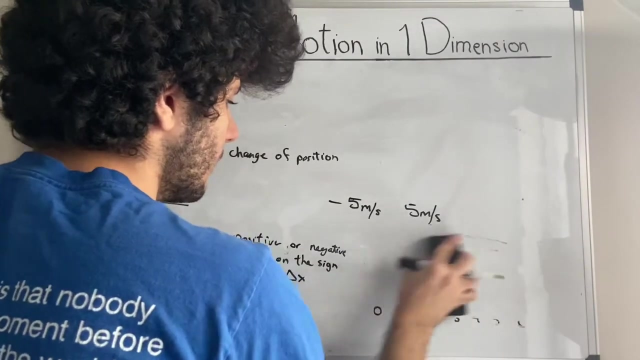 displacement, right. the difference between the final position and the initial position is negative, then the average velocity will be negative, right, and negative will probably just signifies that we're heading in the negative X direction. if the number is positive, then we're dealing with a positive X direction, right. that's very important to pinpoint. all right you have. 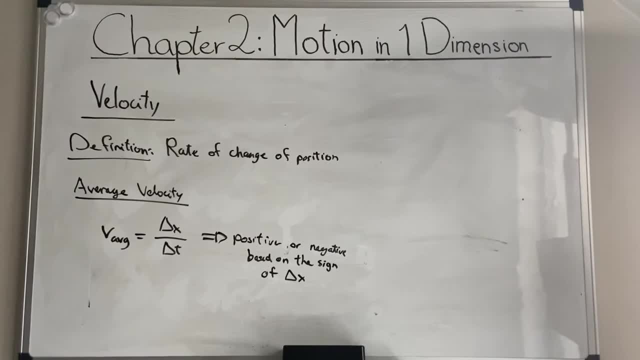 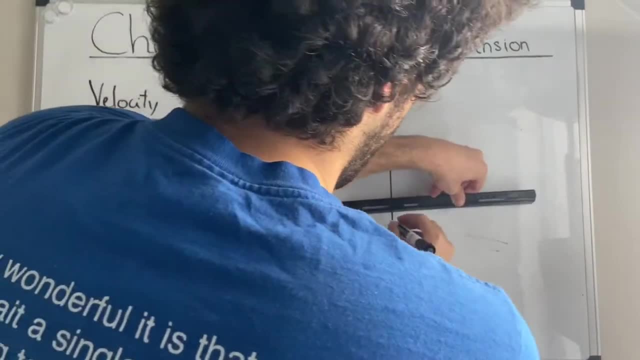 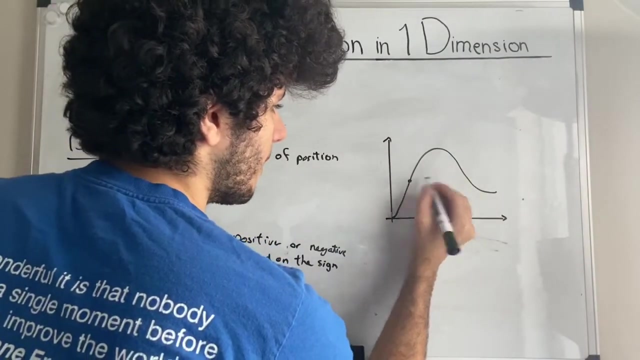 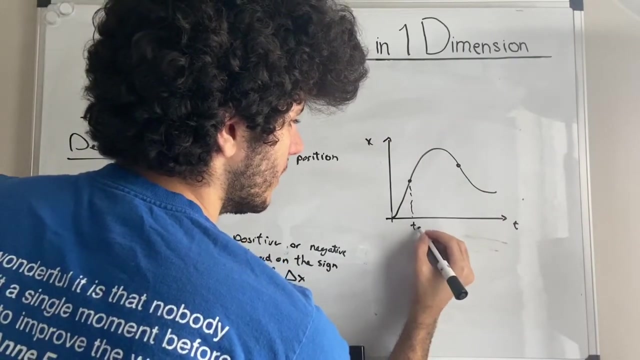 that stood, and if we look at a position versus a lot of position versus time graph, we can put this definition to use. say, we have something like this and we're trying to figure out what the average velocity is, and we're trying to find the average velocity between these two points, between TI and TF. well, the 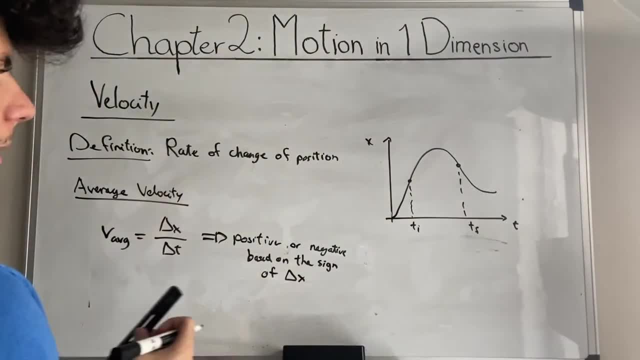 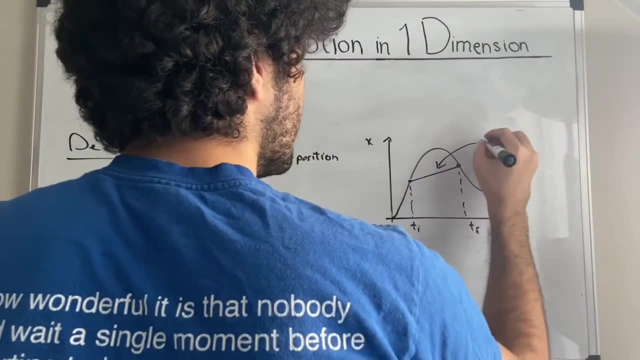 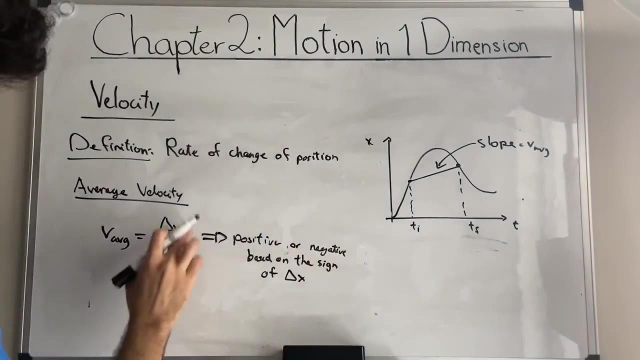 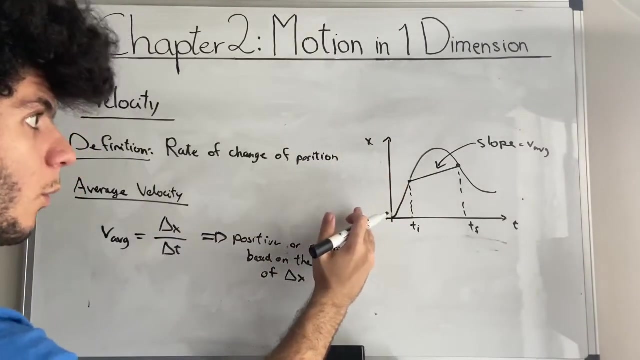 way that we, when we calculate the average velocity, we're basically considering both these points and we're drawing a line between them. calculating the slope of this will give us the average velocity, and you can notice that by taking a look at this equation. this equation is the change of, let's say, Y over the change of X. if this was. 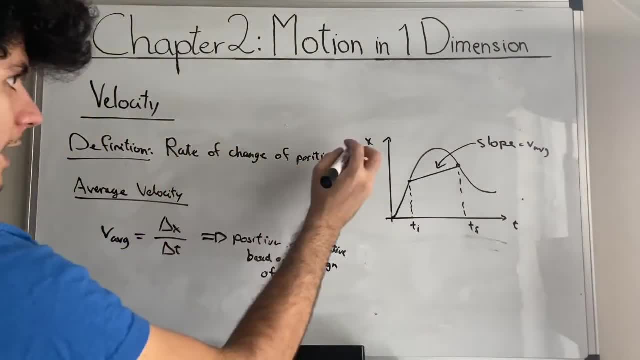 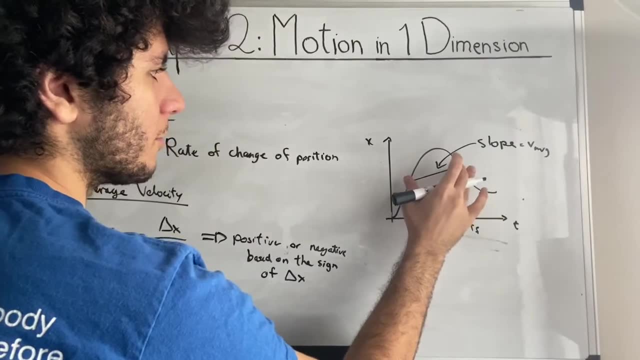 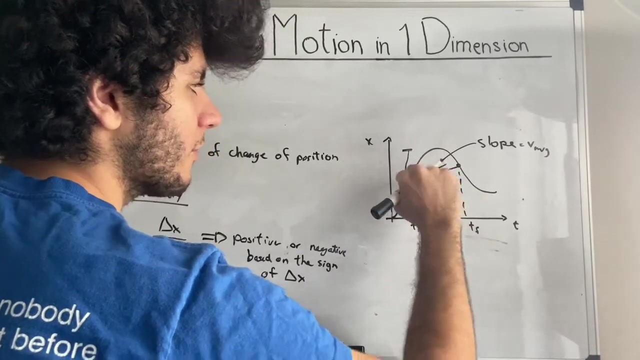 like regular math, right, except for we're dealing with X for position and time, right, so it's basically the slope of these between these two points. it's not. as you can see, there is other stuff above it, right, there is the. the graph continues despite this. this line. 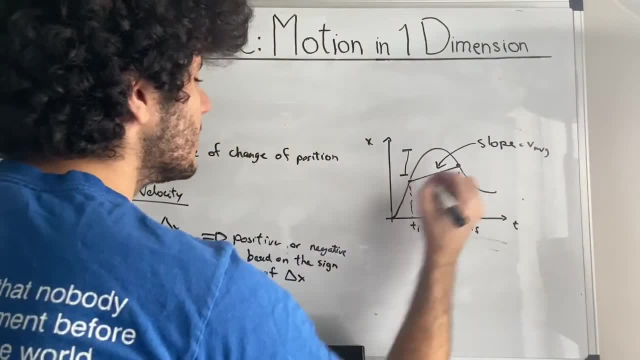 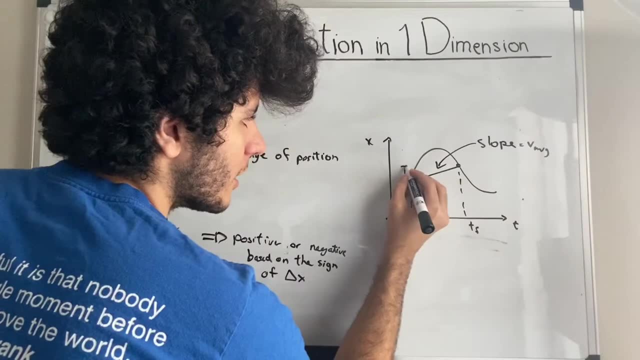 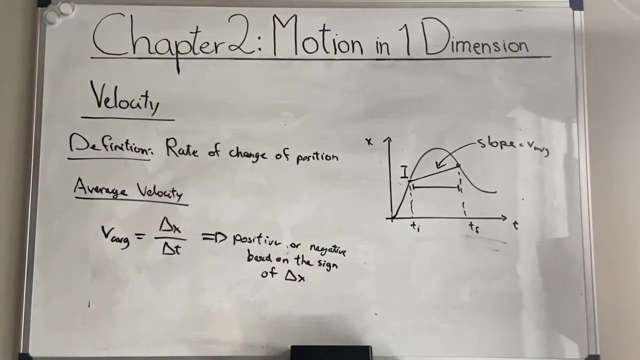 however, we're just trying to discuss the average velocity between these two points, and thus we don't we don't need to care about the rest over here. we're just trying to find the change in X, and then trying to find the change in Y, and then dividing one by the other, and that gives us the average velocity. next is: 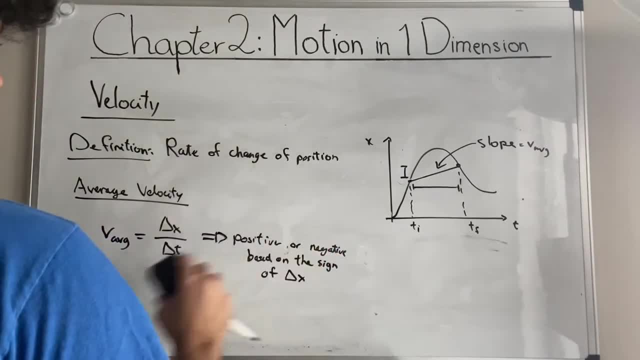 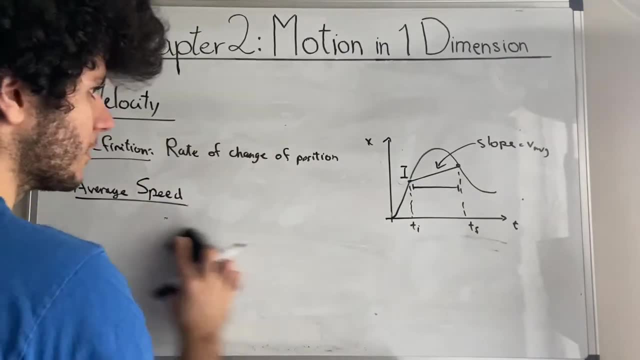 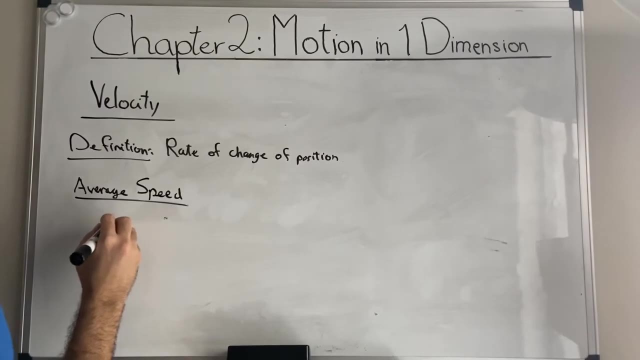 the average speed right, so I spoke about this earlier. I said we were going to talk about this, and here we are. average speed is very, very similar, though the way that we denote it is like this: average speed is equal to D over Delta T, so it's. 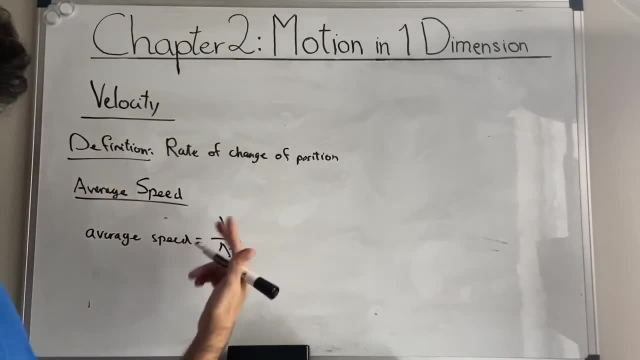 distance covered divided by the interval of time over which that distance has been covered. right so the total distance traveled, than a developer who simply us divided by the total time interval required to travel that distance. The average speed has no direction and is always expressed as a positive number. Oh, and it's worth. yeah, so, um, average speed. 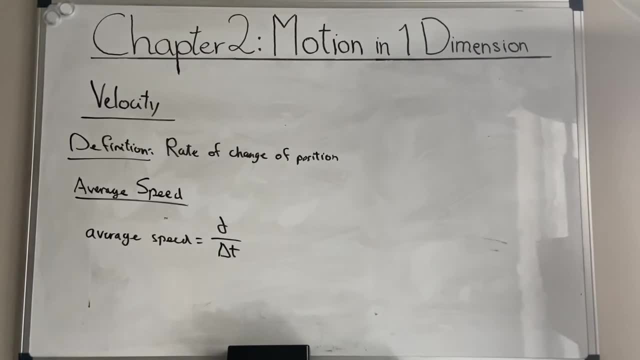 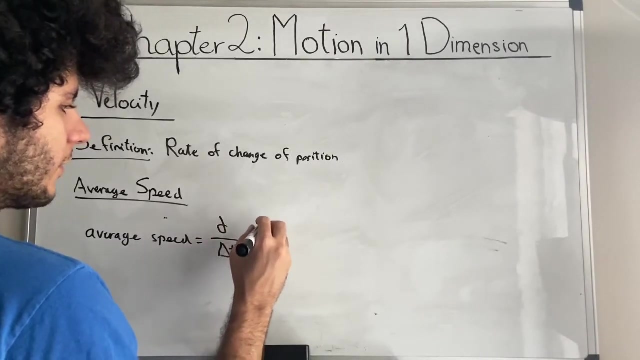 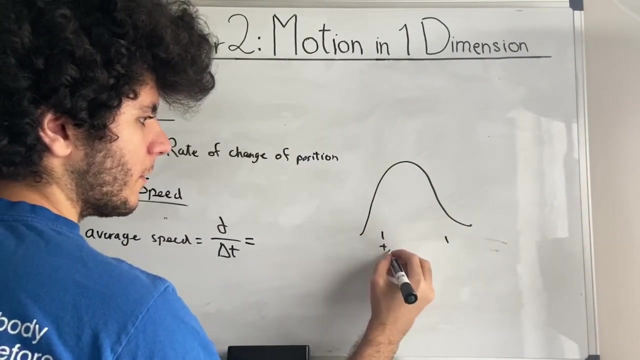 has no direction is always expressed as a positive number. so because it is, it has no direction. it has no direction because of this distance. it's just. this is just a scalar, a number, right, um say, we travel a total. say, in that situation, here, over, in that same situation, we're dealing. 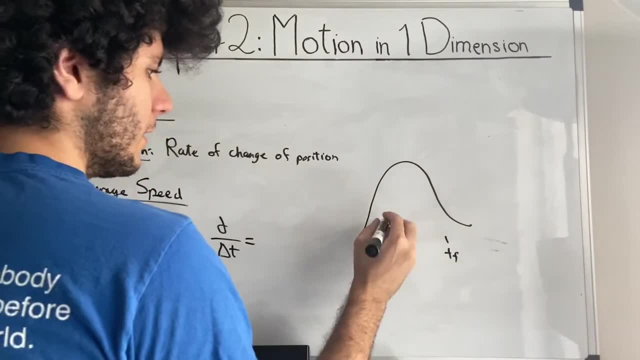 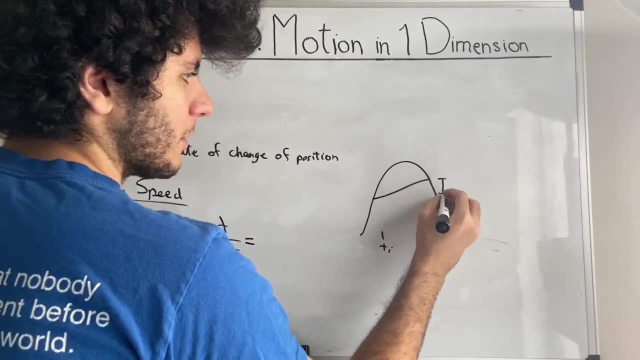 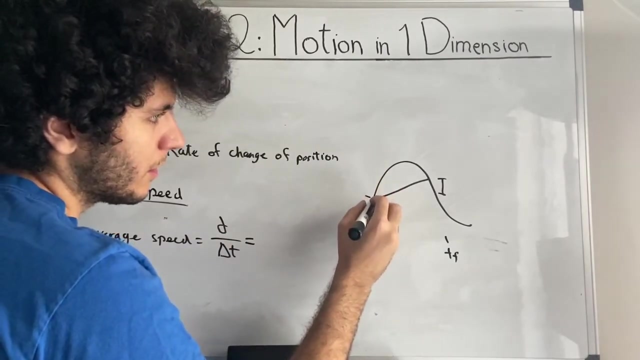 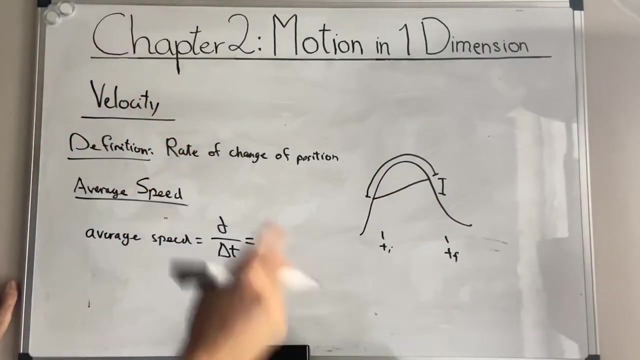 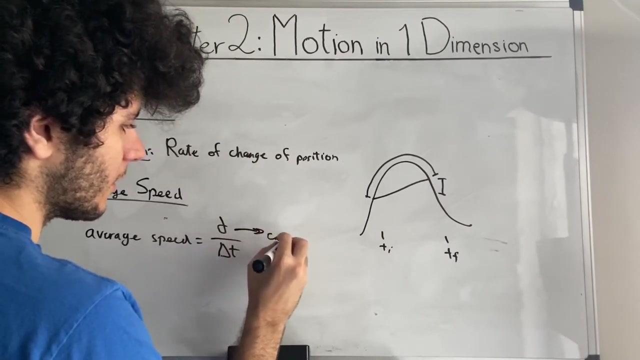 with before, say in between. so what we ended up doing before is what we can. is we calculated the displacement, which is this: but the average speed would consider the entire distance covered divided by time, and that's how we differentiate velocity, average velocity from average speed. it's um, and also it's worth knowing that this number can only be positive, because this can only 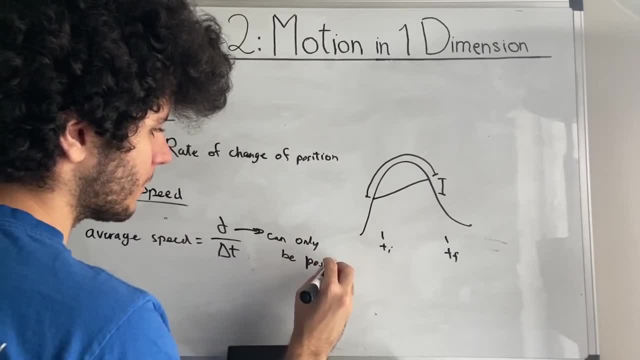 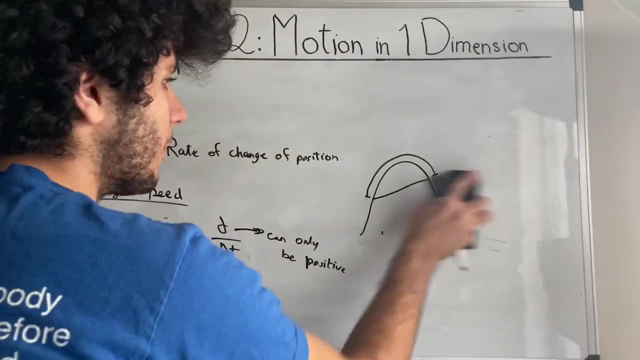 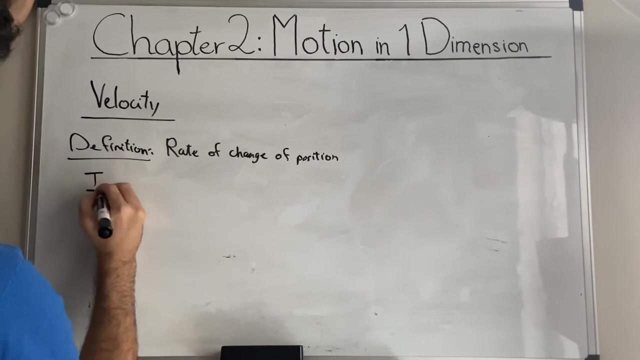 be positive. all right, um. next is a one of the most important, one of the more important forms of velocity, which is instantaneous velocity. let me erase that instantaneous velocity. there are a number of ways that we can write this right um, and we're going to start using 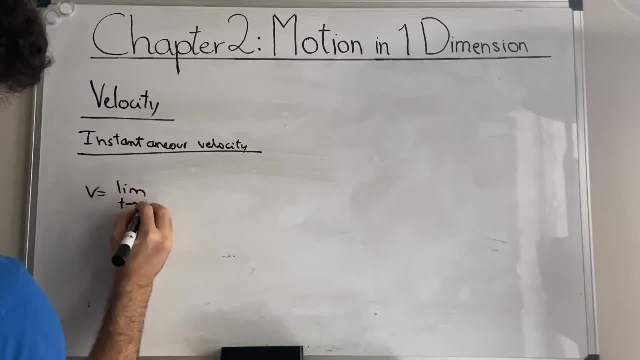 this. here it's the limit, as delta t- my god, delta t approaches zero for delta x over delta t. so this part of the equation is the same as for the average velocity. however, because we take the limit, we are dealing with a derivative. so, um, what this tells us is that 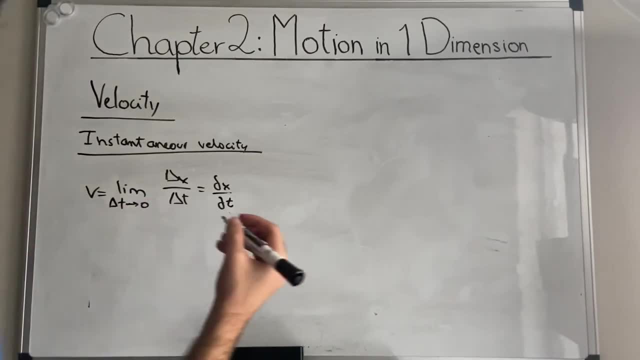 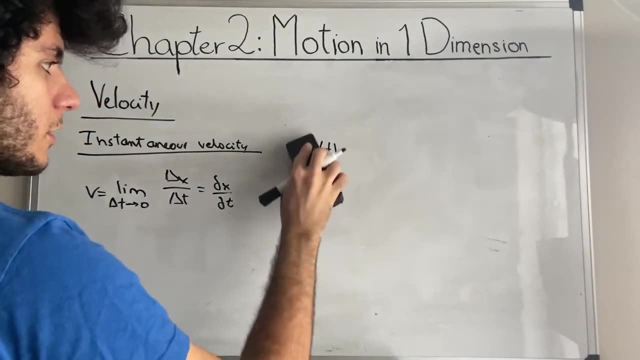 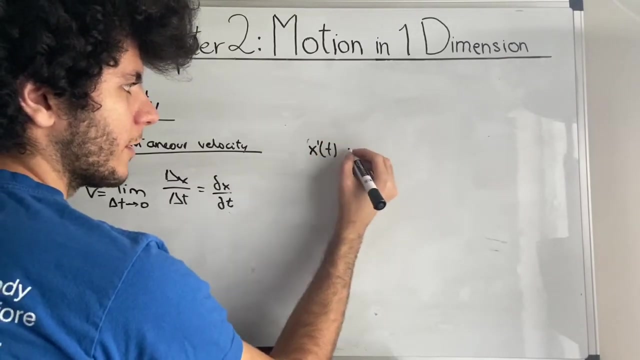 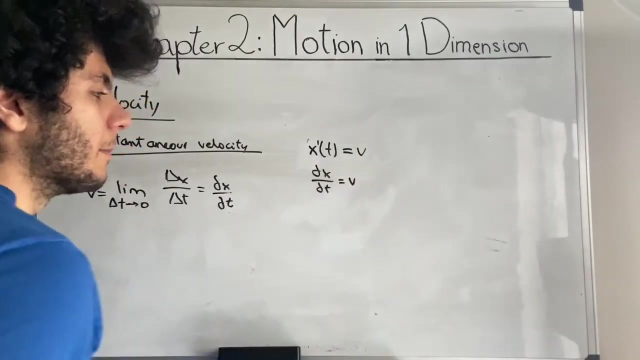 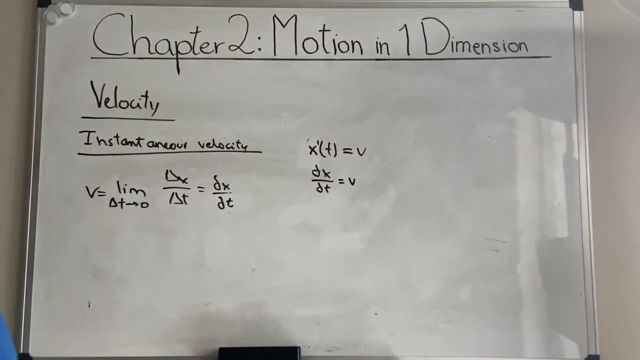 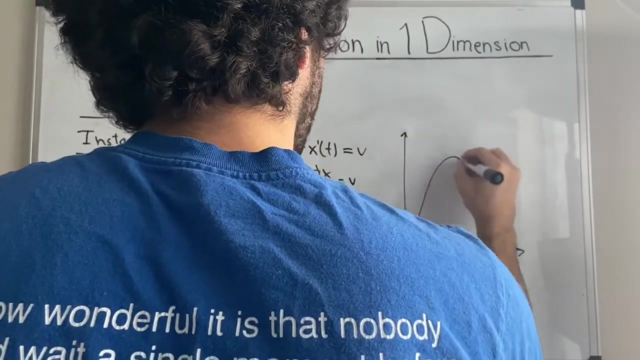 the derivative of the of the position function. right, if we take the derivative of this, either by placing that over there or by doing dx over dt, we obtain v in both situations, which is the instantaneous velocity. and what that means is so, if we have a, a graph- let me try this really quick- if we have a graph like this, 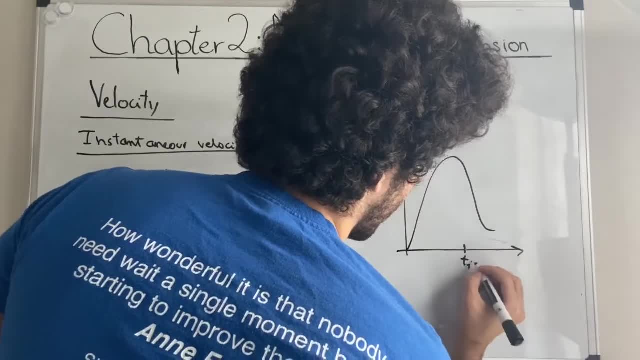 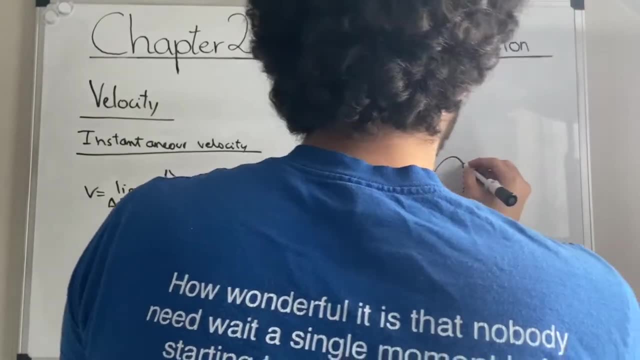 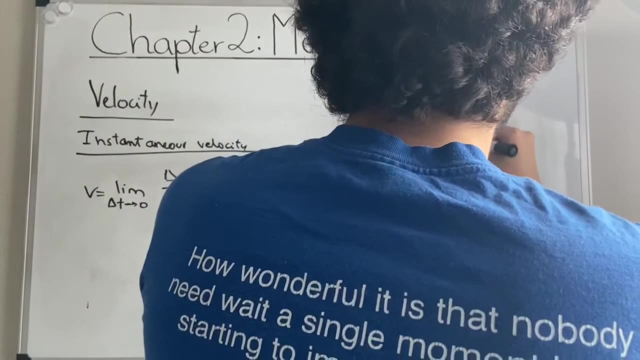 and we're trying to find the instantaneous velocity at this point t1, ti. then we're gonna pinpoint, point across the points on the actual graph and then we're going to try and trace a tangent to the graph. that will give us the tangent to the graph. that will give us the tangent to the graph. that will give 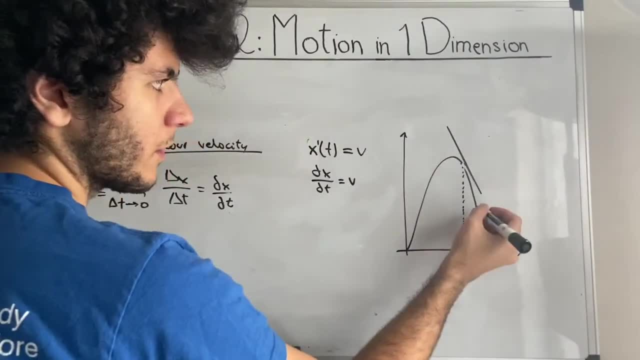 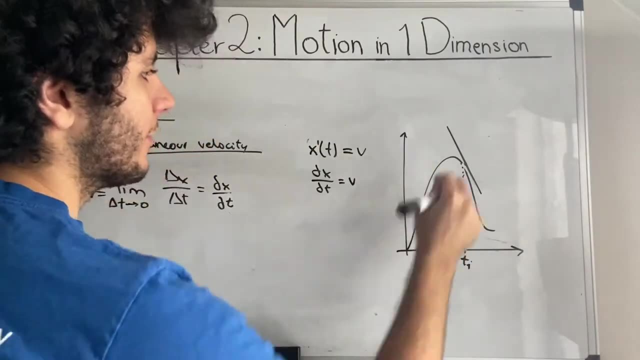 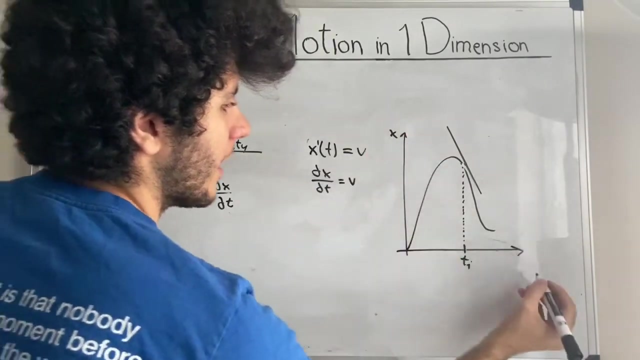 give us the slope of the graph at that point and thus will give us the instantaneous velocity At that point. what is the velocity of an object, right? Oh, and my bad, this is X and T, right. And if you dig a little bit deeper, 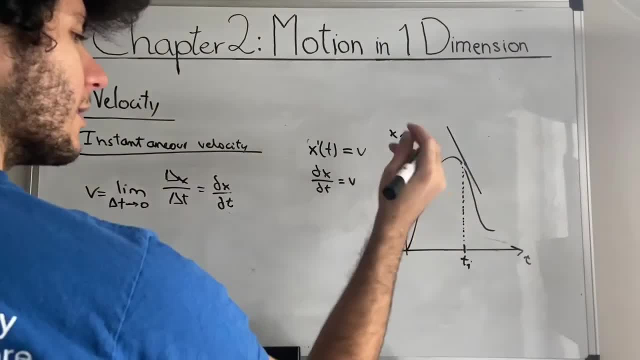 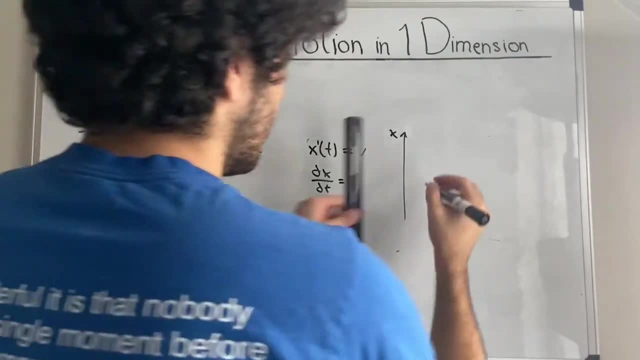 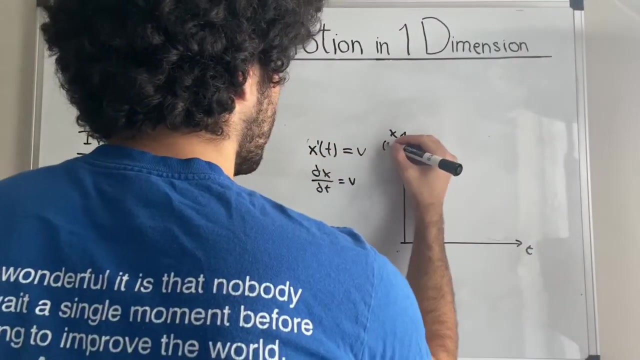 you'll actually realize that this does not only apply for, like, singular points, If we have a function right, As I actually already wrote it here- but if we have a function like this, like on a graph, if we have say something like this: very simple, 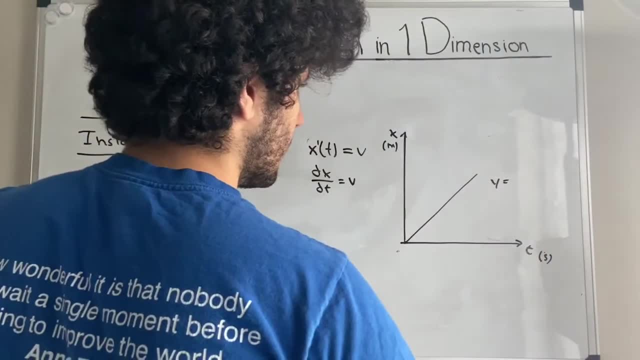 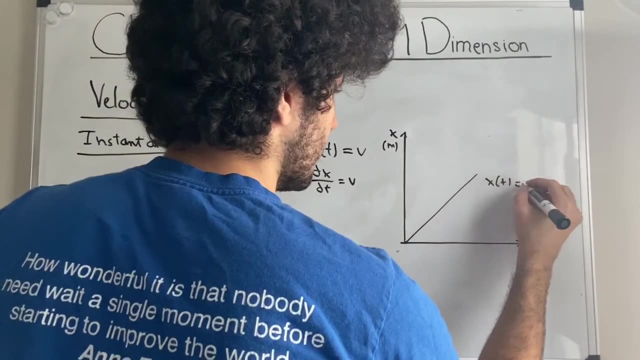 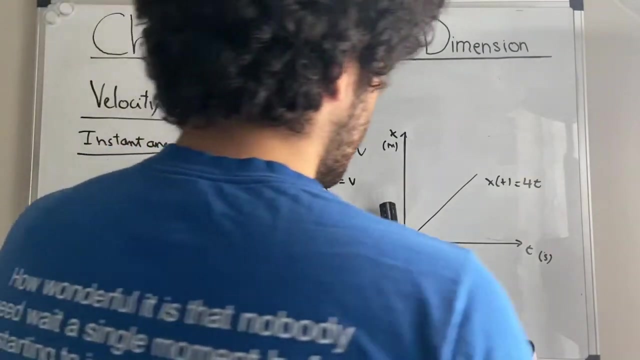 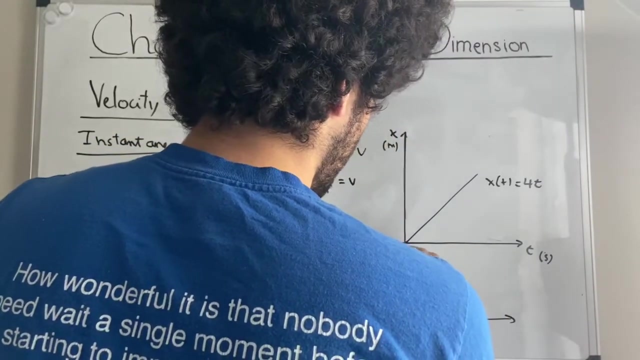 let's call this: Y is equal to. let's call this X of T. X of T is equal to four T, right, Okay? well then, if we're trying to find the graph of the velocity with respect to time, meters per second and seconds, 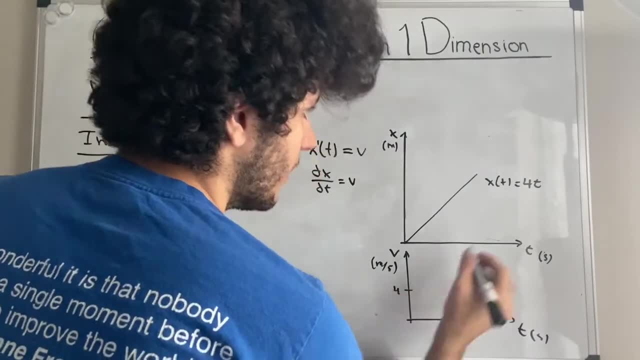 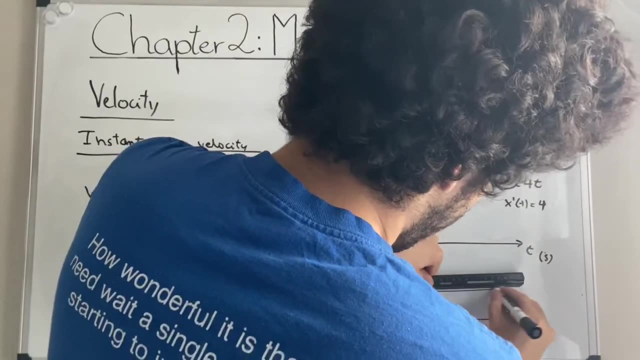 then we're actually going to just take the derivative. The derivative of this is four, and then we're actually going to just take the derivative. The derivative of this is four, and then we're actually going to just take the derivative, And thus we have a constant function for V right. 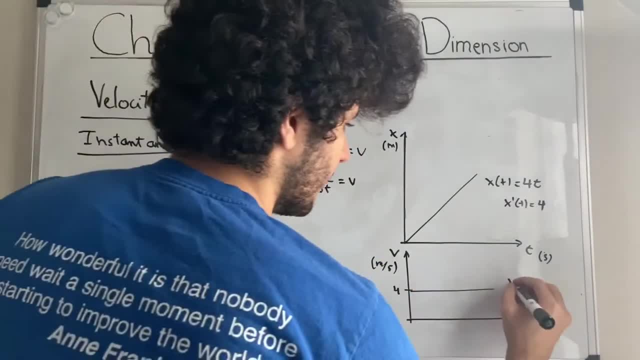 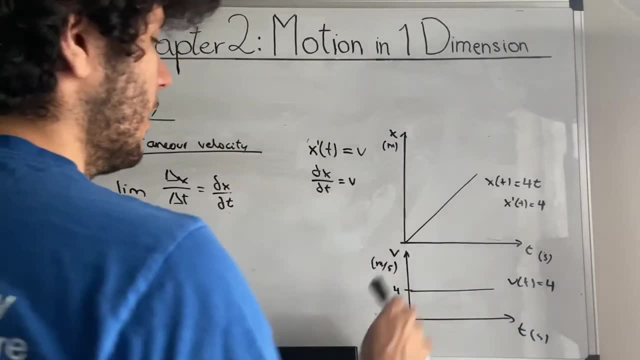 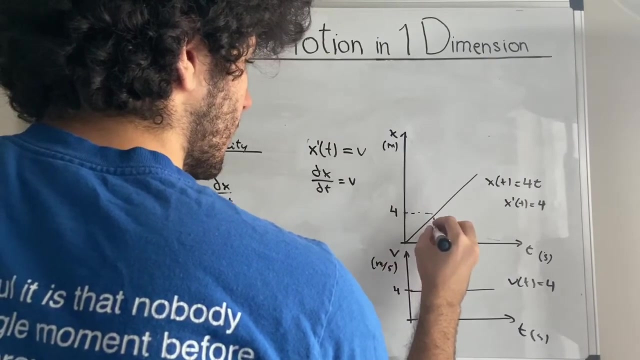 And thus we have a constant function for V, right. So we know that V of T is equal to four, And this is very helpful And this makes sense. if you think about it, An object is moving at a rhythm of so every four meters, one second passes. 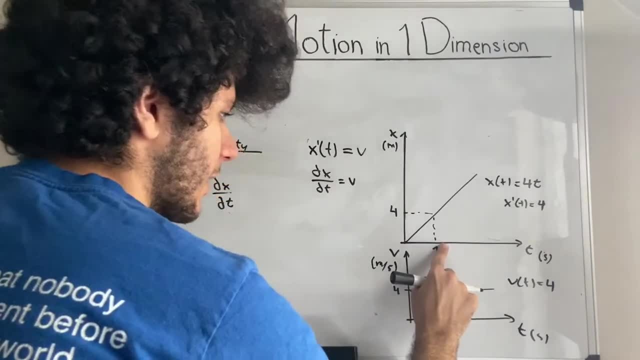 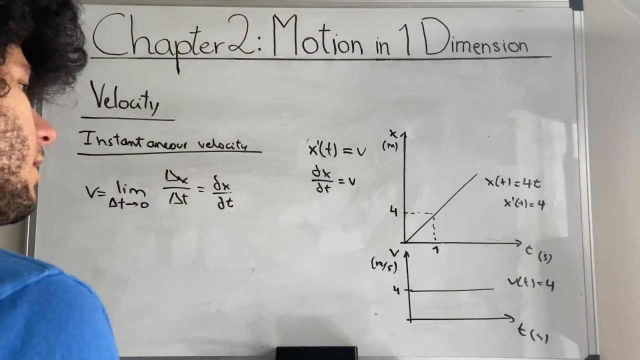 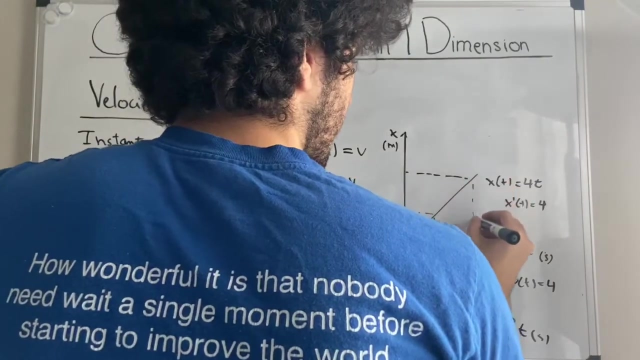 That's what that is basically saying. I don't even have to write the seconds. Every four meters, one second. No, we travel four meters every second, Four meters per second. That's the speed And it does not change at any place here. 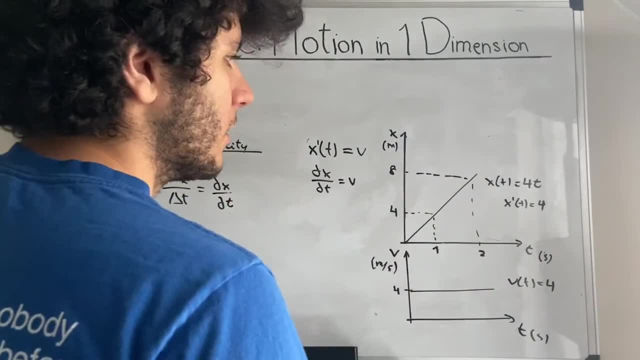 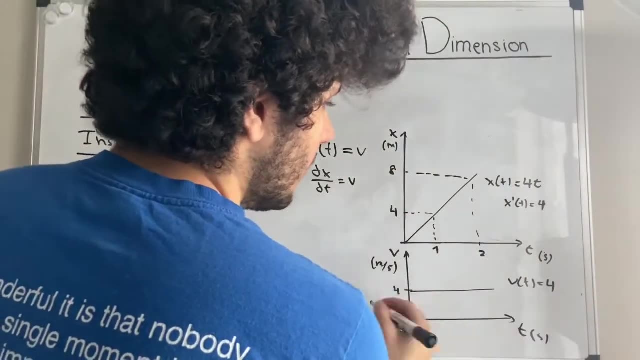 See eight to two. That's a continuous slope. The slope is always the same, no matter how far we go Basically, and that's why the here too, the slope is the same and the function is just constant. It's just always equal to four. 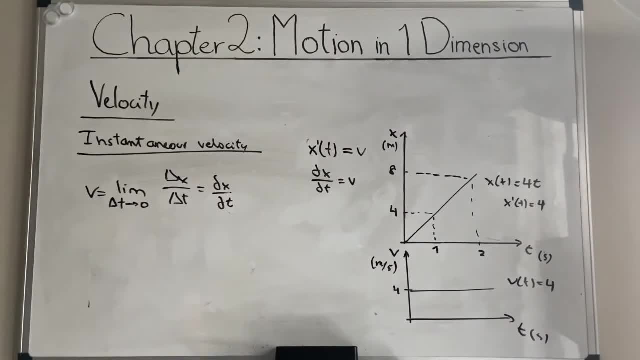 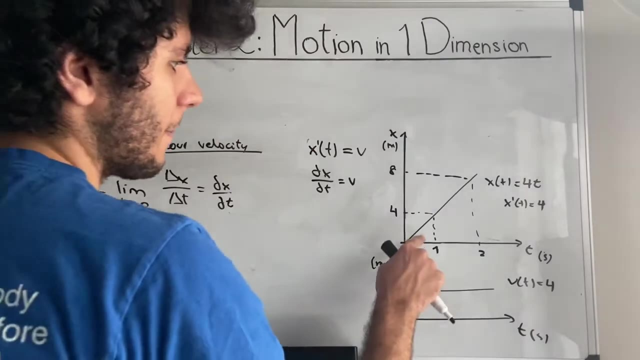 And that helps us quite a lot. It's going to that's going to come a lot in use. We're gonna use that a lot in the class. Let's think about: yes, it's worth noting that if we have positive slope, 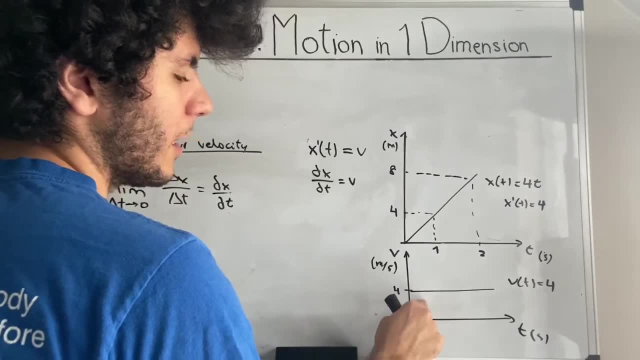 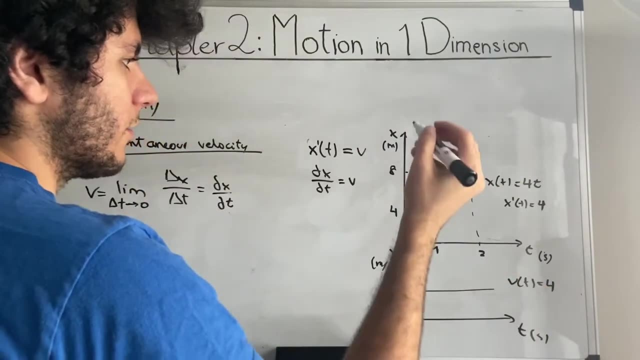 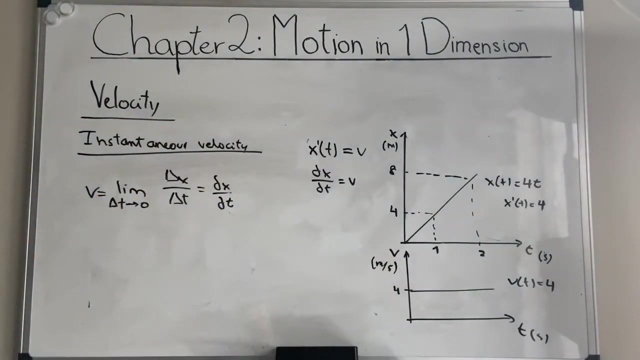 then we're gonna have a positive, a positive instantaneous velocity at any point. And if we have a negative slope, we're gonna have a negative instantaneous velocity at any point. And if we have a slope, that is constant in the X versus time. 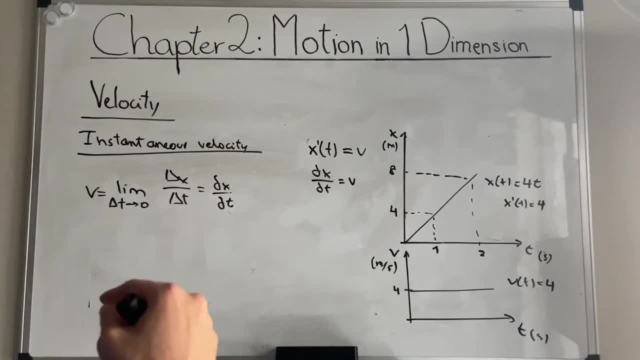 the position versus time graph, then we're going to have a slope of zero, So that's a instantaneous velocity of zero at any point along the graph Right. So that's pretty much it, And if we think about this- let's think about this a little bit- 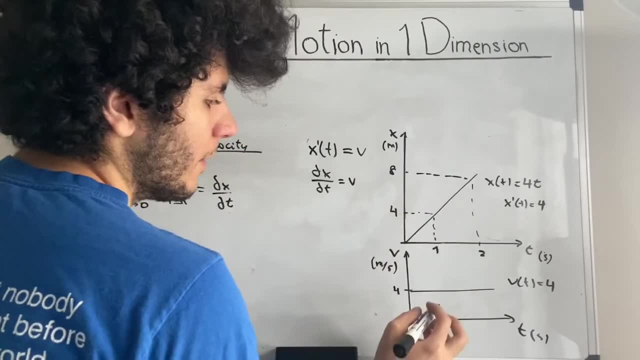 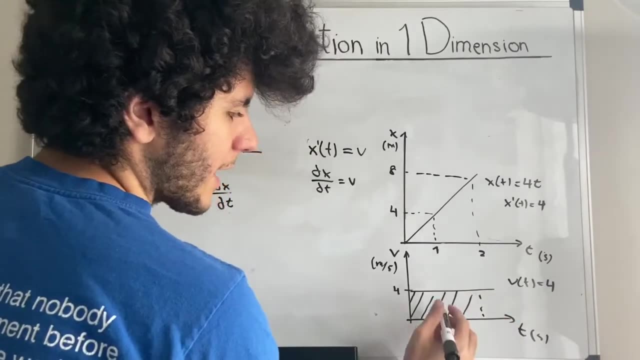 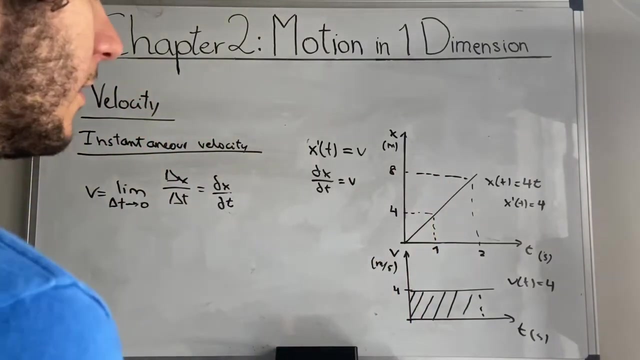 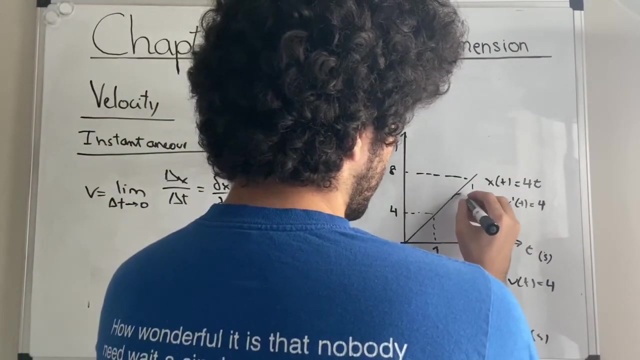 If this is the derivative of that, then the integral of this function is actually the distance covered by this function. right, And let's think about this a little bit. right, If we have, if the function were to change, change a little bit and maybe drop, like this: 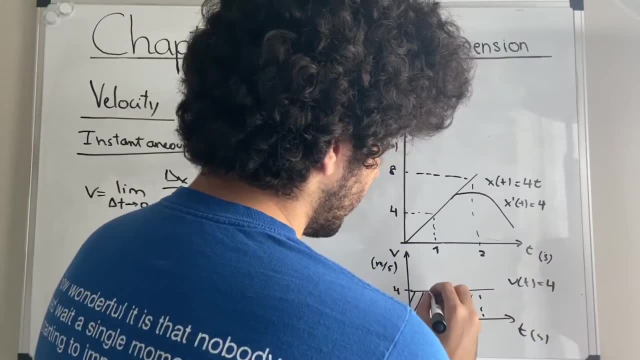 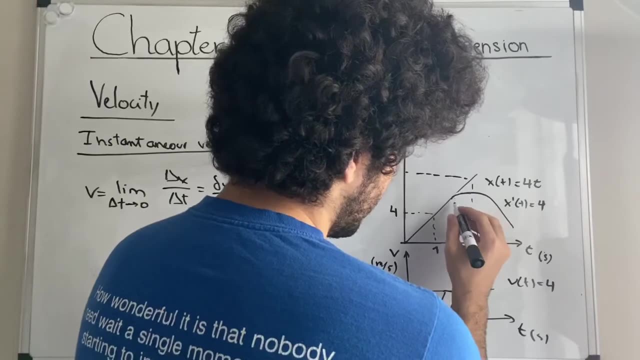 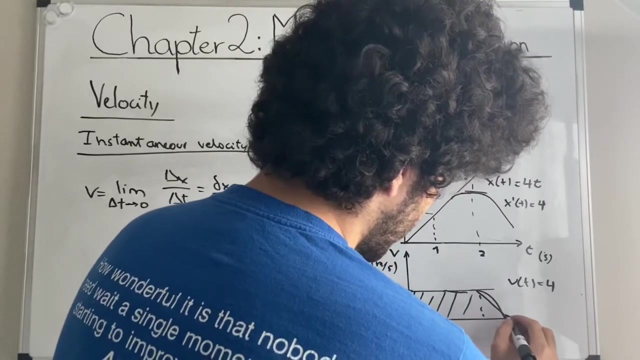 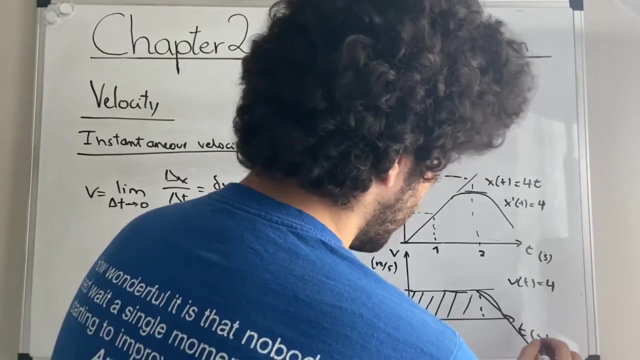 then this function would also drop right. So it's gonna continue positive And then here the slope is zero. It's gonna go like this, like that ish, And it's gonna turn out to be negative, like that Right. 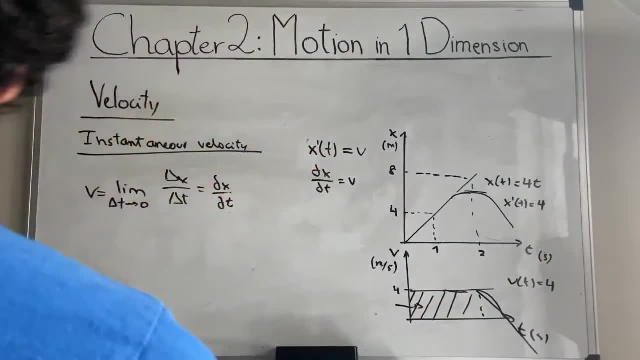 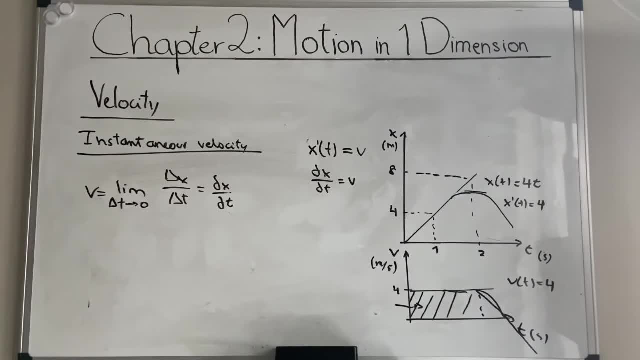 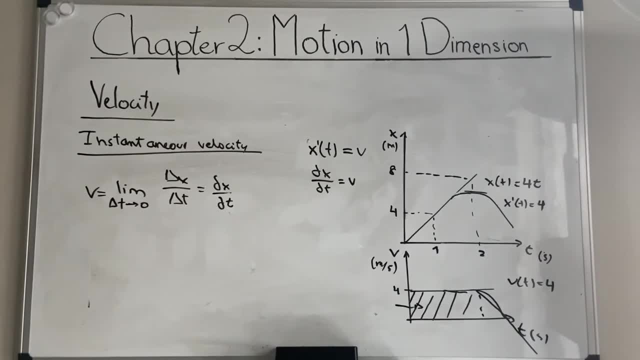 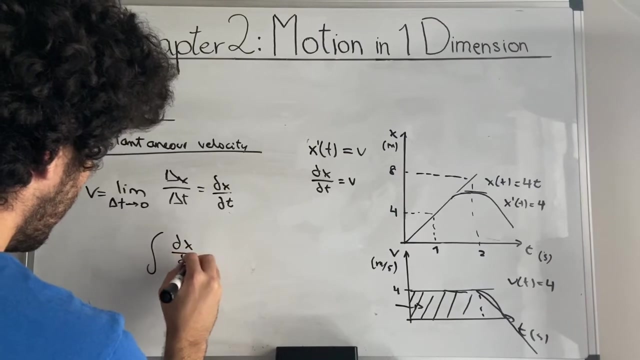 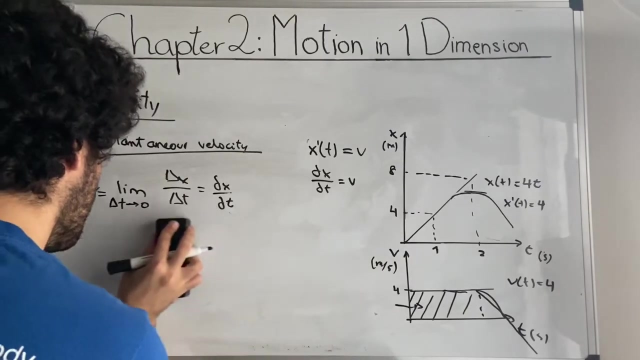 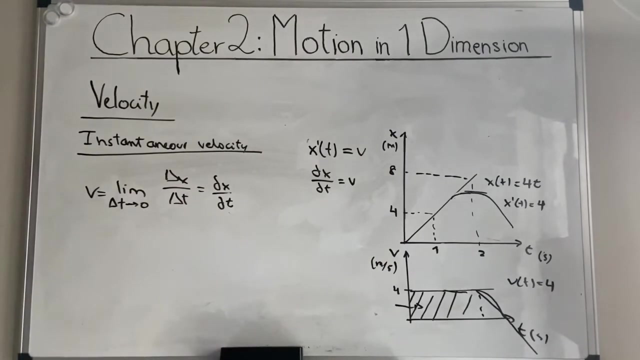 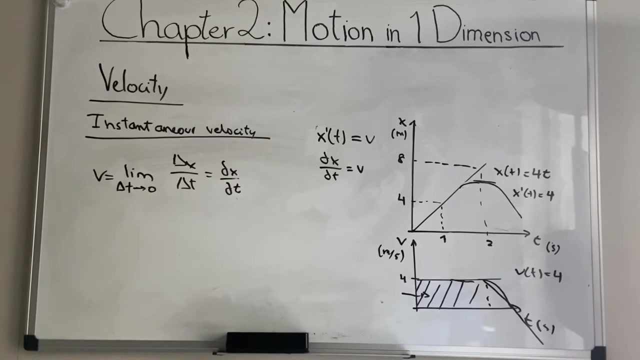 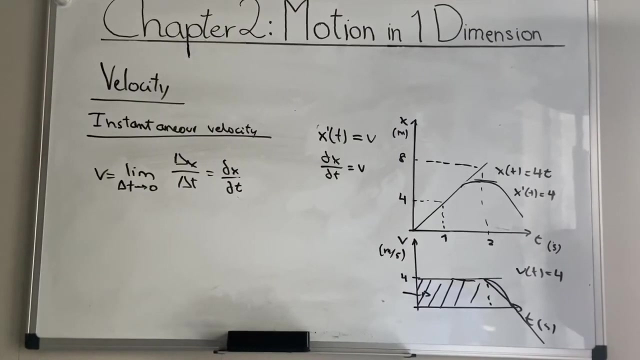 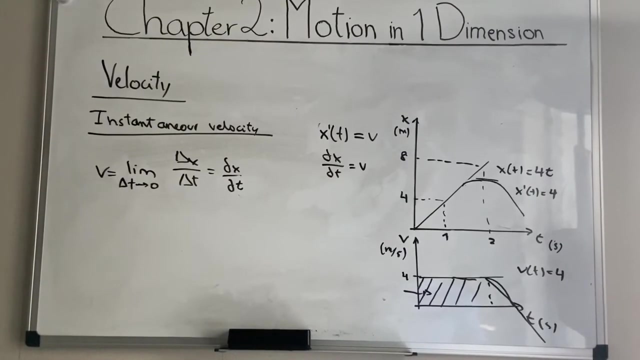 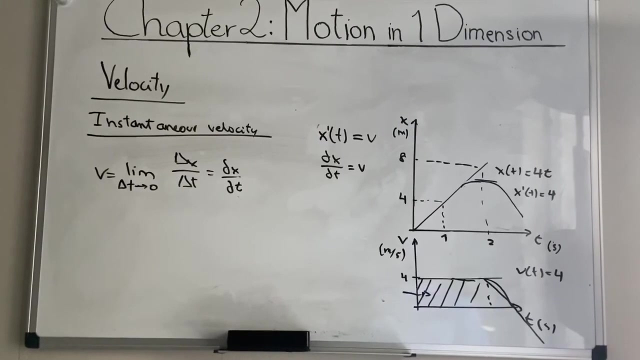 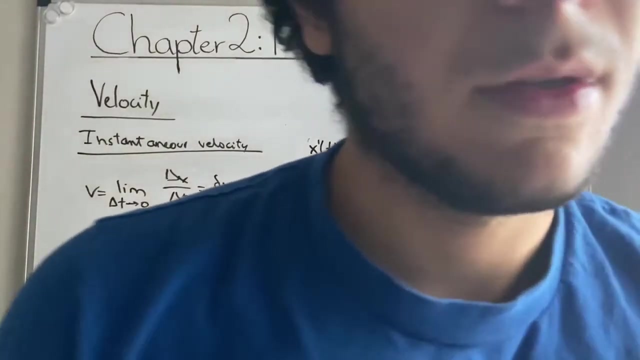 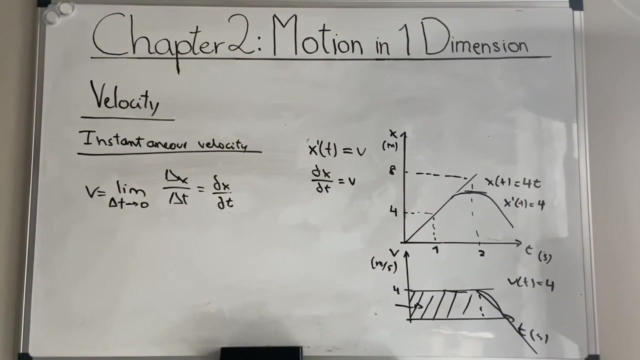 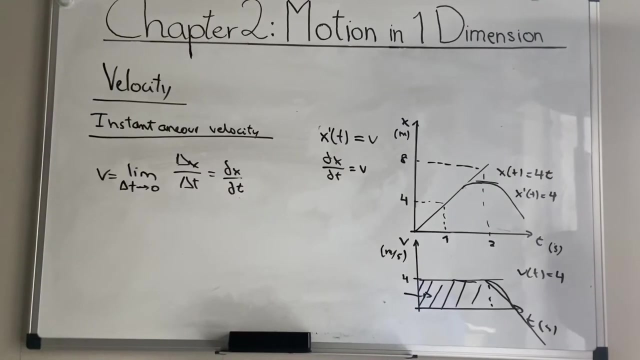 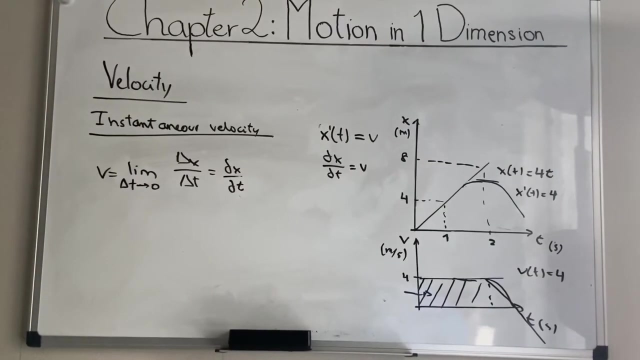 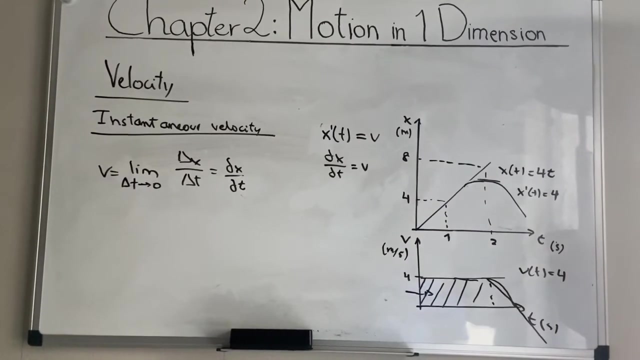 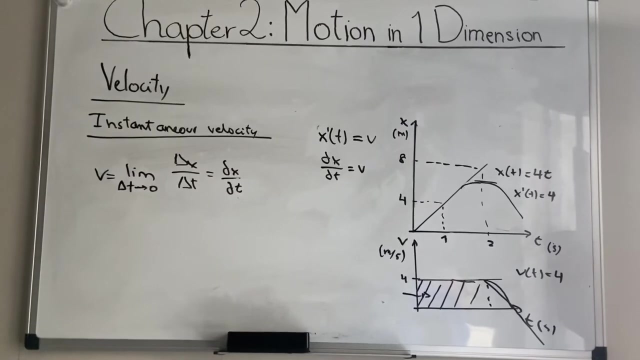 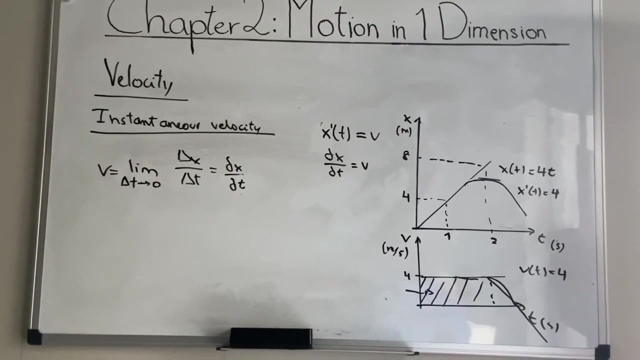 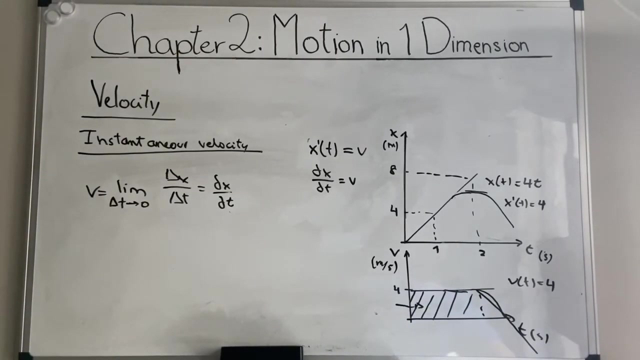 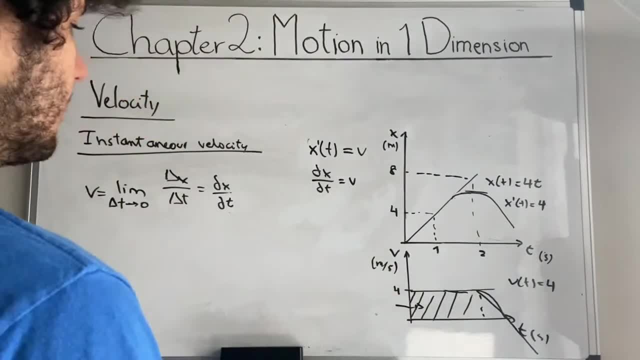 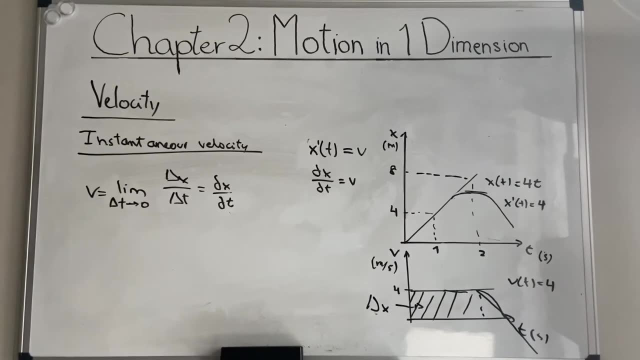 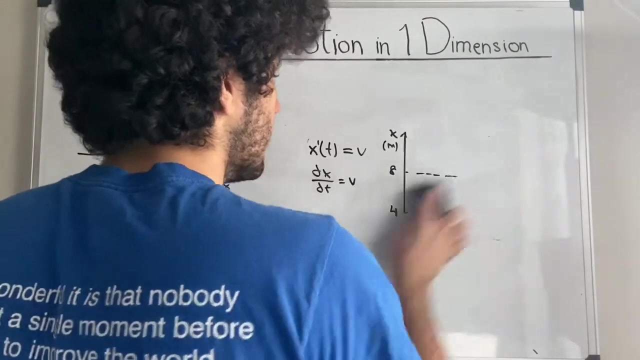 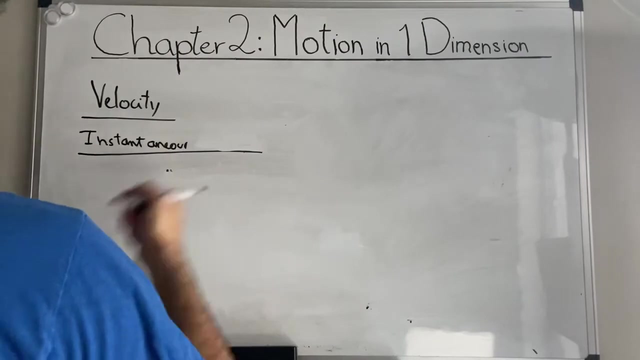 is in fact the displacement right. Okay, that's worth noting as well. Okay, next, we're going to go over quickly the instantaneous speed, which is the magnitude. instantaneous speed, All right, it is the, The definition of it is the magnitude. 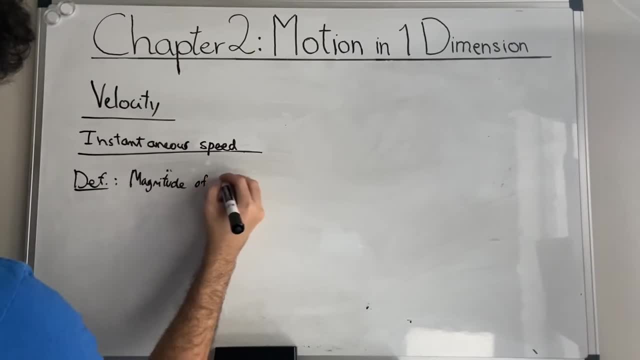 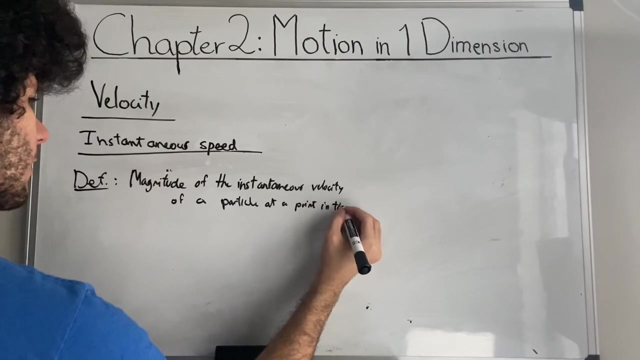 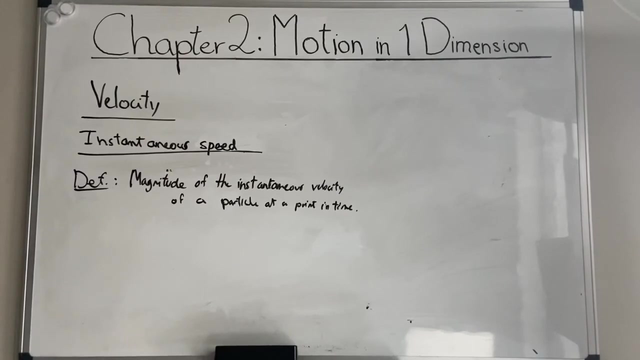 of the instantaneous velocity of a particle at a point in time, And it's gonna make a little bit more sense when we start chapter 3, but for now we're gonna have to deal with it. So basically, an example could be that. okay, so say we have a particle with negative 25 meters per 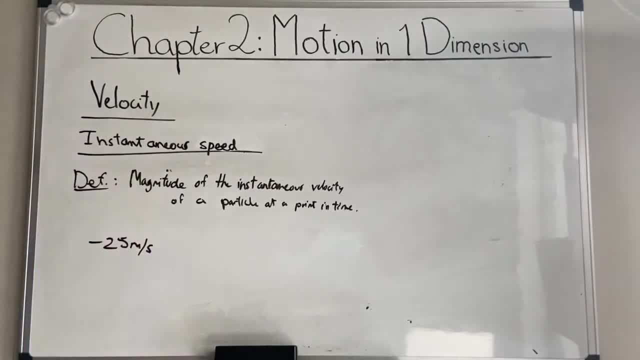 second, as a velocity, and that's possible because velocities can be negative, speeds cannot be negative. So basically, we're gonna go over this in chapter 3, but this, this is a vector, Right, It's a quantity which has a sign, and the sign is basically saying that 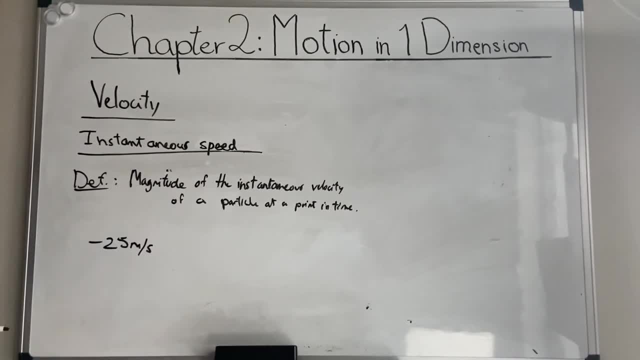 it's going in the opposite direction, the opposite negative, the opposite X direction right. So the magnitude of this is the number right, And that's the speed. That's what we're defining as magnitude. So therefore, the speed of something. 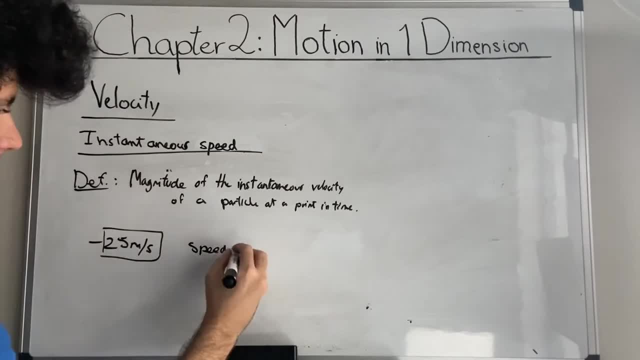 moving with a velocity of negative 25,. 25 meters per second is 25 meters per second. As simple as that. It's basically the- yeah, it's just the magnitude of the vector And we're gonna go over that very. 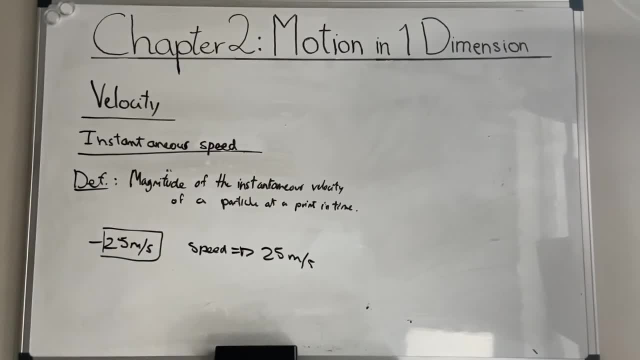 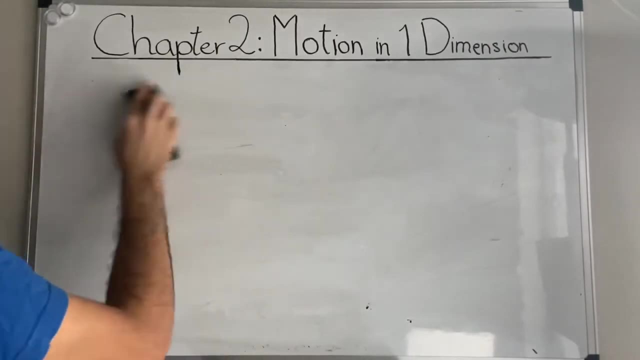 shortly it will start to make sense. Alright, now we're gonna start going over. acceleration, Okay, Acceleration, The velocity of velocity, Kind of Acceleration. Ok. so this is basically the rate of change of velocity, And just. 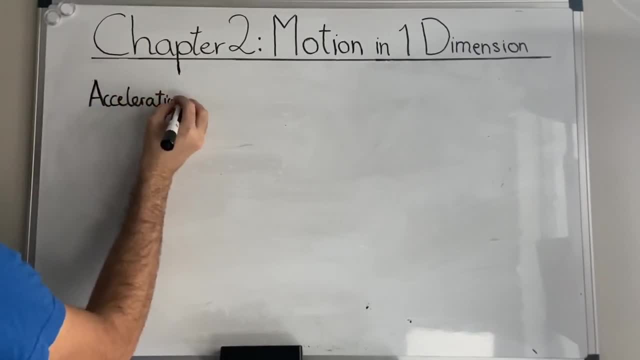 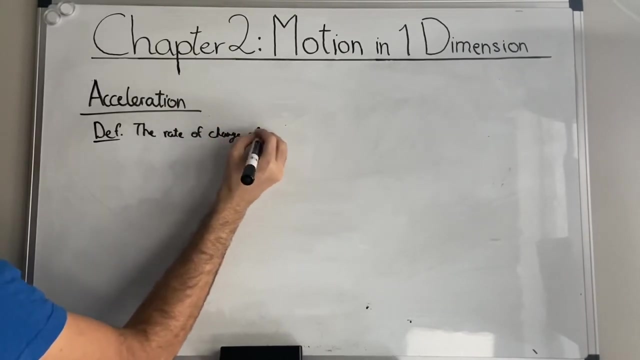 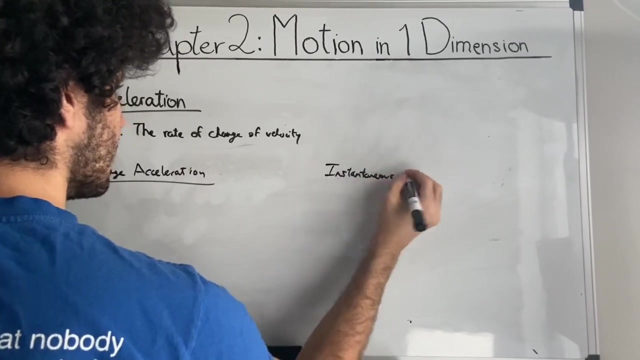 So this is basically the rate of change of velocity And just And just and just like velocity, we can define it as we can use acceleration as average acceleration. sometimes we're going to ask for that value and sometimes we're going to look for instantaneous acceleration and for the most part, is 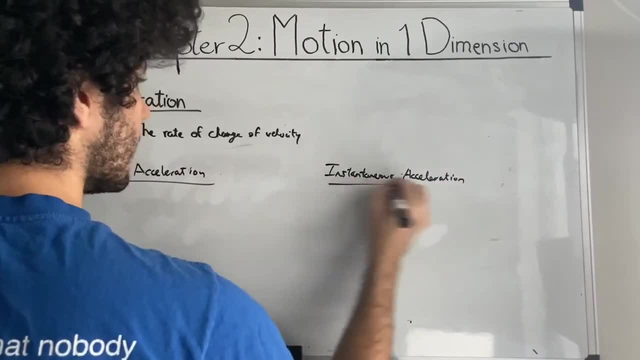 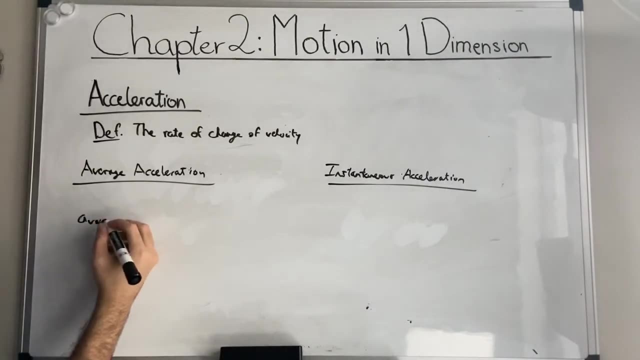 class. we're going to be dealing with constant acceleration. okay, so average acceleration, just as the other. just like the other definitions, I kind of screwed that up. just like the other definitions of like. just like the other. average, just like the other. just like the average velocity is the Delta V. 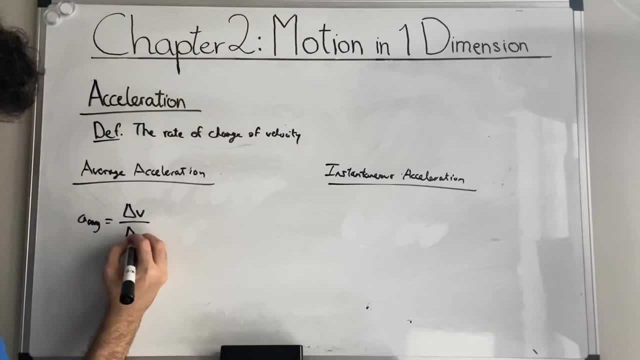 Delta velocity: change in velocity over the change in time, over that, yeah, exactly, so that's pretty much it. it's rather simple. you, the units of acceleration are meters per square, meters per second squared, and so, yeah, we, just as we did before, we can interpret average acceleration as like: 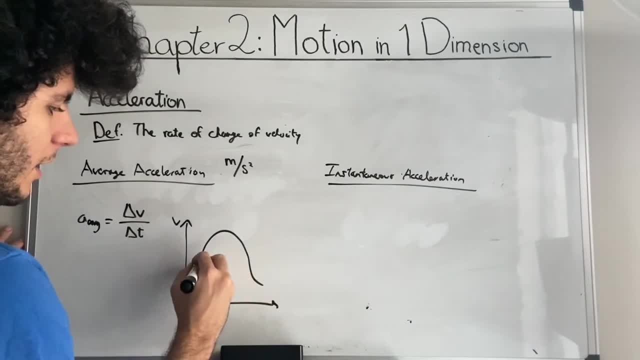 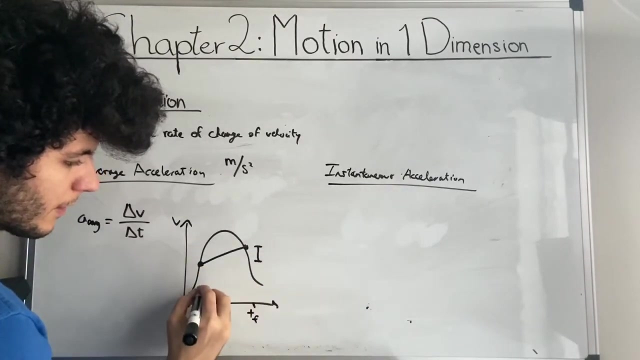 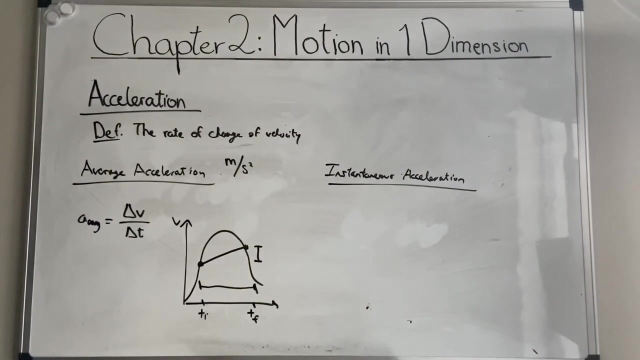 if we have a graph like this, it's cutting the graph to connect two dots, this being TI, this being TF, right, and then we end up with a change of velocity and a change of no. no, I have them last night. it's okay, I have them last night. thank you, mom. 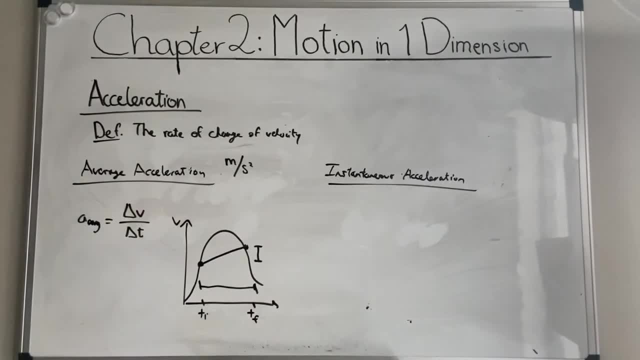 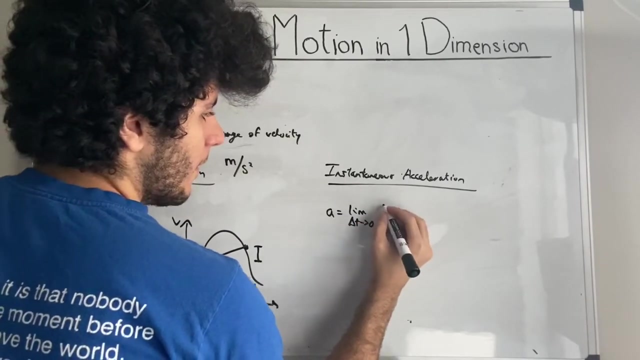 and a change, a change of, uh yeah. so basically it's the change of velocity over the change of time, right time. We can also define acceleration as instantaneous acceleration, in which circumstances we would be taking the limit of delta t heading towards zero, of delta v over delta t, which gives 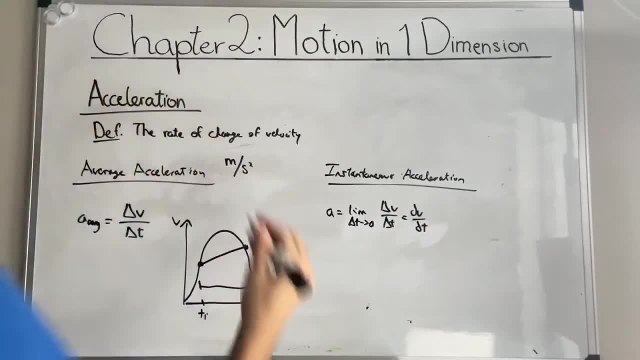 us delta, v, dv over dt, something that we can familiarize ourselves with if we've taken calculus, And now we are going to be dealing with a slightly- I would say- weirdwe're going to have to create new intuition, And let me explain what I mean by that: Acceleration. 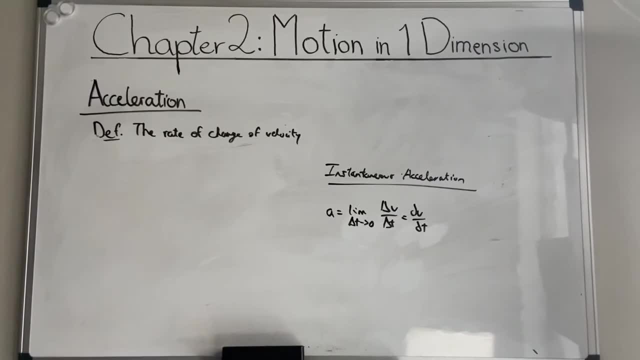 is the rate at which velocity changes. If we say something is accelerating, it means that velocity, the change of velocity, is positive. right, that means that we are well, actually there. there's positive acceleration when the velocity increases with time, when the velocity increases with the T, and then there's negative a. 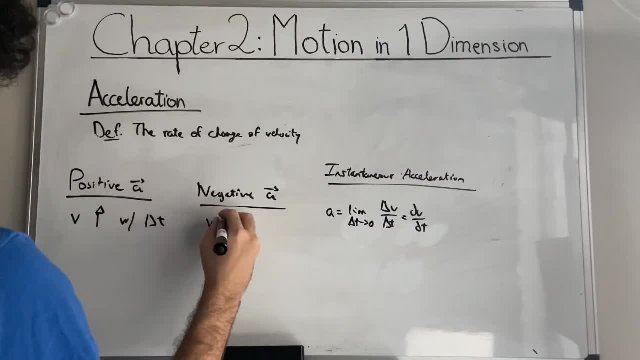 when V decreases with delta, T, T right, and so the acceleration of an object is positive if its direction is the same as that of the direction of the motion of the object. all right, not nice. I'm a little bit difficult to digest, but let me phrase it in a different way. 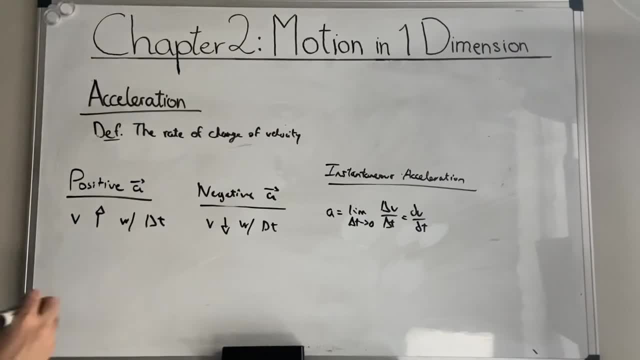 basically, we have a car driving and it's moving in this direction. this is its motion, and if the acceleration is in the opposite direction, then this is called. this is negative acceleration. the acceleration is caused by the acceleration of, the is causing the car to reduce its speed, Reducing its speed with respect to time. 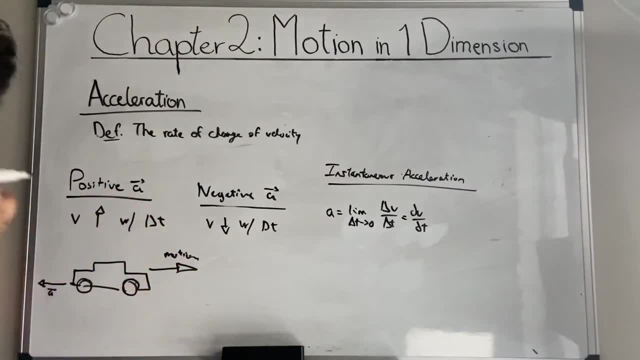 Therefore, this is deceleration Negative. If the acceleration is pointing in the same direction as the motion, well then the car will be accelerating right, And that's pretty much it, Even if the car would be backing up, as long as the acceleration and the motion are in the same direction. that 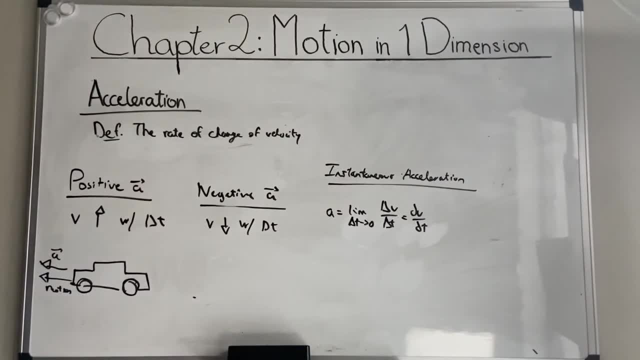 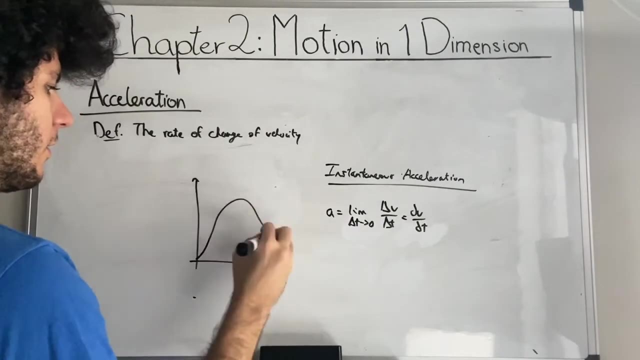 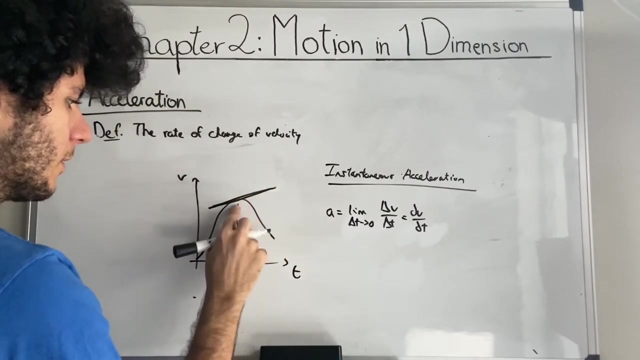 would be considered positive acceleration, And that also depends on the coordinate system that we're working with, of course. And so, going back to instantaneous acceleration, if we have a graph of v over t, taking the tangent at a point, at a point can help us. 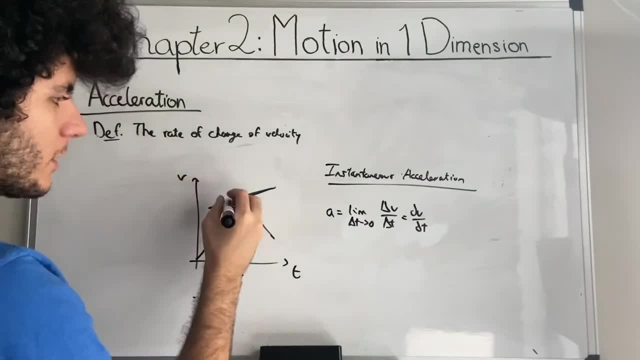 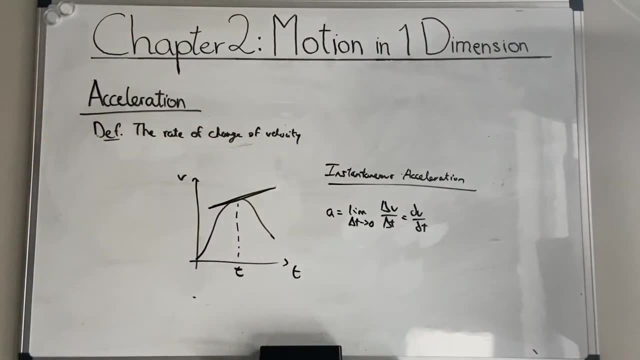 taking the tangent of a point will show us the slope of that point, and that slope is the instantaneous acceleration, And that's pretty much it. Just as dv over dt, just as dx over dt is velocity, we have dv over dt, which is acceleration. 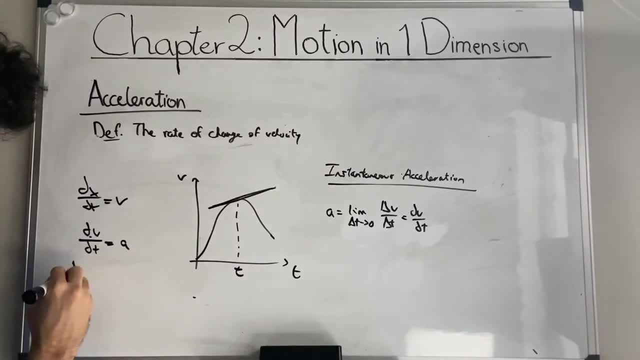 And thus we can. we know that d, the double derivative of position with respect to t, is equal to the derivative of velocity with respect to t, which is equal to a acceleration. There we go, And now we're finally gonna make our way. 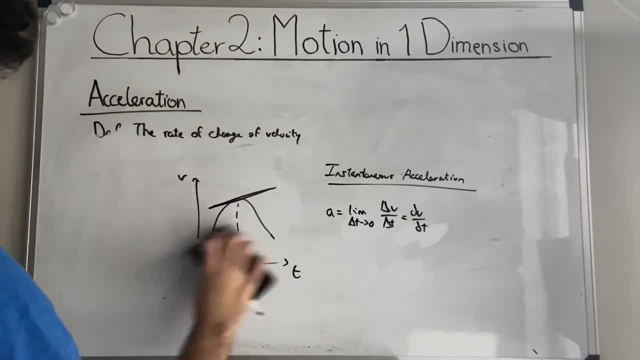 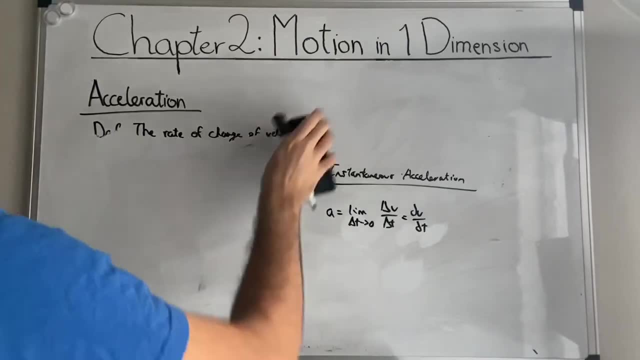 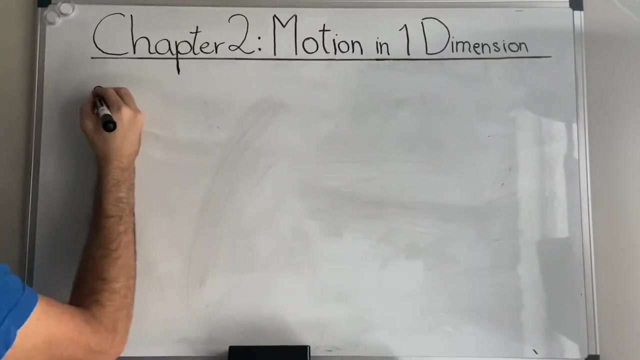 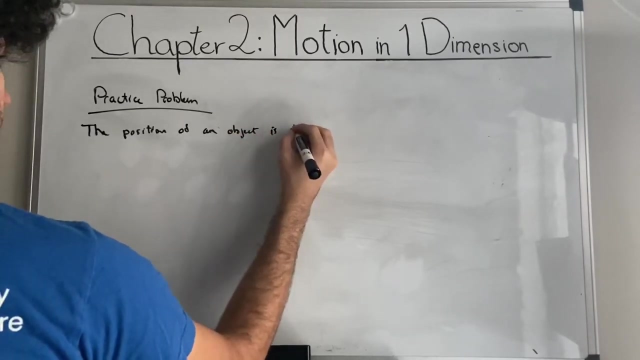 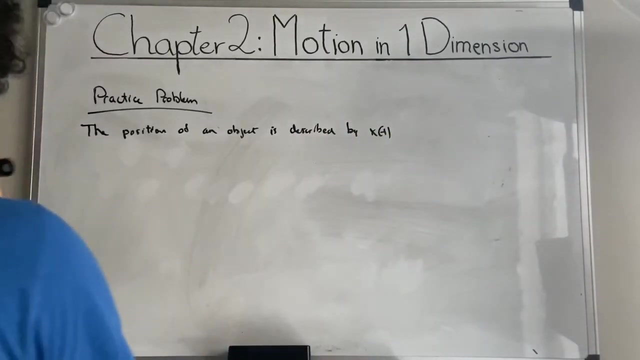 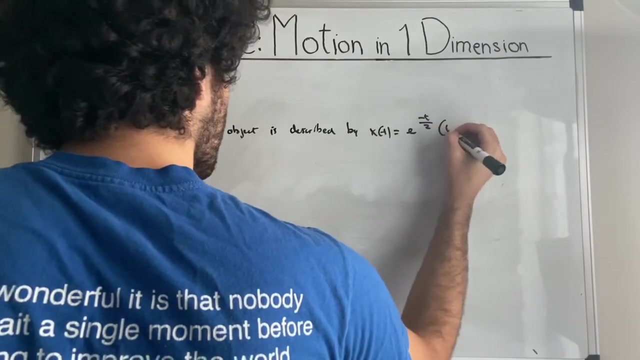 to some practice problems. All right, Finally, just further our understanding of acceleration. Just make sure that we really understand what is going on. A practice problem: The position of an object is described by X of t is equal to e. I've got a little function over here, minus two t. 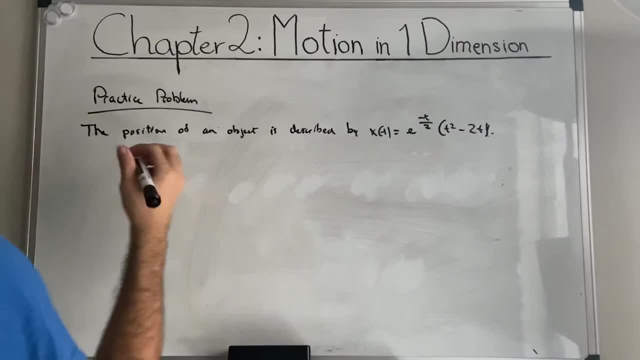 Minus two t. okay, When is the velocity zero? Okay, So the position of an object is described by that function. When is the velocity zero? So that's a little bit. it feels a little bit tricky, The velocity, we only have the position function. 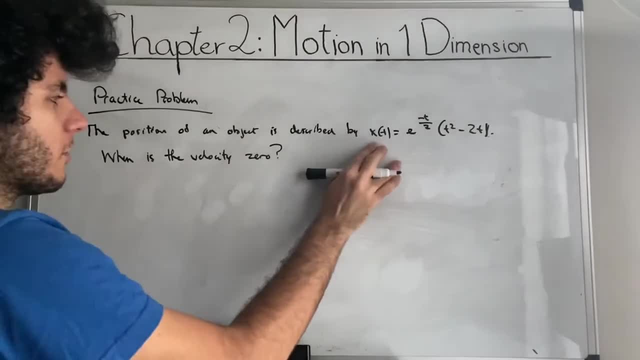 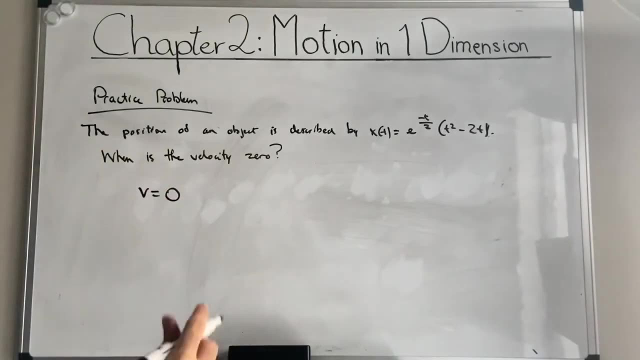 What relationship do we have between the position function and the velocity function that can help us find out when v is equal to zero? Well, we should know that dx over dt is equal to v. Therefore, if we find the derivative of this, 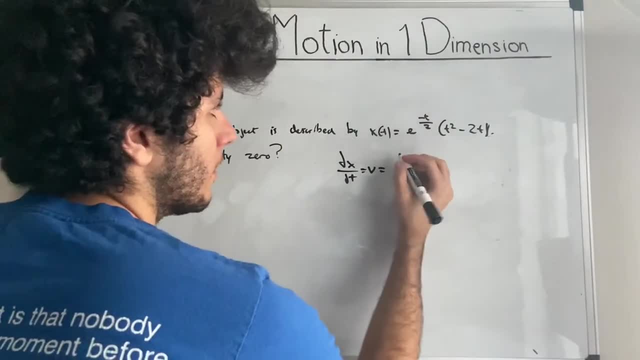 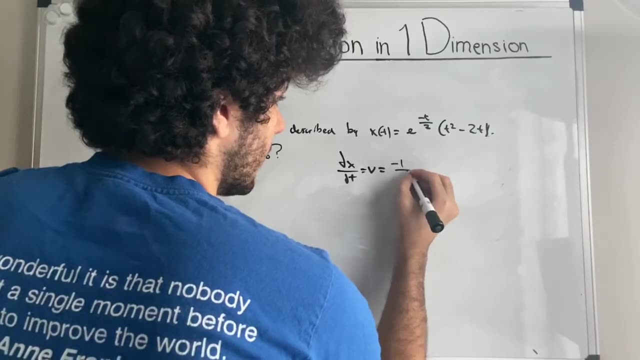 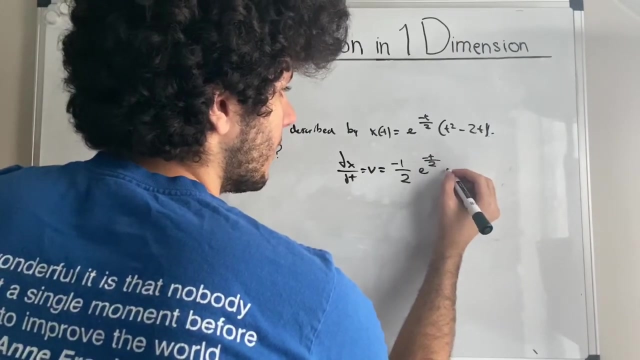 we can find the answer. So we go ahead and do that. So we are going to be doing the product rule. So negative, add e to the negative. two over t. over t times t. I'm worried of losing the space. 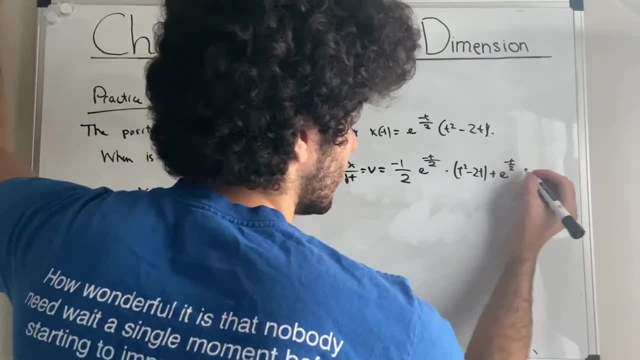 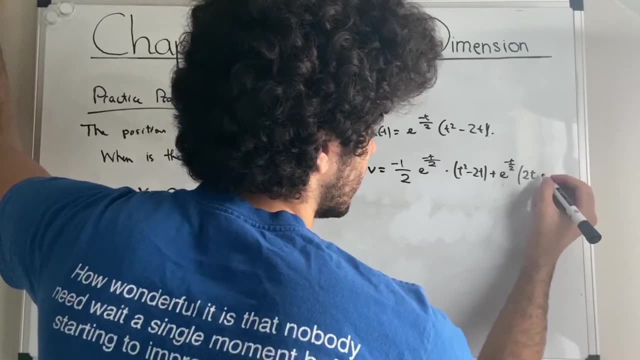 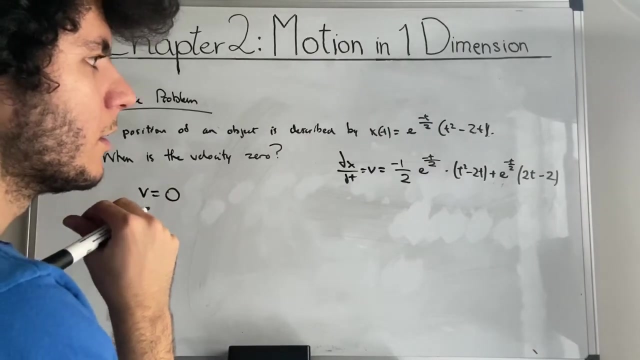 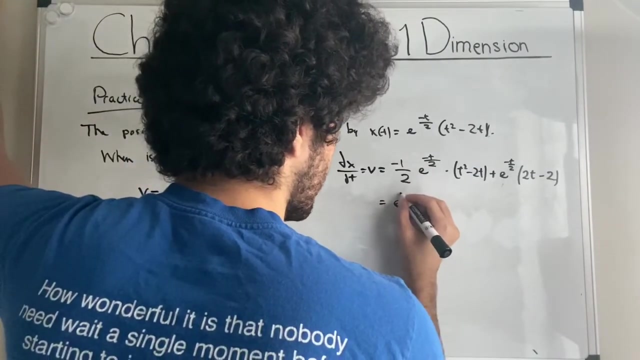 plus e to the negative t over two plus, not plus times two, t minus two. Okay, Right, Is that everything? Yeah, I think that is So, then we do we. we can simplify this Is: 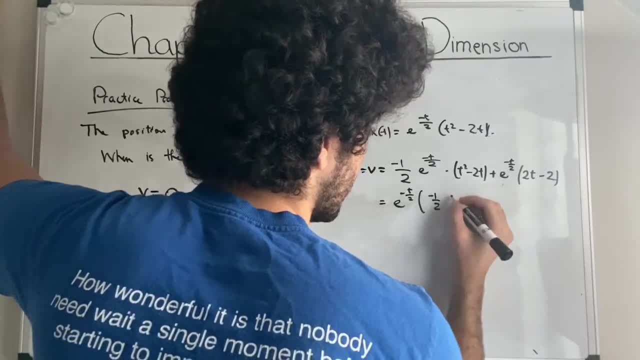 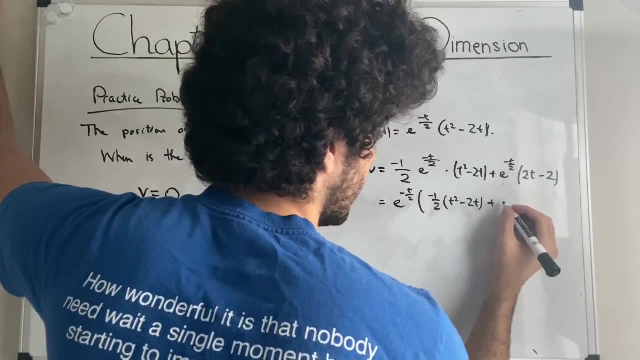 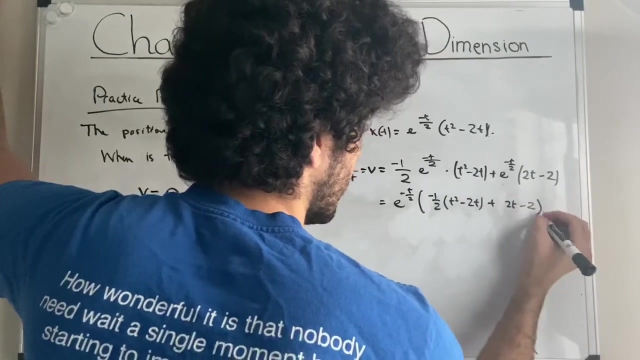 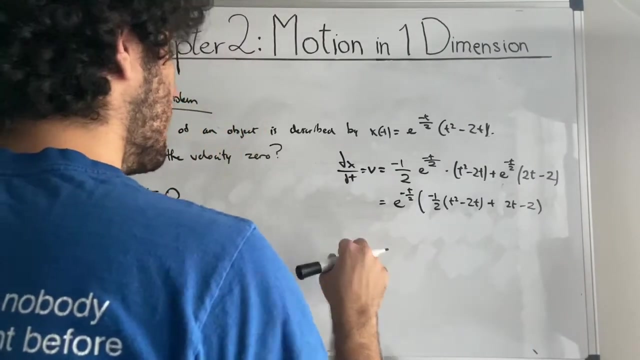 Okay, Okay, Let's let me just submit that. Yeah, I was just thinking for a second. Yeah, we don't okay, so Here, so we have the. we haven't fully finished simplifying, but we have to come to a certain understanding. 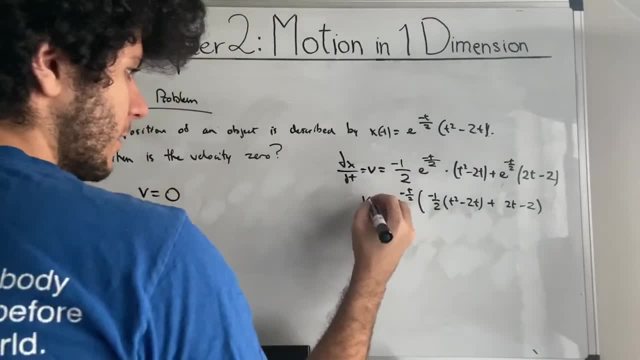 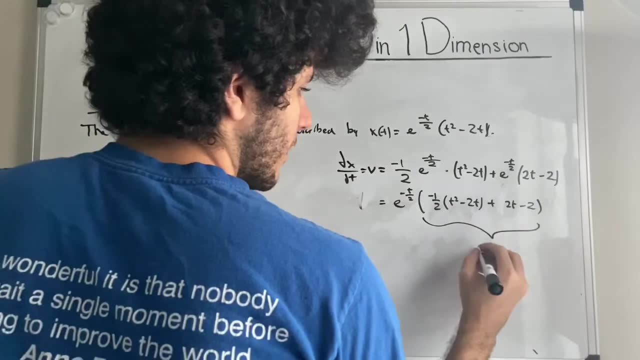 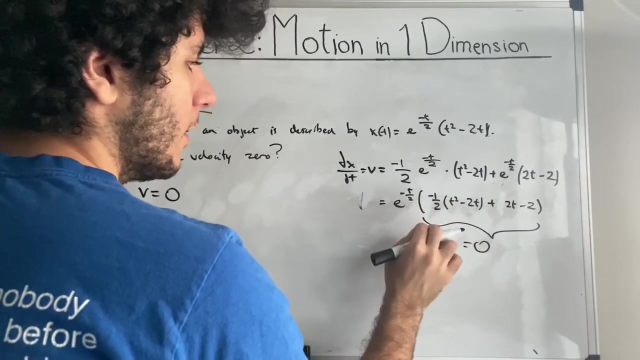 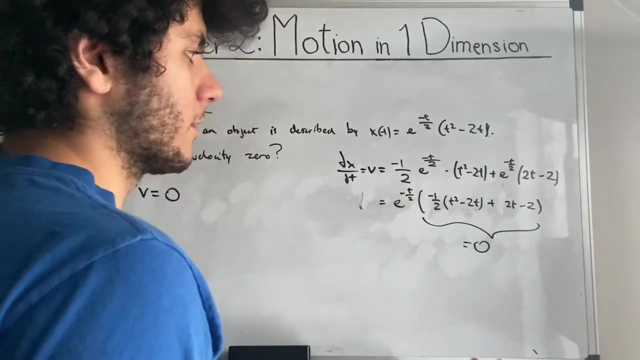 We're trying to find the moment when this is equal to zero. This will be equal to zero Only if this part is equal to zero, because this will never be equal to zero, And a multiplication will only be equal to zero if one side, one of the parts of the multiplication, is equal to 0. 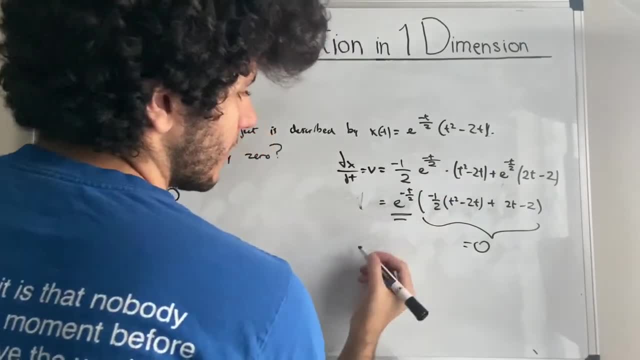 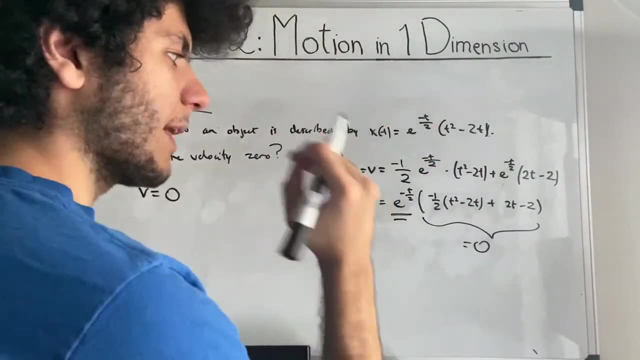 And this cannot be equal to 0, as it is an exponent e to the, something will never be equal to 0, the smallest It can become as very close to 0,, but never flat out 0. So here we can just single this out. 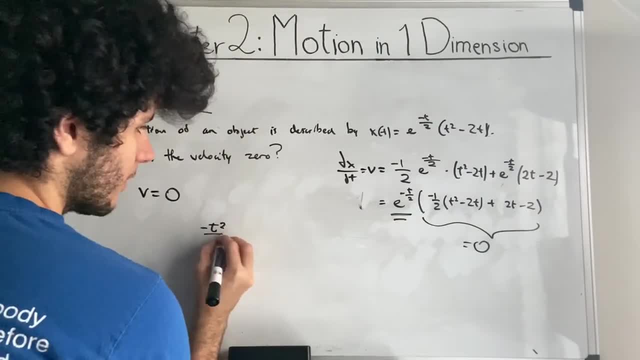 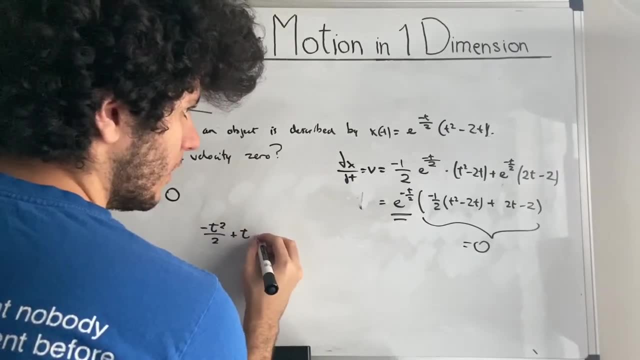 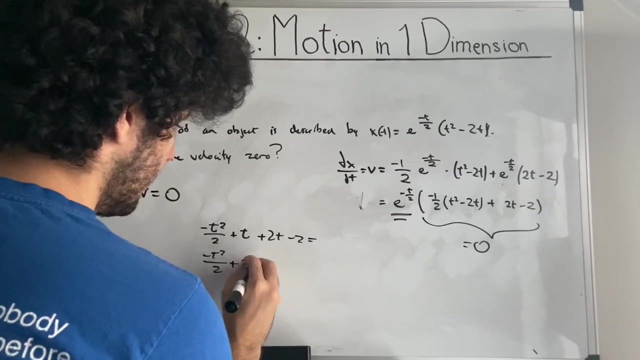 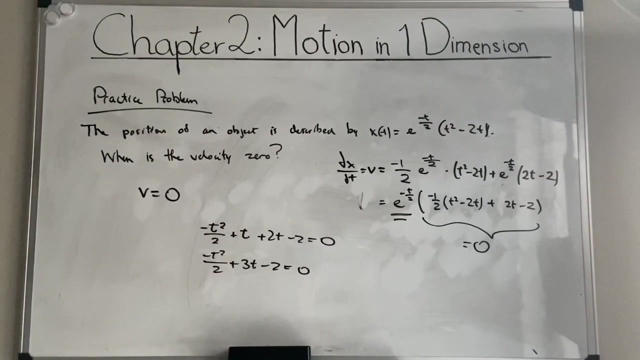 and simplify while we're at it: 2 minus plus t plus 2t minus 2 is equal to negative. t over 2 plus 3t minus 2 is equal to 0.. And now we use the quadratic equation to find our final times. 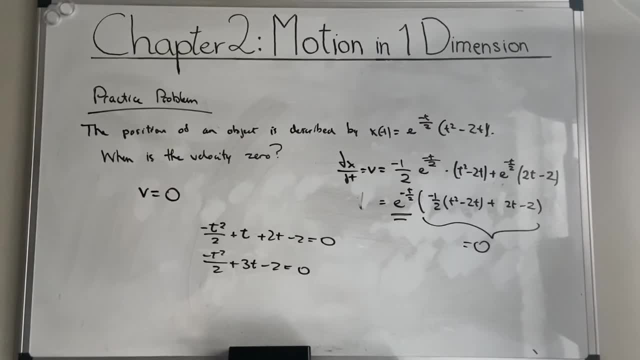 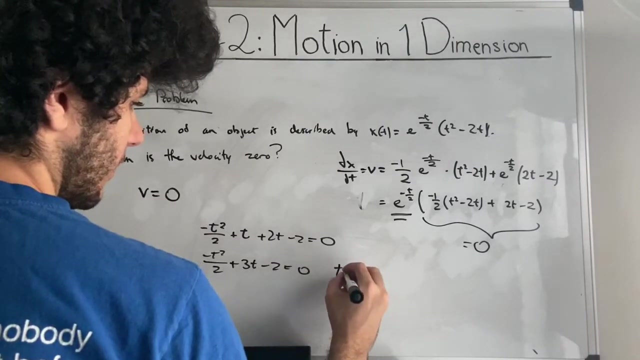 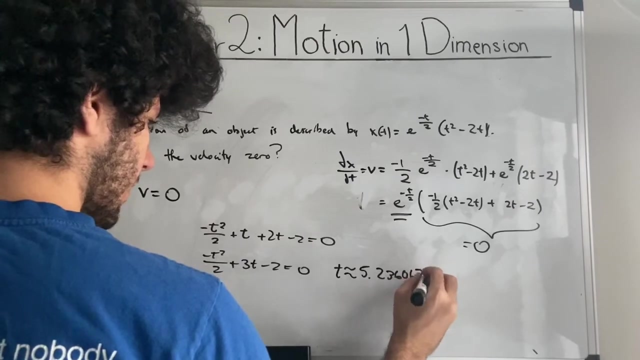 I'm going to use my calculator: Negative 1 divided by 2, negative 1 half 3, negative 2.. And we get an answer of: we obtain 2, we get 2 answers. actually, t is about equal to 5.2360679,. we'll trim the last few decimals. 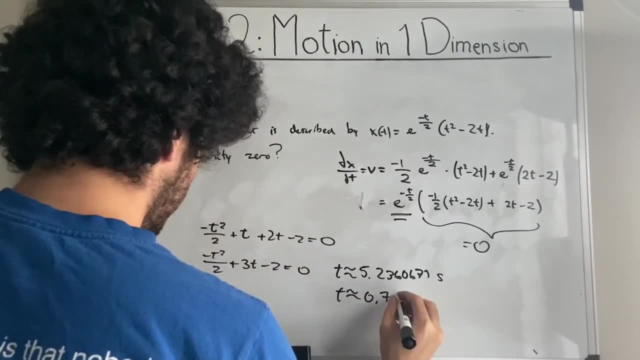 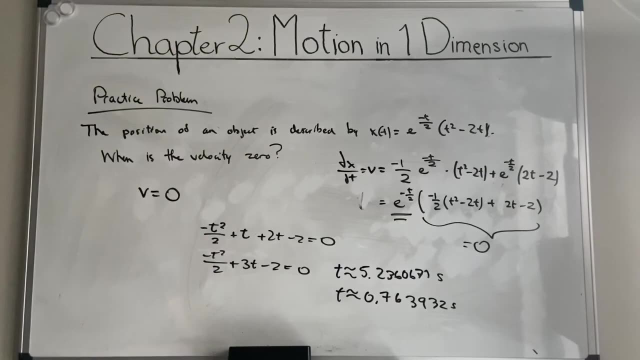 Or 0.7, and this is in seconds: 0.763932 seconds. Okay, But now what do we do? Hmm, This is interesting. We have two results. Is one correct Or is the other correct? No, Actually, both are correct. 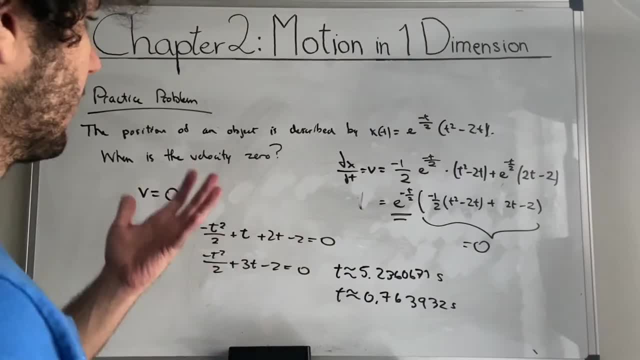 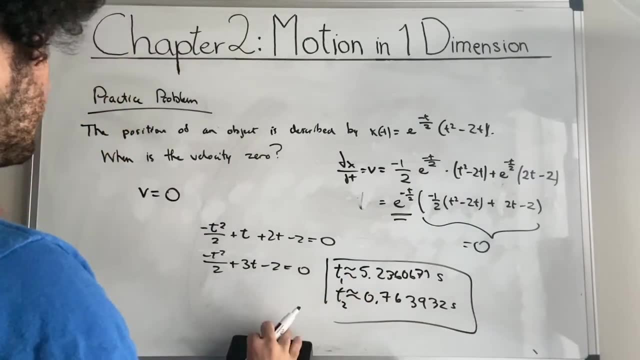 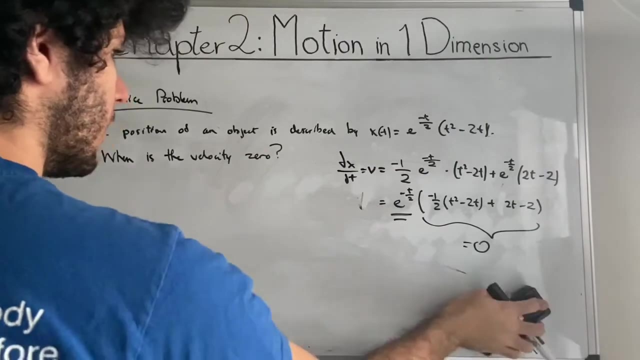 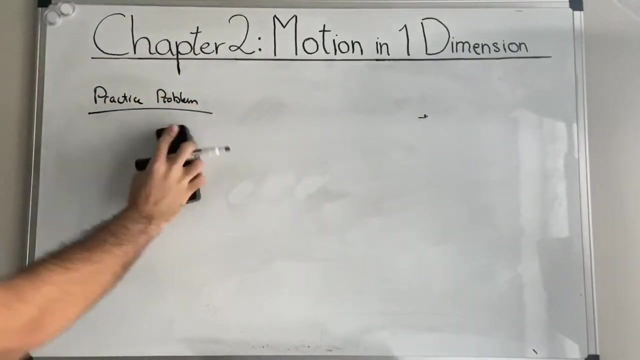 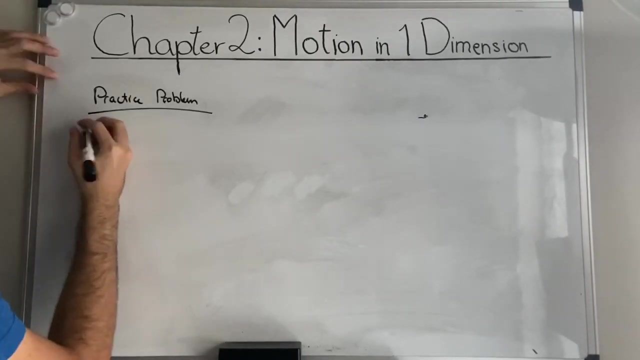 These are two times during which the velocity will be equal to 0. So we find our answer Both of these: t1 and t2.. All right, Let's go on to the next question. Okay, This question is asking saying that the velocity, the velocity of a particle, 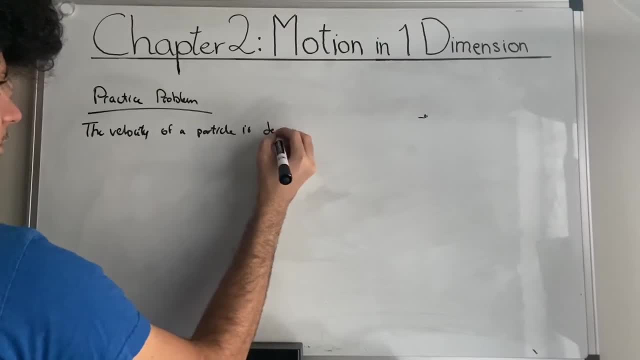 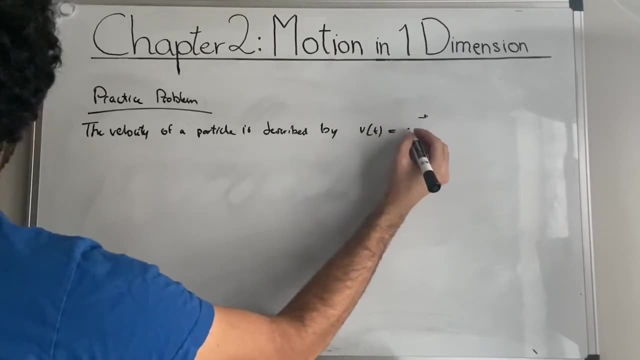 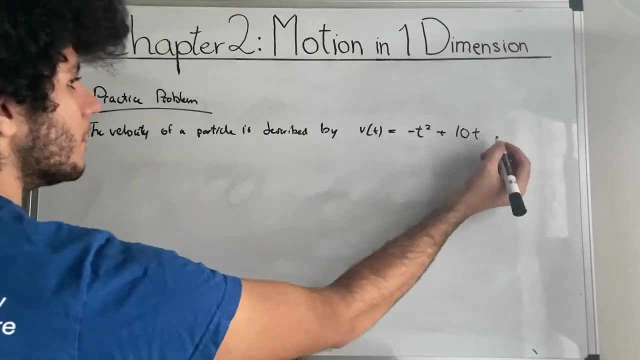 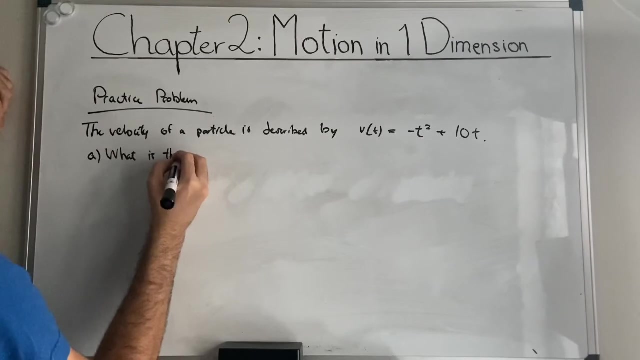 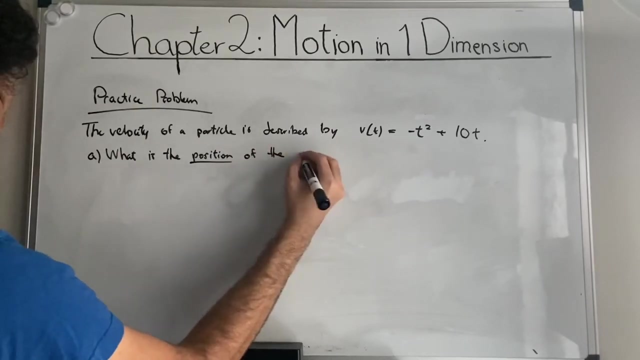 is described by v of t. the velocity function is equal to negative t squared plus 10t period. Question A is asking what is the position of the velocity of a particle at t is equal to 12 seconds? Well, hmm, what can we do here? 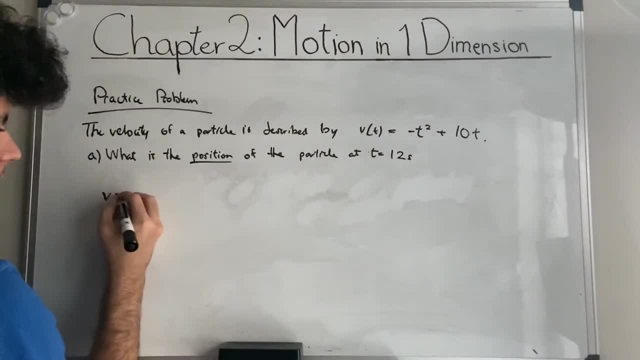 We know that the velocity is the derivative of x with respect to t right, Or at least the instantaneous velocity, And that's what is described in that equation. But what is? how can we do this? How can we find the position from that point? 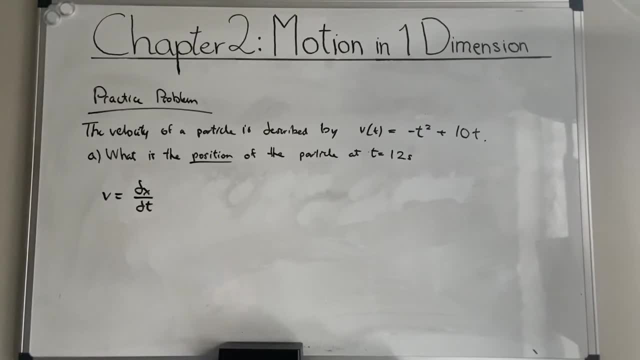 Well, if you think about it for a little, the displacement of a- I'm sorry, the displacement of the displacement of a situation, or like an object, with respect to time is equal, or just like the displacement in a given situation is equal to the integral. 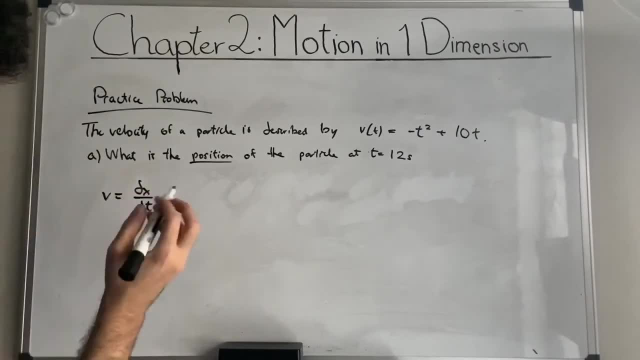 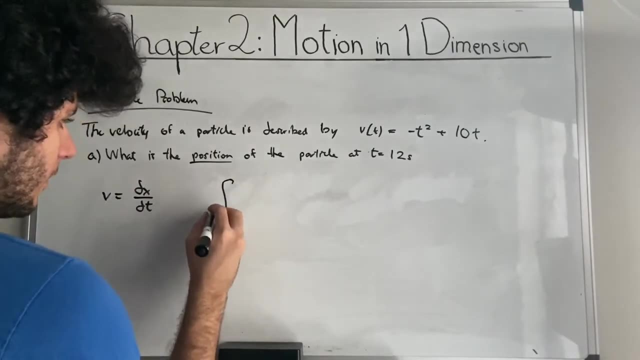 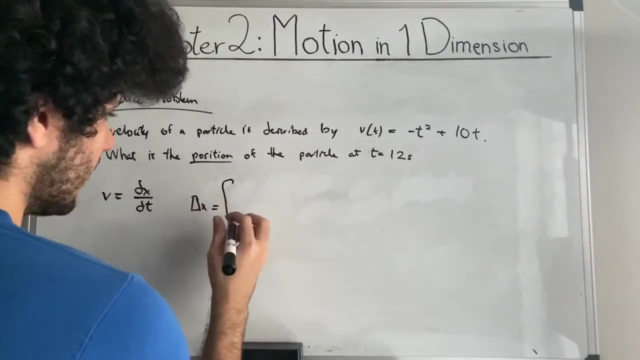 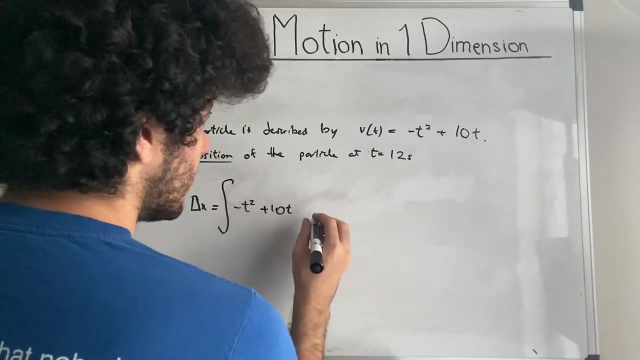 of the function of the velocity. So that's all we have to do. We just find the integral described by. okay, We basically find the integral of that negative 2 squared plus to the t. is this correct? Yeah, this is correct. 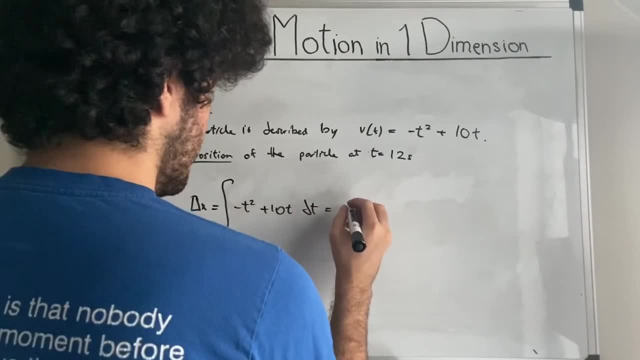 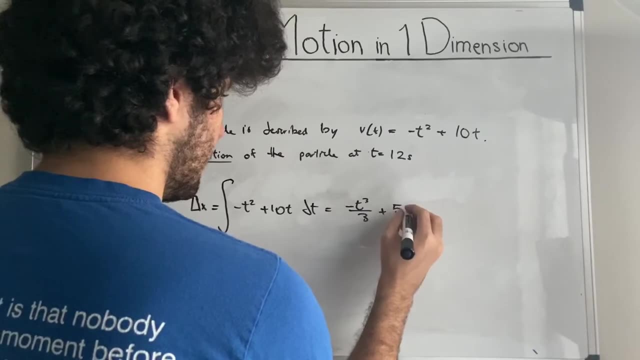 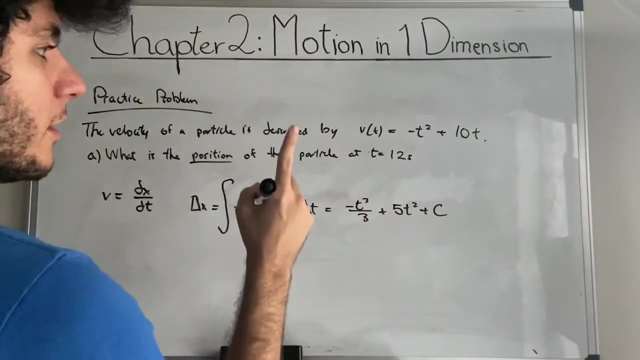 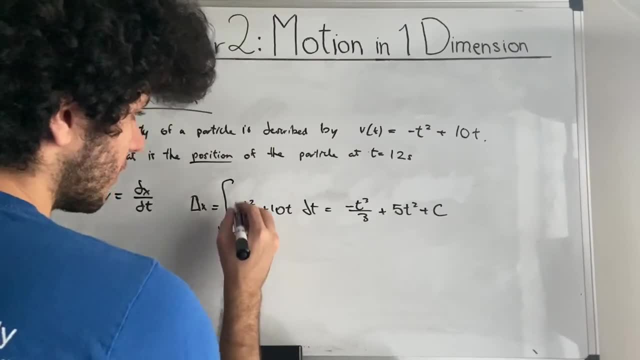 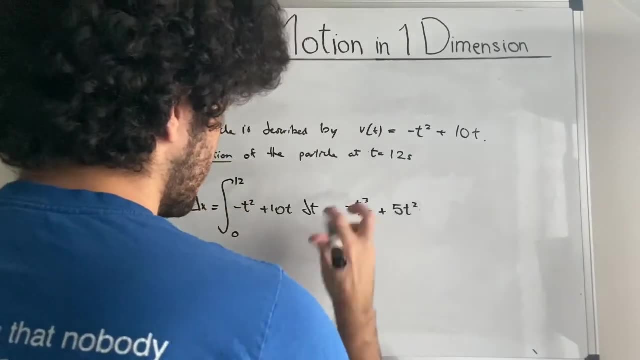 And I'm sorry it's. you can only find, you find the displacement if you mention the limits of integration. Okay, Okay, 0 through 12. so this would not be the answer. this would only be part of the answer. there would be no. 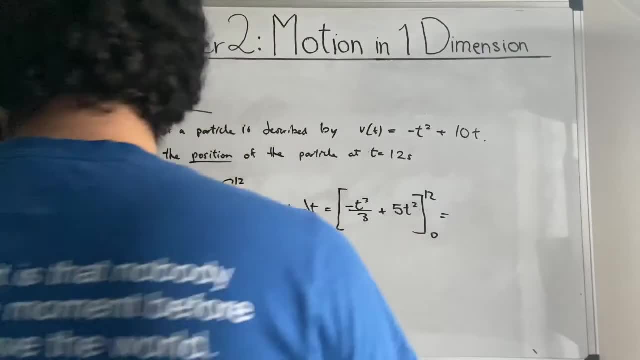 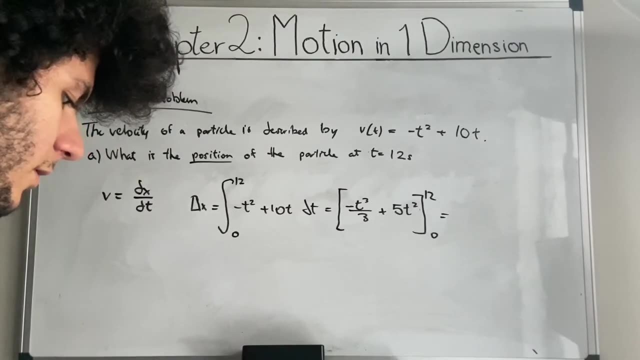 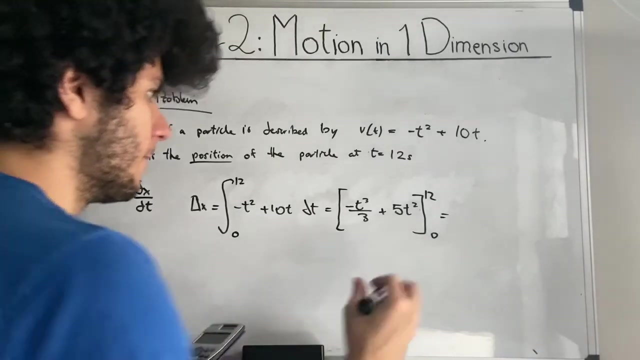 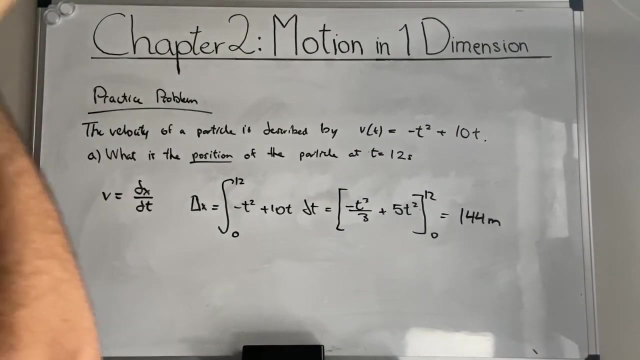 c we have. we're actually going to input this in a calculator, because 12 to the 3 is not a very easy calculation. 12 to the 3 divided by 3- okay, plus 5 times 12 squared equals to 144 meters, which is great. it is worth noting that if you just took the derivative, 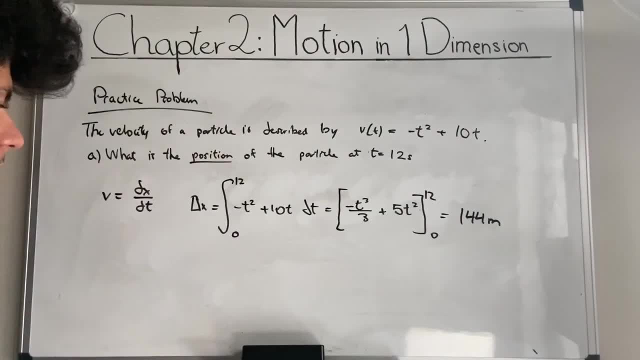 the indefinite integral. with the indefinite integral, you would obtain just the function of the position, whereas if you take the definite integral, you obtain the displacement of, like this, the situation right. and so here, by doing the definite integral, we obtain the displacement, which is all we needed, because we just want to find out the end point. we want to find out like: 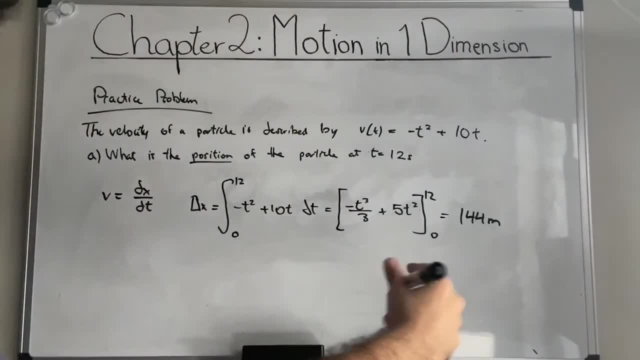 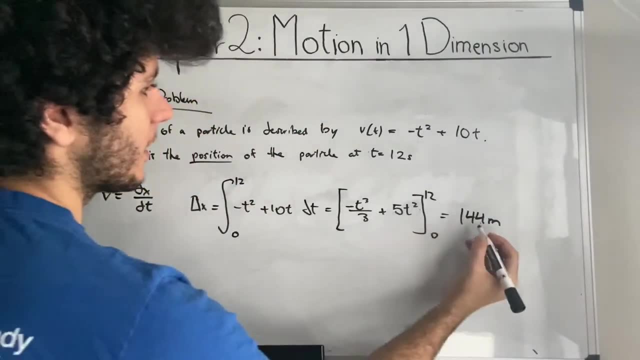 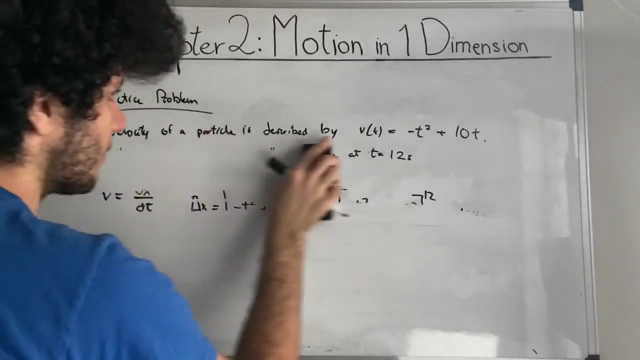 what's the the result of all the zigzags? we don't care about the zigzags, we care about the beginning and the end, and this tells us that after 12 seconds we are at 144 meters. now let's move on to question two, question part b of this question. 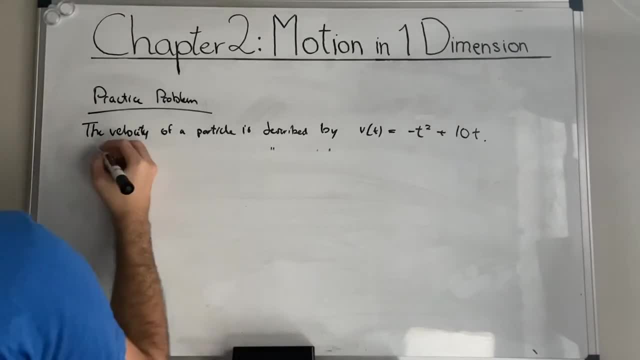 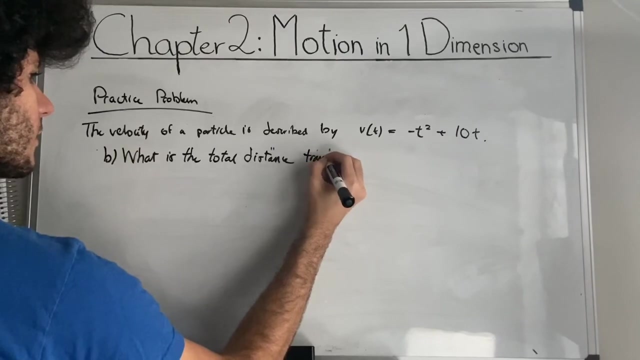 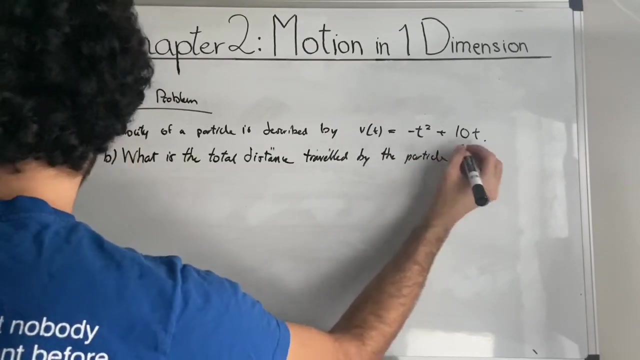 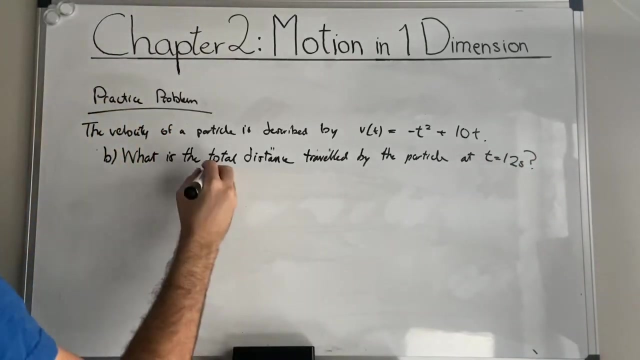 i believe it's asking for speed. the total distance, yeah, and that's correct. that is the question: what is the total distance traveled by the particle? and ty at t is equal to 12 seconds. well, total distance is not displacement. let's again remember that distance is not equal to displacement. 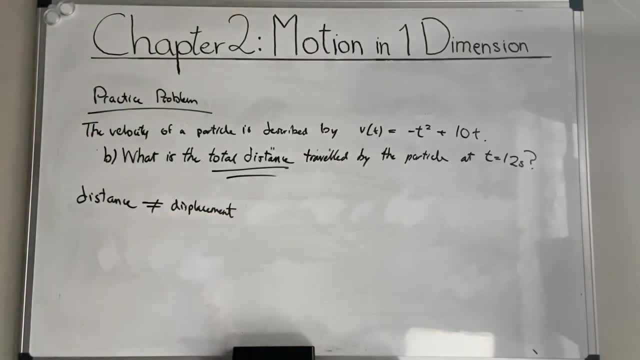 unless we can't use what we just used in the last question, we can't just find the integral. that would only give us the displacement um what we would need to do, for this situation is actually break down well I, I didn't mention this before, but it's worth. 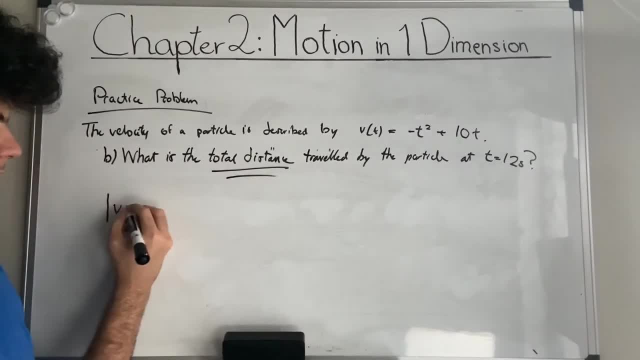 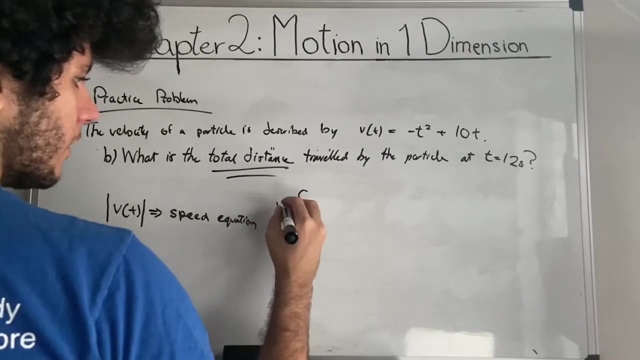 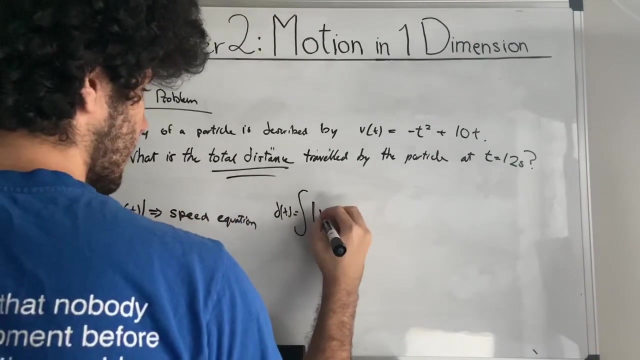 noting that the absolute value of the velocity equation is equal to speed, wasn't? this is the speed equation, and the integral of the speed equation that, my friends, is the total distance. so yeah, like this, just wanna make sure I don't make any mistakes for you guys. 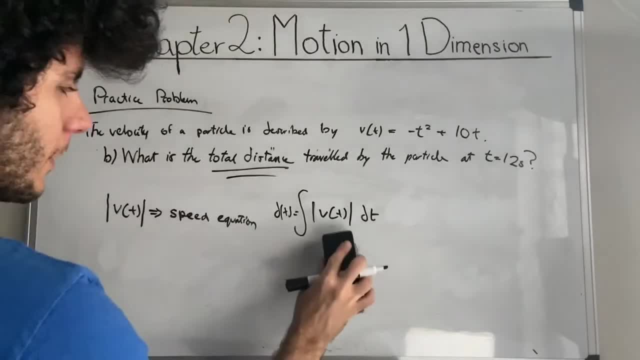 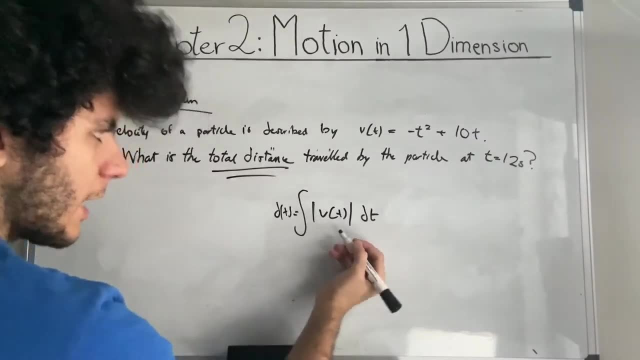 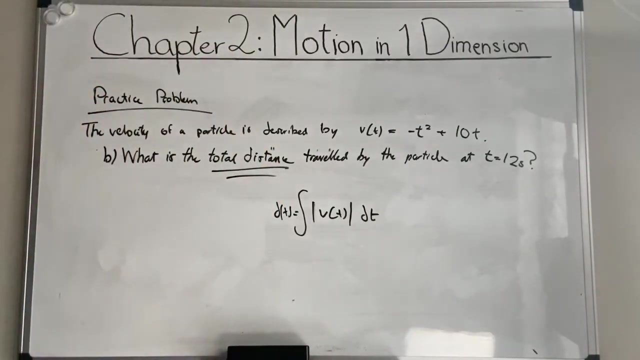 alright, this is what we're doing. however, it's not quite easy, right it? you might be like: what do I do? what is this? how do I take the integral of the absolute value? that's that seems unreasonable. well, maybe it sounds unreasonable, but that's because you have to think about. 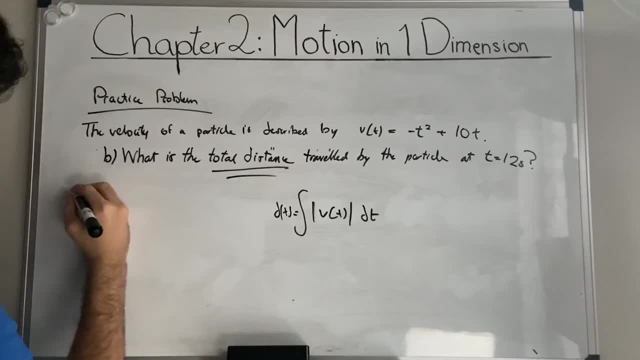 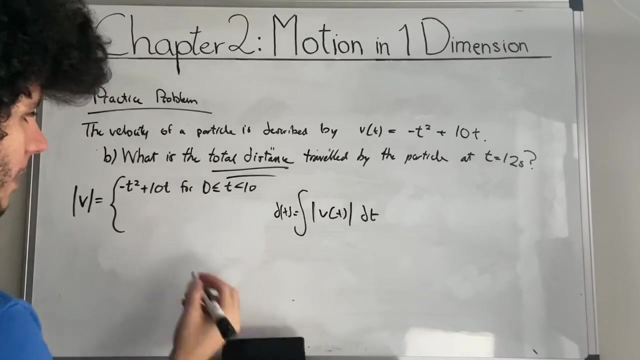 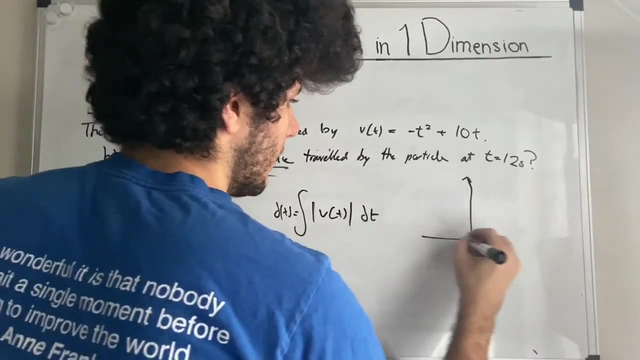 it in a different way. we have to decompose the absolute value of the speed equation, all right, so, so, So, okay, like this: negative plus 10T, 4, 0, through T small 10, right, So if, by finding okay, I guess maybe okay. so if we were to graph this, let's try it. 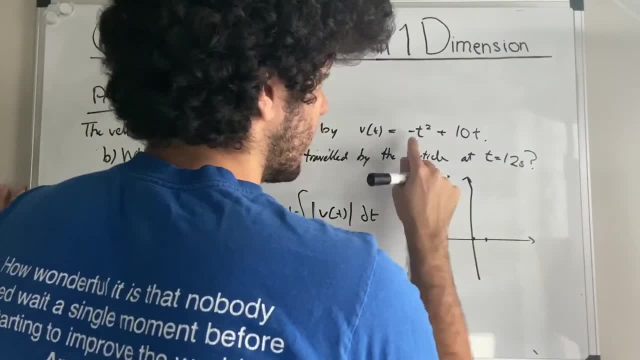 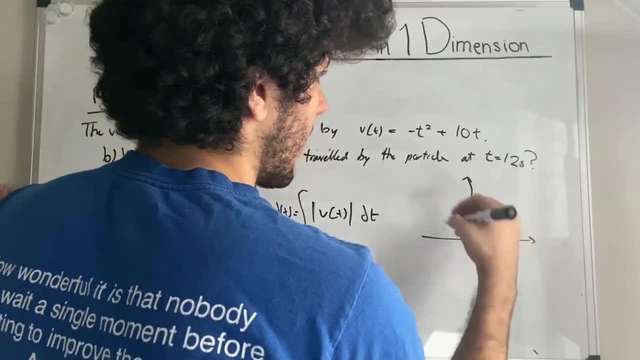 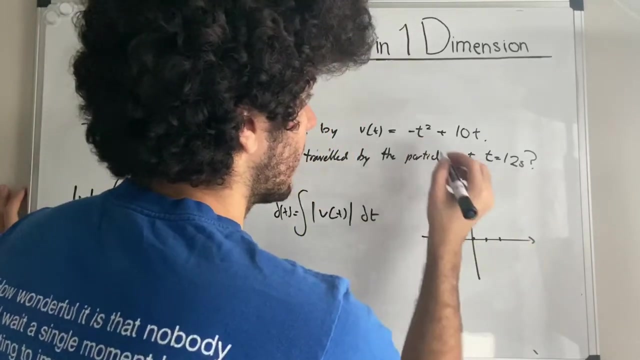 So 0,, it has a point. at 0,, 0,, at T is equal to 1,. we have negative 1,, 9,, that's 9.. And then at 2,, T is equal to 2,. so we have negative 4,, 20, negative 4 and 20 would give like 16.. 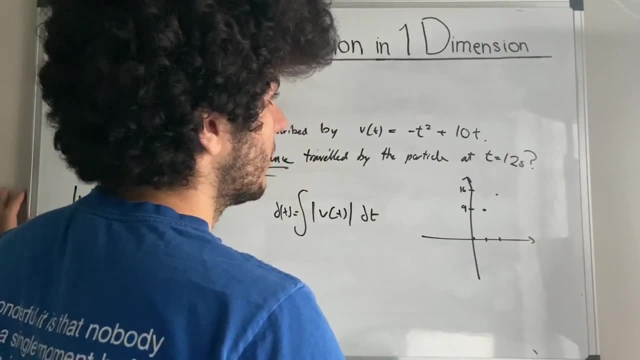 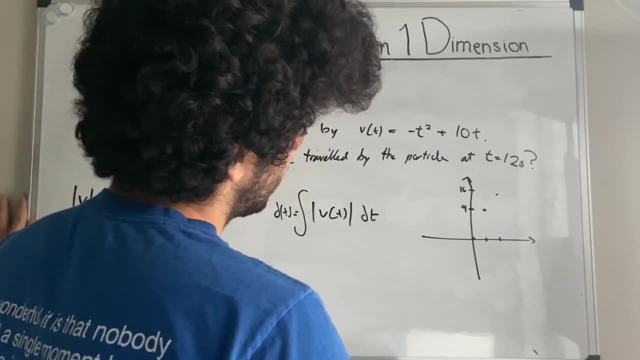 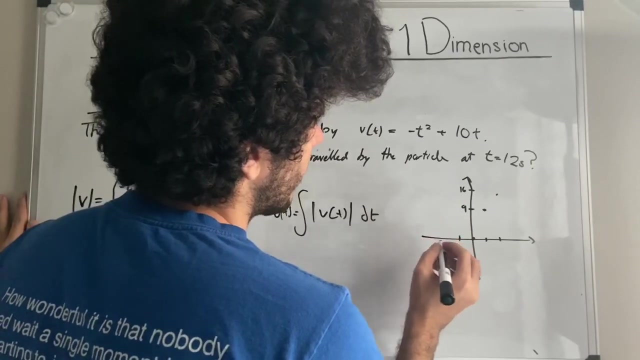 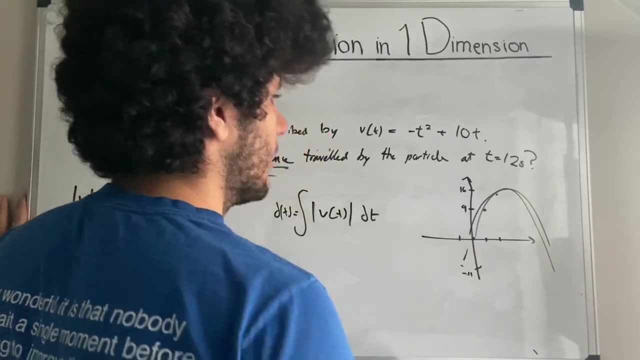 Let's see 5, 50,. huh, well, at some point let's see negative 1,. hmm, At negative, if we input negative 1, we would actually get negative 11,. interesting, I'm guessing the function looks a little bit like that. 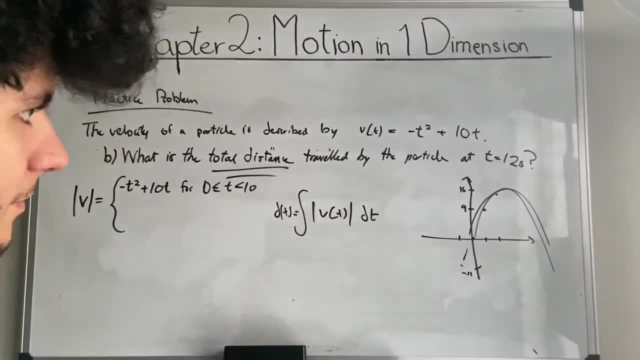 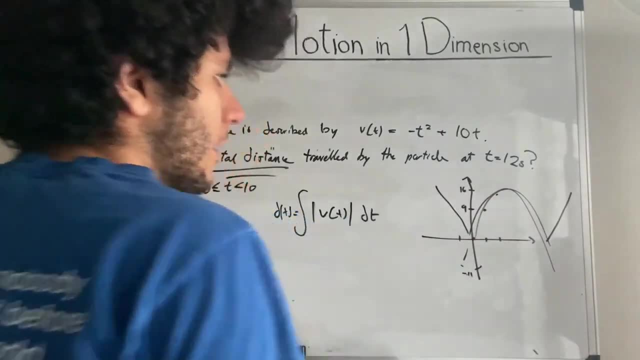 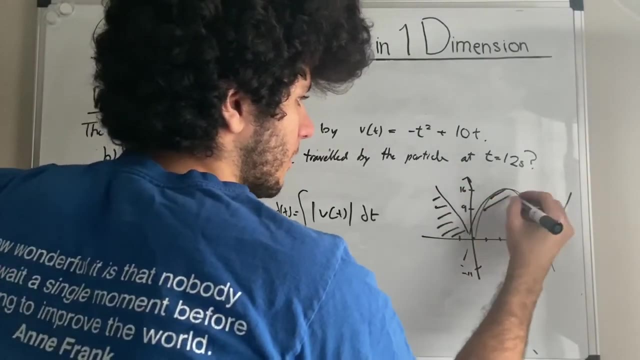 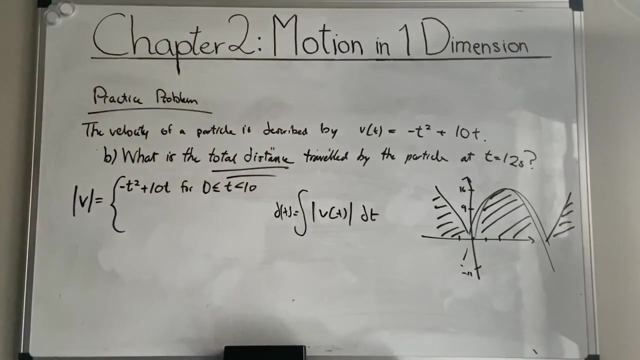 Does it The fuck. But anyways, we want only the positive values. So that's what's, that's what's, that's what it's going to look like. We want the integral only when the, the, the function is above um. y is equal to 0, or, in this case, v is equal to 0.. 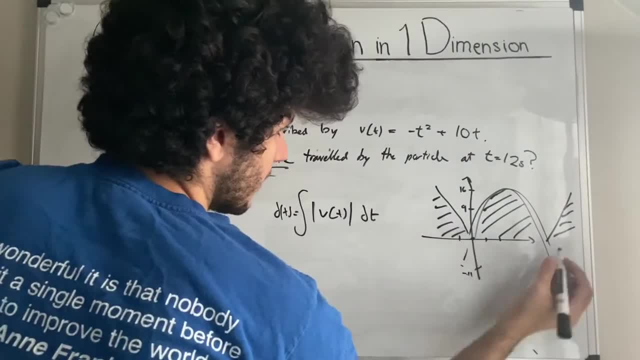 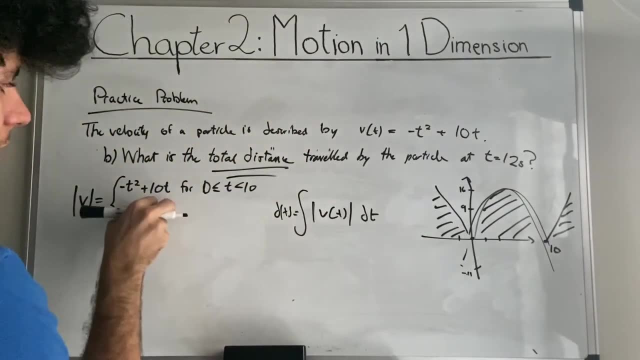 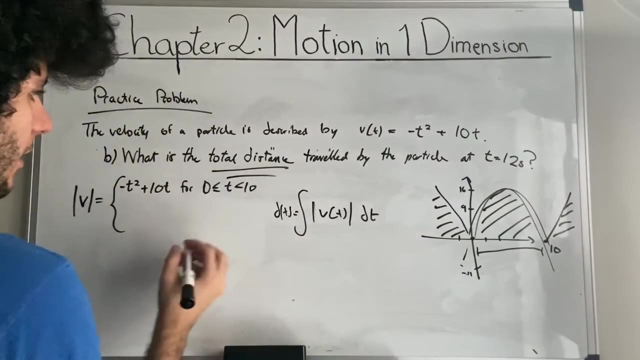 So that's what we're doing. We're finding this point and this point, which is 10, right. That's why I wrote that here. We're saying the function can remain as is between these two values. However, when it's smaller or larger or actually not, we're not going to consider smaller than 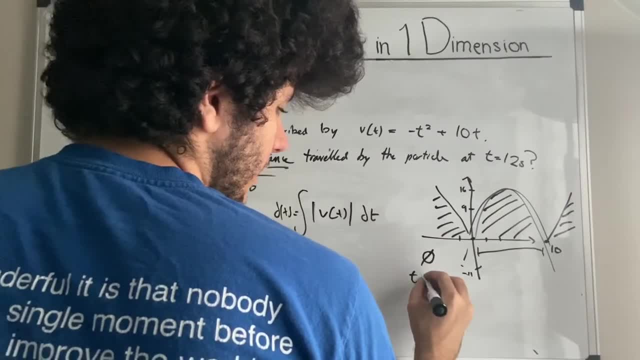 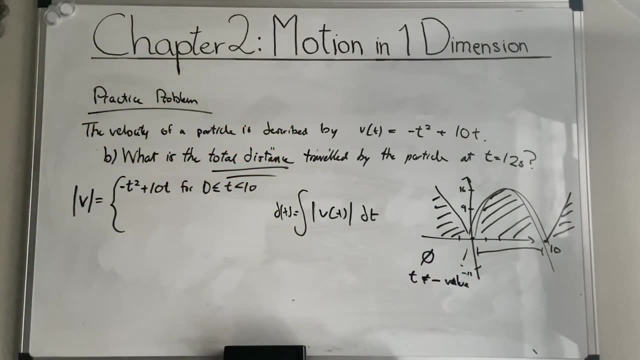 This is irrelevant to us, because t cannot be equal to a negative value, right, So time can't be negative. Therefore, we're only going to treat, we're only going to take, we're only going to consider these values and further on. 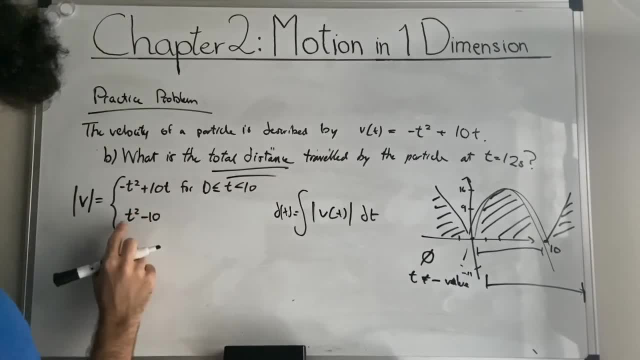 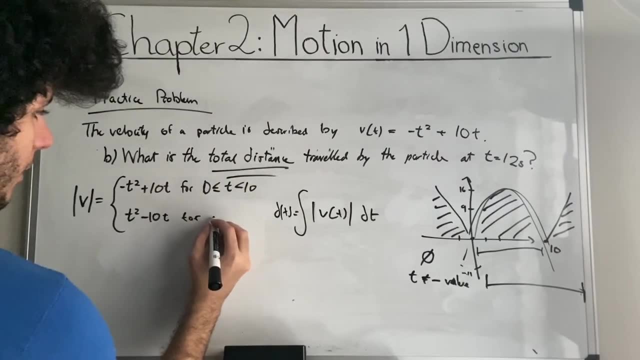 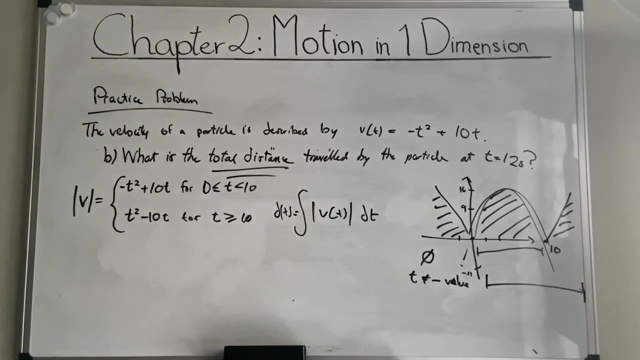 So here we do this. Here we do this. We multiply the equation times negative, uh, times negative 1, for t is larger or equal to 10. That should be correct. And small, oh, and it's until 12.. 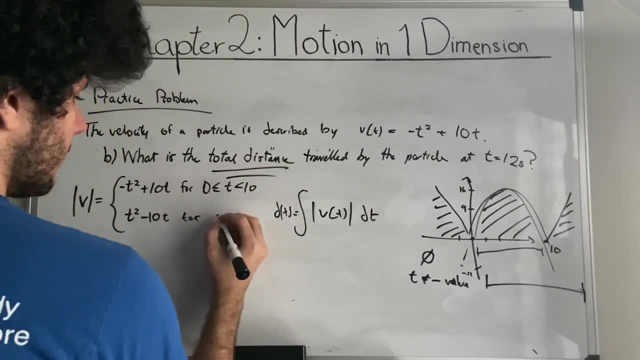 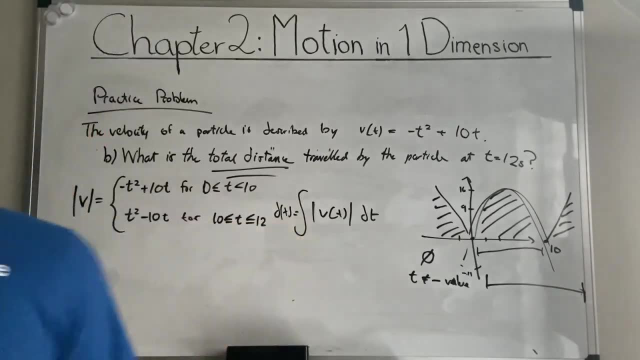 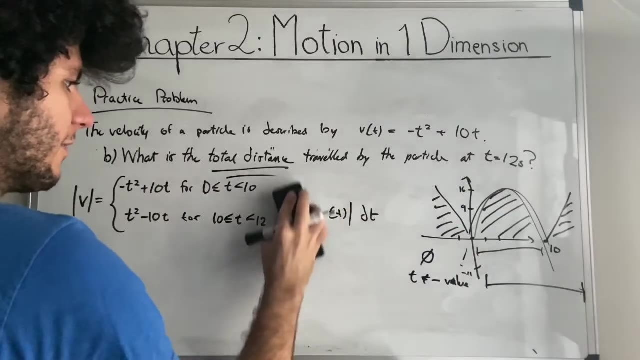 That's another boundary worth noting. So it's from 10 smaller or equal to t, um smaller equal to 10.. And this should be equal to 12.. Alright, Actually, smaller than So. basically, we have this now. 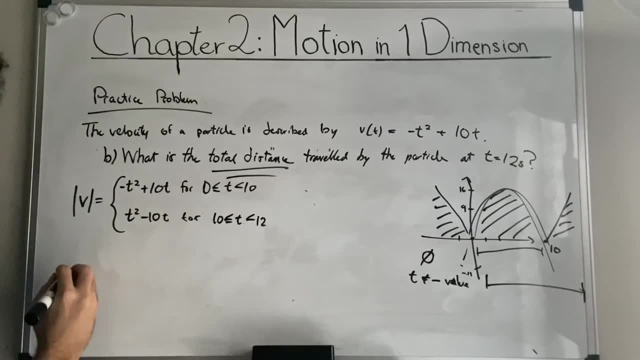 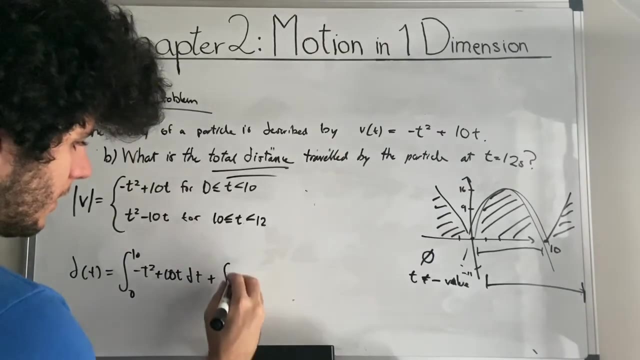 And trying to take the integral of this is quite simple actually. We just do this: You break it down: 0 through 10 of negative 2, plus 10t dt plus 10 through 12 of t squared minus 10t. 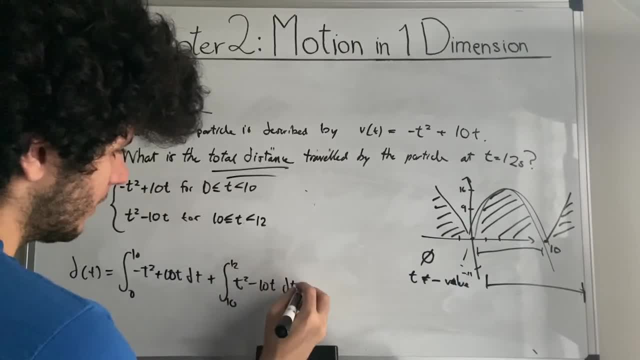 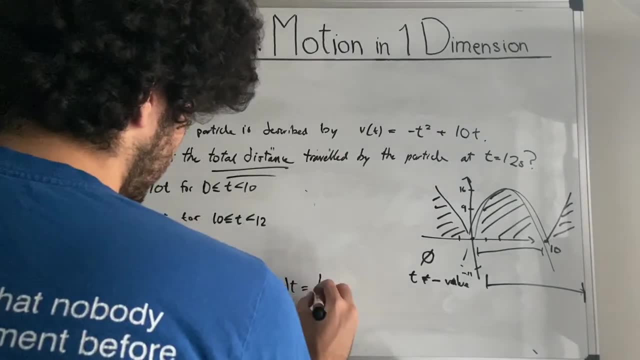 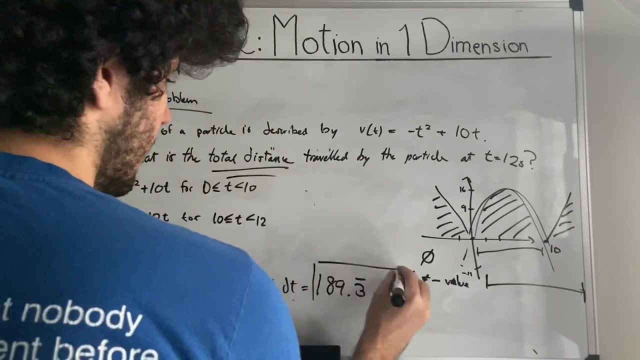 minus 10T dt, And after calculating this, I won't go through that trouble right now- You'll find out that the answer is 89.3 periodic, And this is in meters. This is the total distance covered in that time. 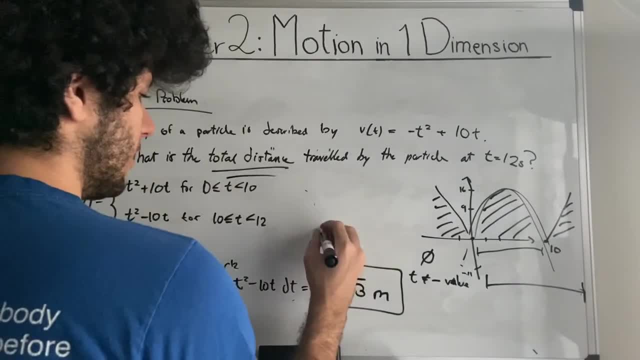 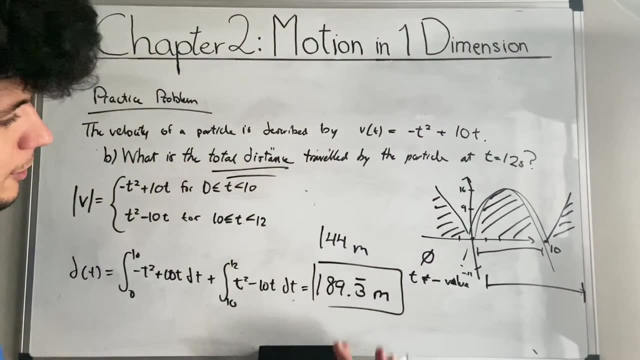 And so if we compare the two- the last, the answer of A to the answer of B, we'll notice that T was actually larger, which makes sense. It'll always be larger or equal to the displacement, as it can't be, there can't be any subtractions. 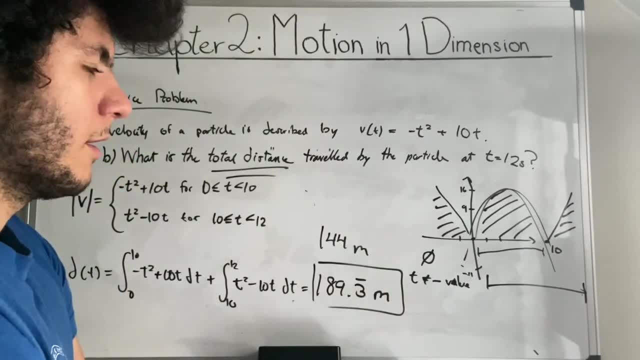 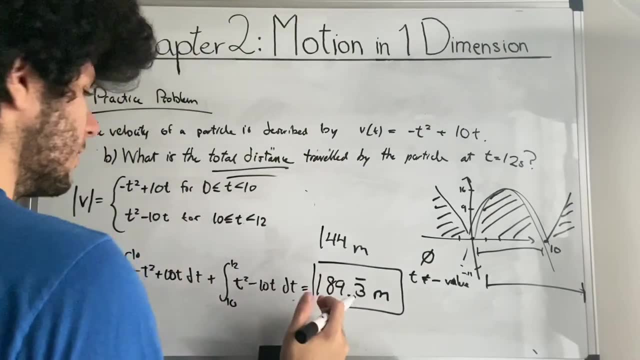 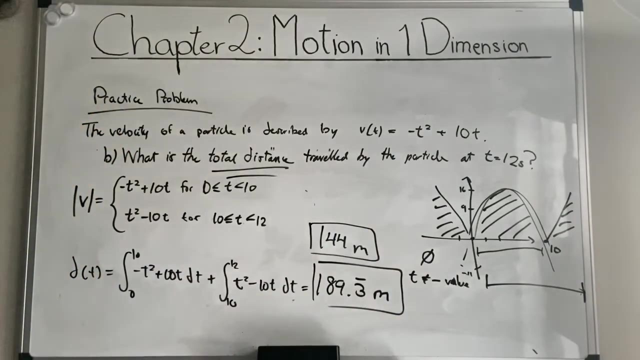 in calculating this, It's always going to be an addition of a length. Either you stop or you continue going, And if you continue going you're gonna increase the distance traveled. However, the distance, the displacement, can be negative, So you can't subtract values to it. 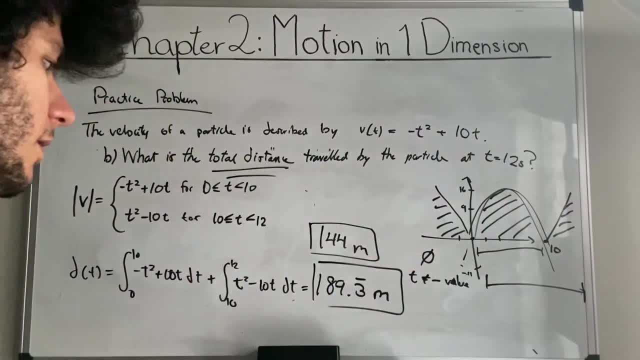 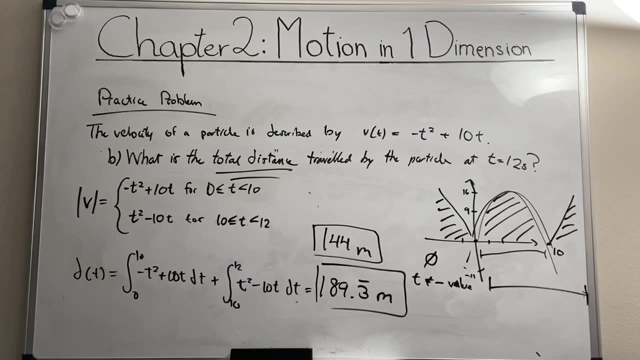 If you go in one direction and they start going in the opposite direction, then you're gonna subtract your displacement. All right, thanks so much for watching guys. Next video we're gonna go over the kinematic equations of chapter two. So see you guys there.